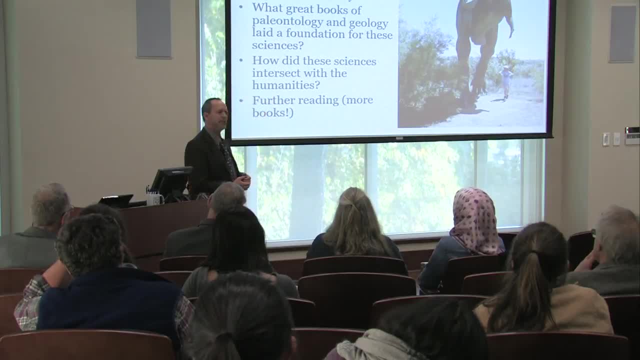 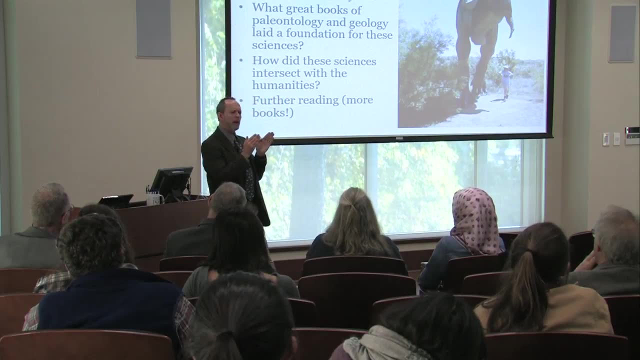 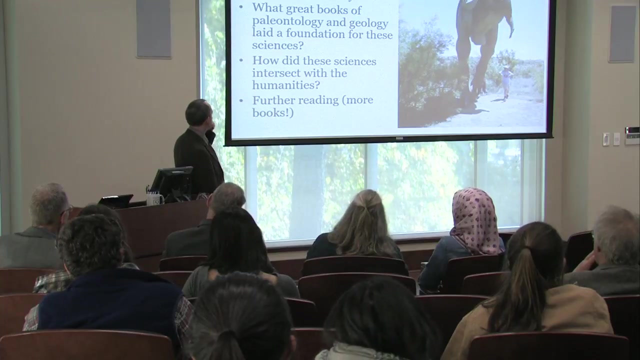 That's yet another question- Dinosaurs and some of their contemporary animals. And then, third, we are going to look at the great books of paleontology. And when I say the great books of paleontology, I'm talking right at the very beginning of the discipline, right around the early to mid-19th century. And then how did that lead to the booming science of paleontology we have today? That's an international science practiced by people in more than 100 countries. Now, how did these sciences intersect with the humanities? Oh, that's a curveball you didn't expect. 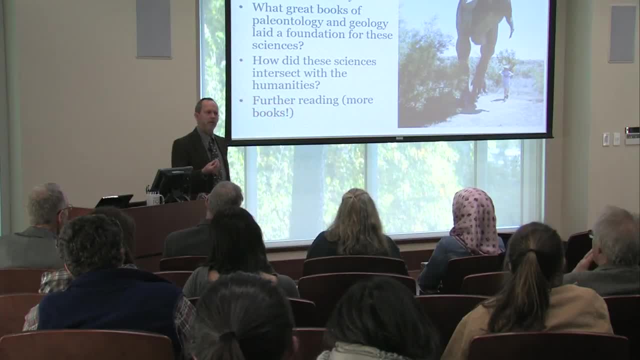 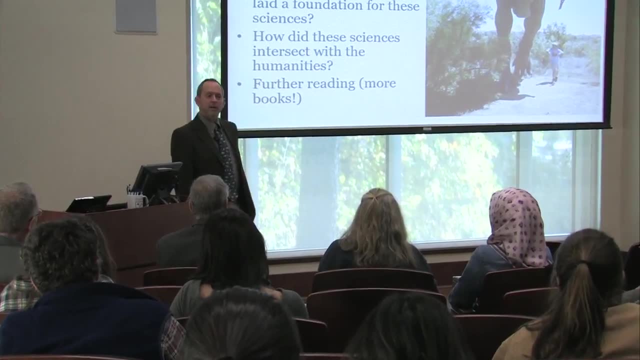 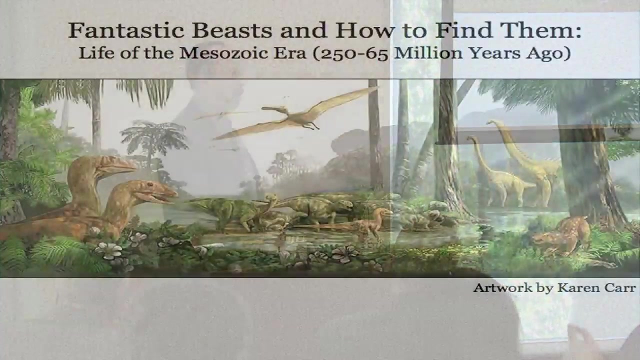 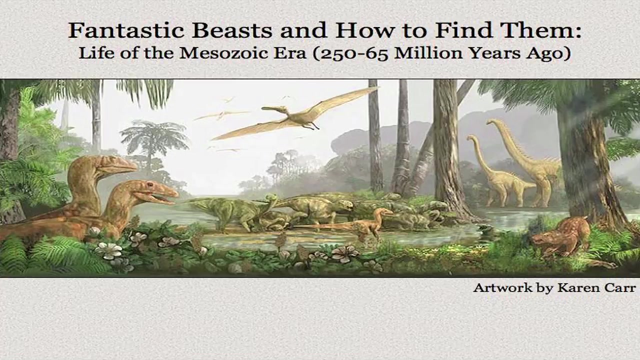 Did you, But they do, And paleontology is a particularly excellent science for connecting with the humanities, social sciences and other disciplines. Then at the end, I'm going to give you homework- but there's going to be no grades on it- Some more books that you can read that are about paleontology. So fantastic beasts. How do we find them? If you go back to the Mesozoic, if you have a time machine, you go back to the Mesozoic era from, say, 250 to 65 million years ago. these 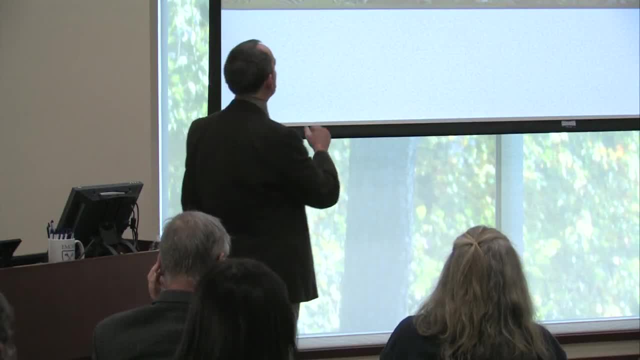 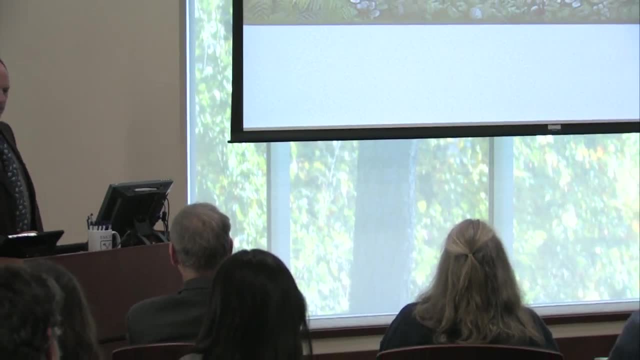 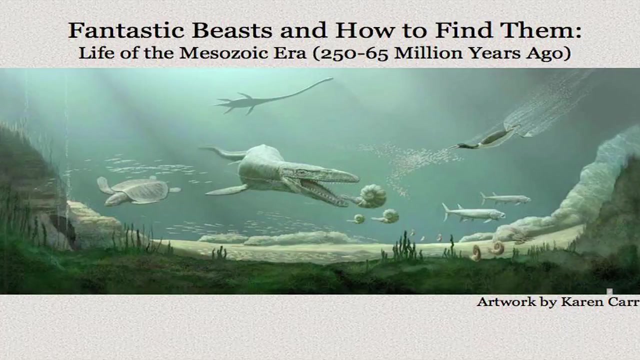 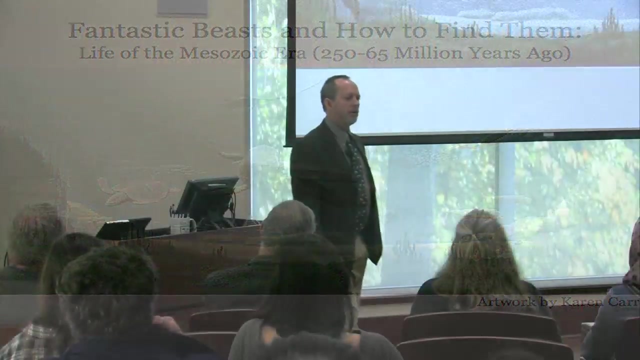 are some of the animals you would see. These are some of the plants you would see. It would be this fantastic world with these beasts that some of them may be familiar but most of them are extinct. If you go into the ocean for a swim, you're in for a surprise, because there are going to be some very large animals out there that if you were afraid of sharks, you're going to be even more afraid of these: Mosasaurs, plesiosaurs, but also a few familiar animals that you see still around today, such as sea turtles. 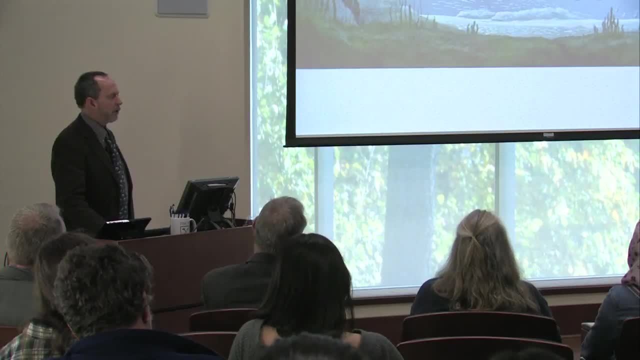 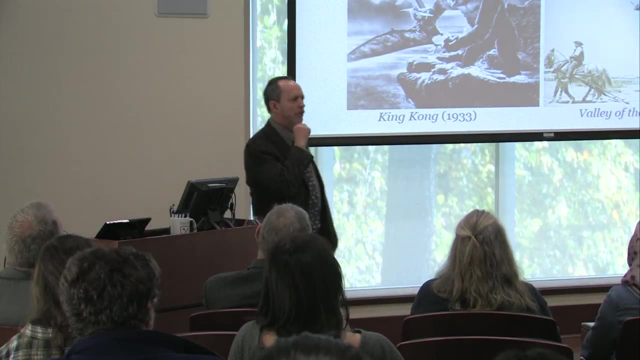 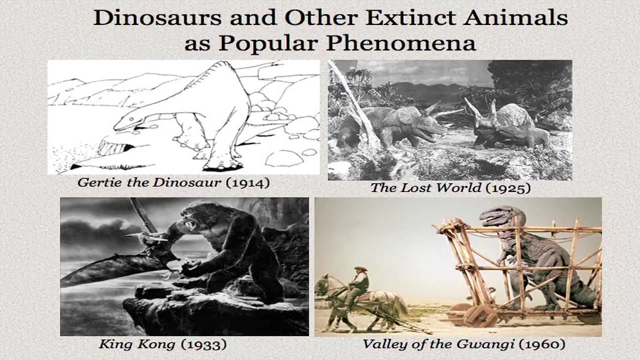 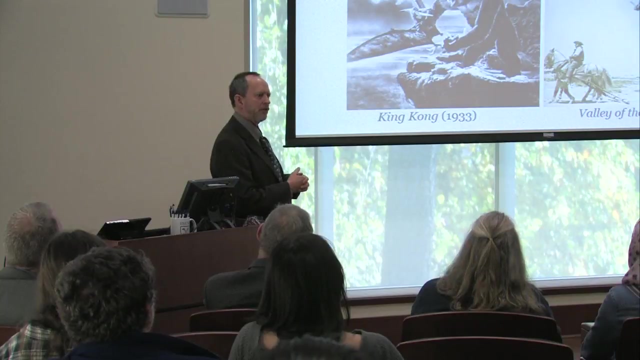 sharks and other types of animals like that. So in the oceans and on the land were these different animals that, when we think about it in terms of how does that connect to today? there's pop culture And pop culture has definitely been tapping into our fascination with these extinct animals of the past, Going back to the first animated film that featured a dinosaur, Gertie the Dinosaur. to Lost World, a silent film in 1925,. 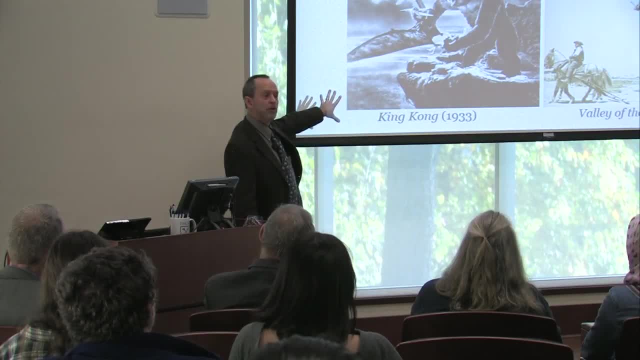 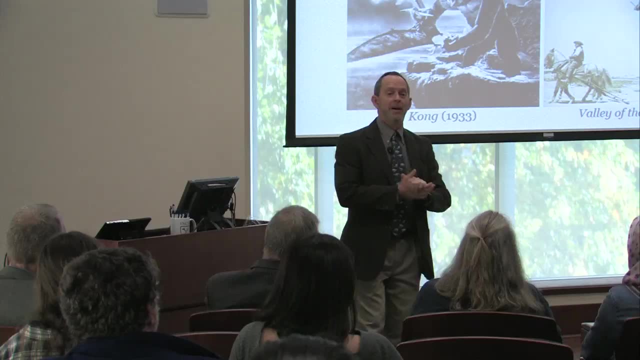 the original King Kong. not all the remakes, but the original King Kong featured dinosaurs and a pterosaur- a flying reptile there, and one of my favorites when I was growing up as a kid Valley of the Gwangi. What a great movie. Cowboys and dinosaurs- it doesn't get any better than that. 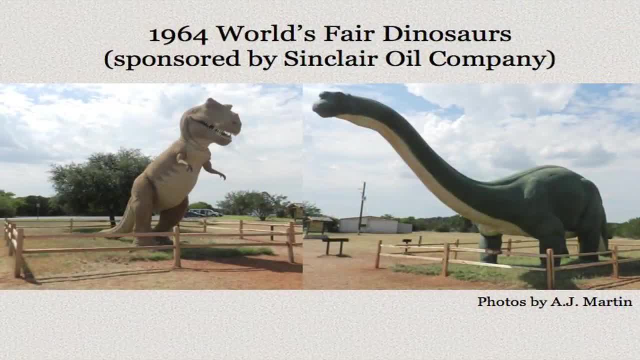 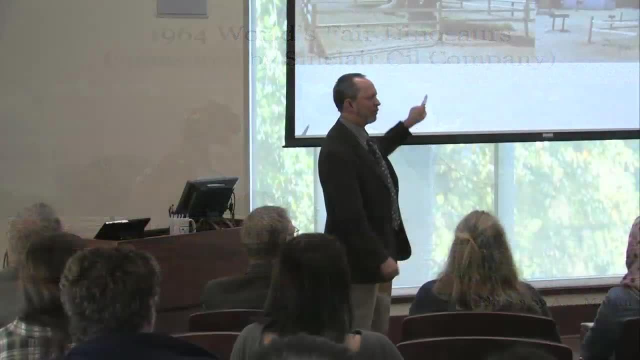 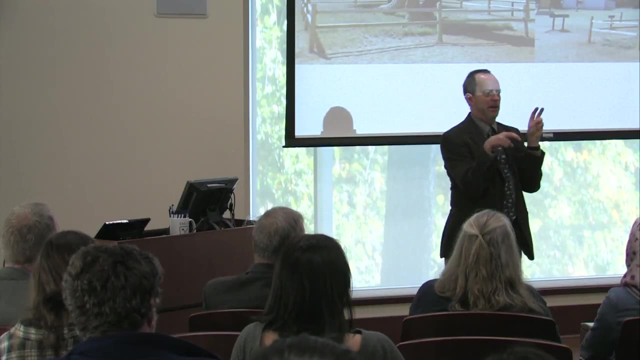 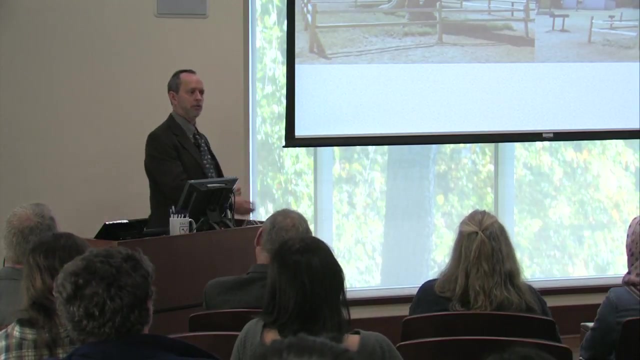 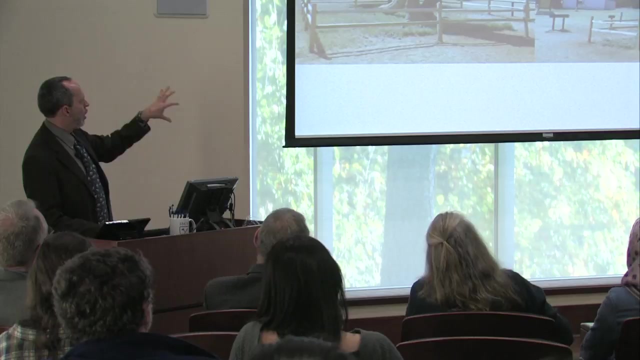 All right, but 1964, Sinclair Oil Company sponsored these dinosaurs to be made life-sized dinosaurs. Everybody can name the one on the left right. On the left is Tyrannosaurus Rex- you can tell by the arms right- And then on the right Brontosaurus. Yeah, and actually the name Brontosaurus was obliterated for a while, but it just made a comeback and we can again use the name Brontosaurus for these long-necked big sauropods. 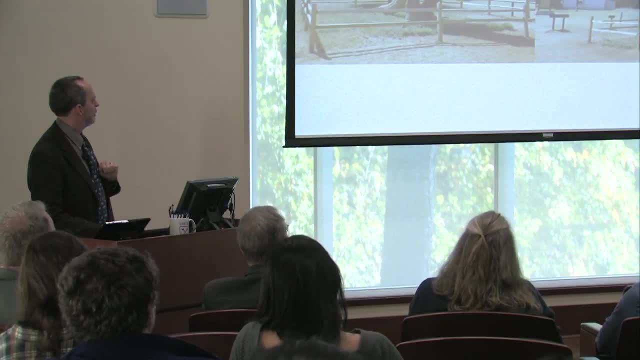 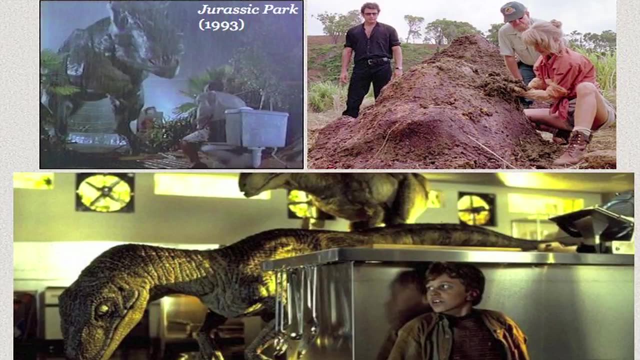 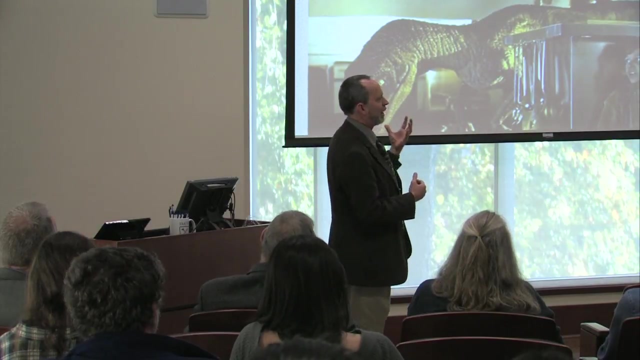 You can see these in Glen Rose, Texas. They're right there, just outside of town. But of course, we have to always go back to the documentary film Jurassic Park- right, Because that is the classic dinosaur film. Still, it holds up as the classic dinosaur film, where we think about dinosaurs as being some form of entertainment, but also these fearsome, awesome beasts. 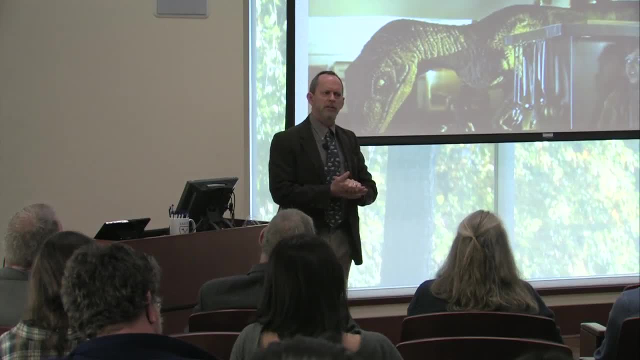 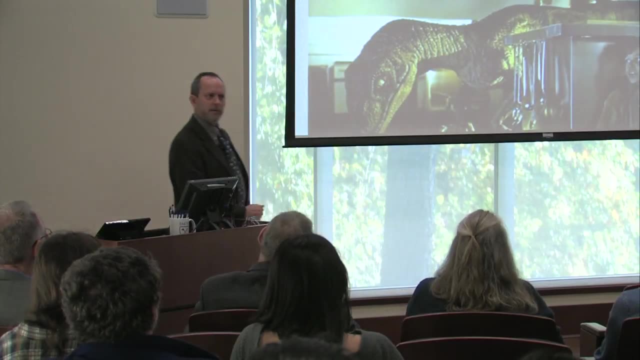 And up there on the left, that is a still from the greatest scene in cinematic history, when the Tyrannosaurus Rex, the true hero of the film, ate a lawyer off a toilet. I see none of you are disagreeing with me. Okay, good. 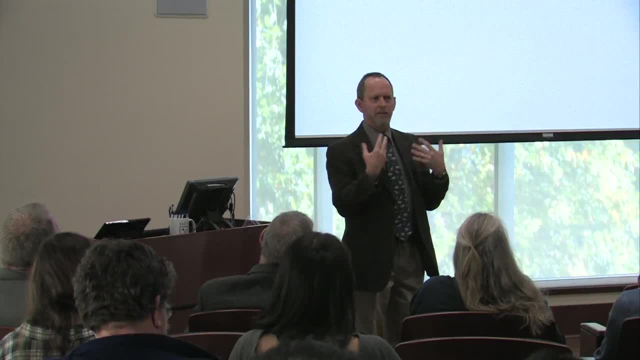 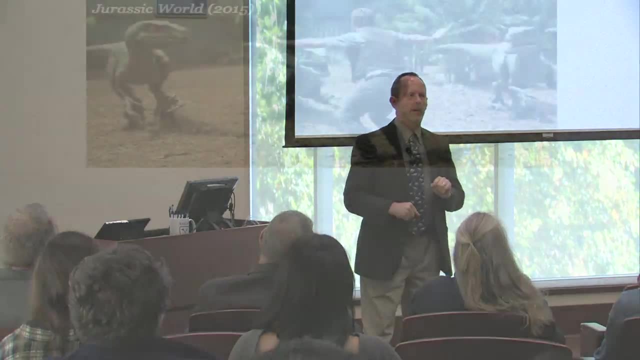 Then it took a big step back With this movie. I'm not even going to say what the title was, but it happened a couple of years ago. It is most famous for this scene where Chris Pratt's character did what's now been dubbed Pratt-keeping. 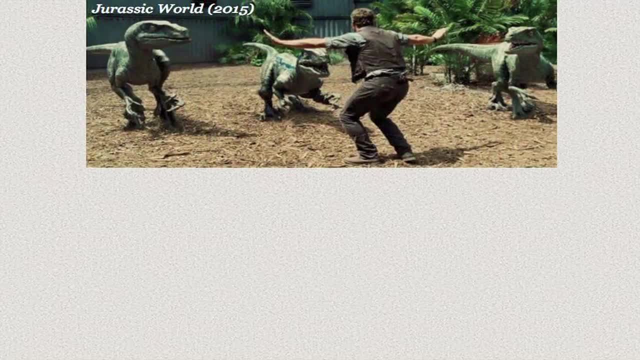 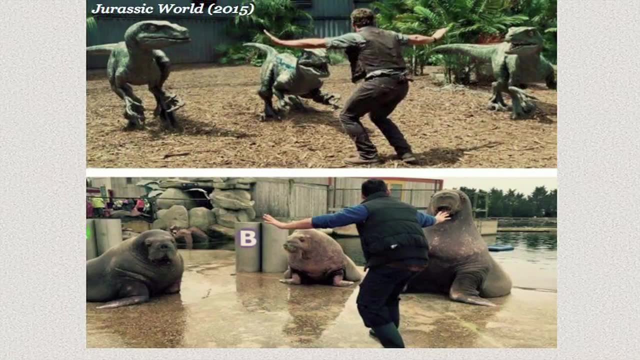 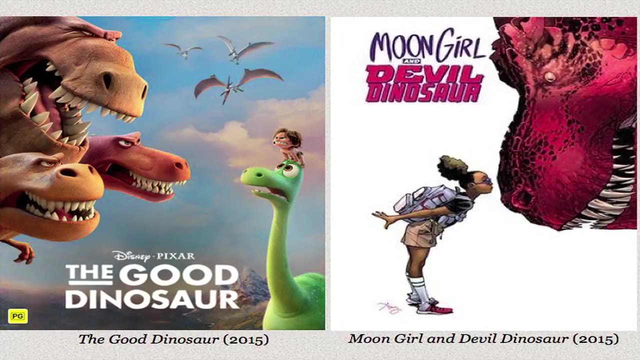 You remember that Pratt-keeping And what came out of it was a meme in which zookeepers all over the world imitated him. That was the redeeming quality of that film. All right, so going to. just recently, We also have animated films still featuring dinosaurs and Marvel comic books. 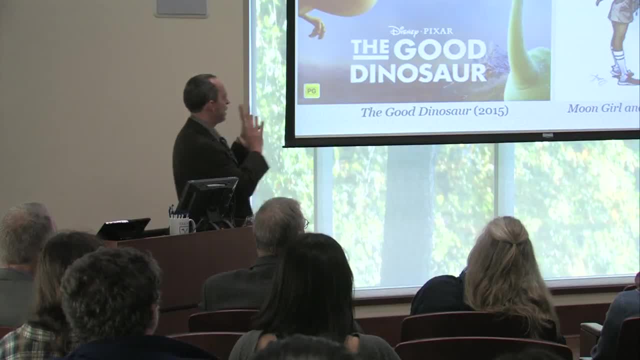 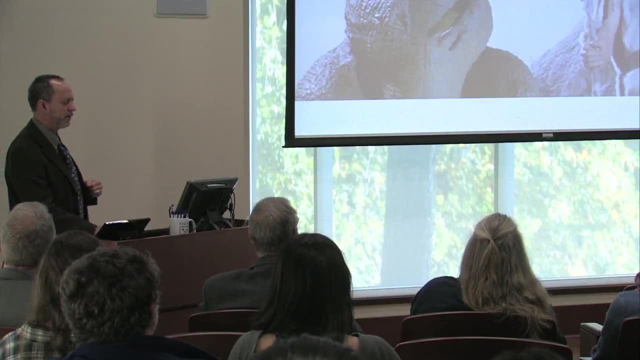 Why is this not a movie? Oh my gosh, this needs to be a movie. Moon Girl and Devil Dinosaur. So dinosaurs are still hot. They've always been hot since we knew they existed. But when did we start getting fascinated with them? 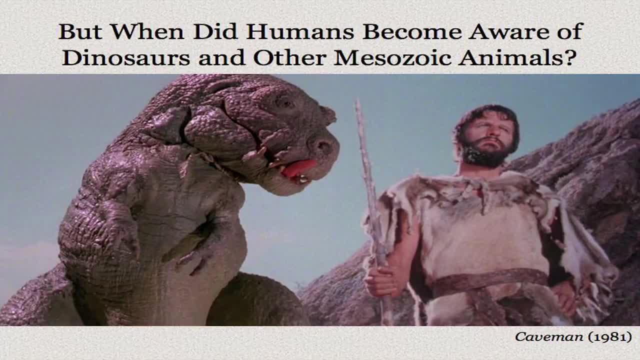 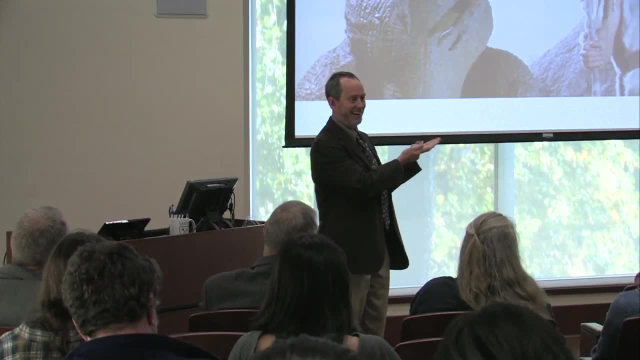 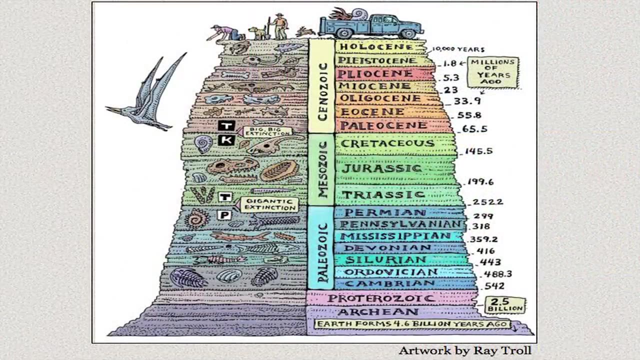 When did we start thinking about dinosaurs and other animals of the ancient past? When did that happen? What you see here never happened, because we have been separated from dinosaurs for about 65 million years Now. I'll make an exception of that later on when I talk about birds, because birds are modern dinosaurs. 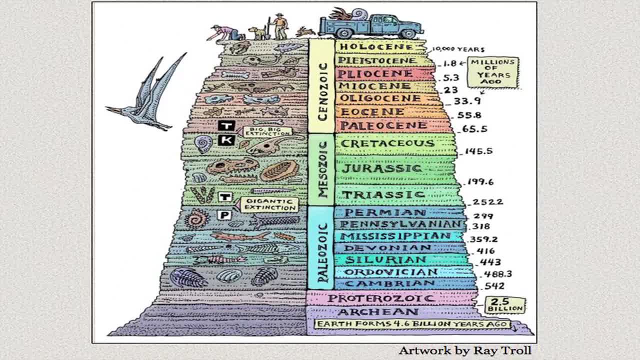 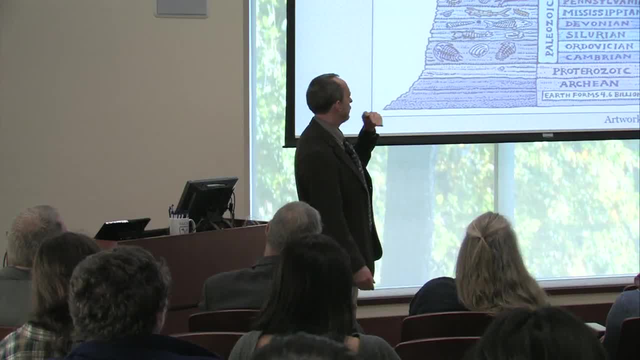 But if you look at the geologic time scale, you look at the Triassic, Jurassic and Cretaceous periods. that's when dinosaurs and a lot of their contemporaries lived. And then there was a mass extinction when a meteorite hit about 65 million years ago. 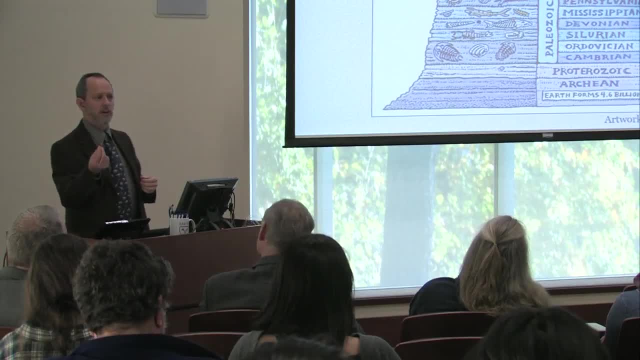 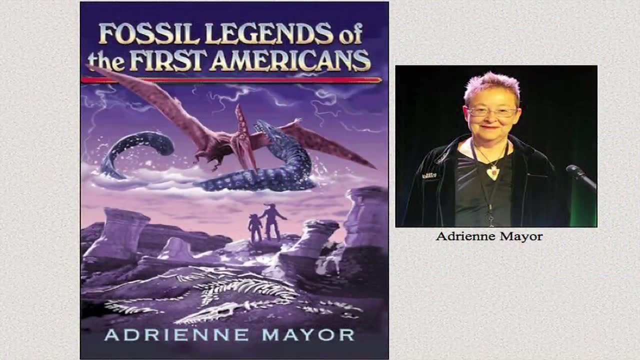 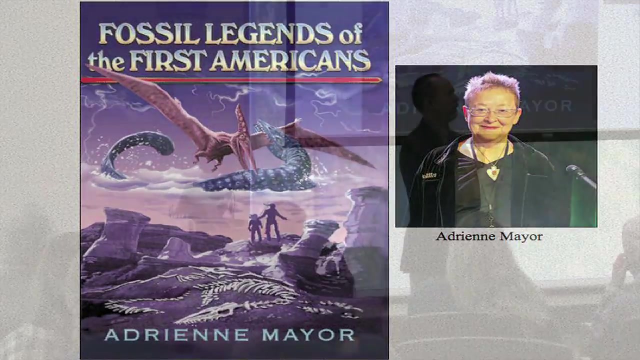 We are, then, at this slice in time: 65 million years later, We have been separated from those animals. Well, what's really interesting is to think about how indigenous people recognized some of the traces, some of the bones of these dinosaurs, recognized them as living animals. 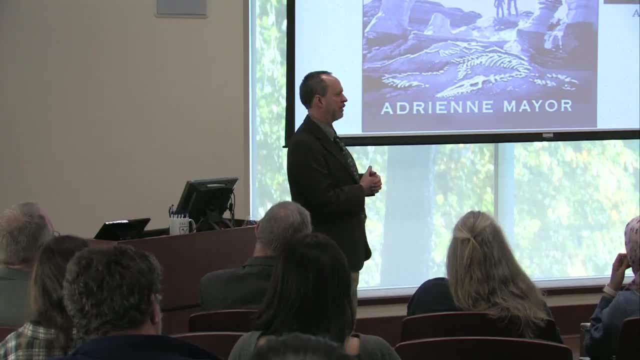 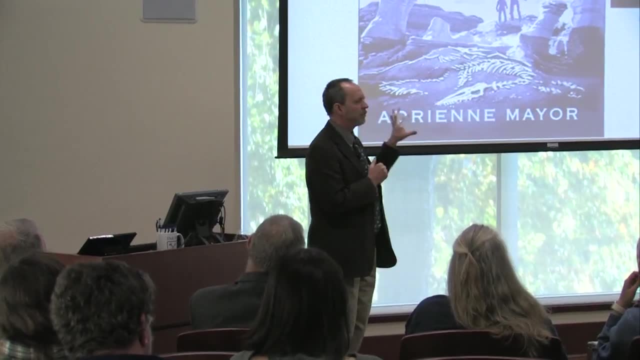 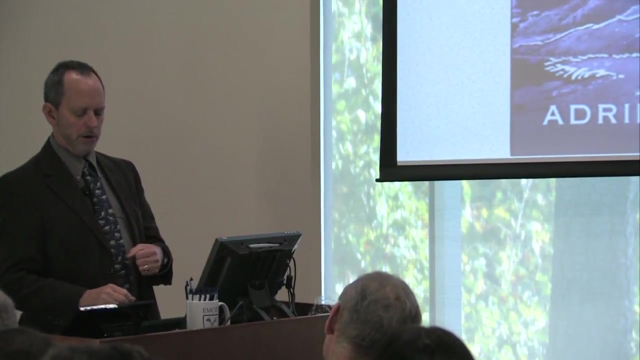 and recognized these vestiges as belonging to living animals. This is a book I'd recommend reading by a scholar, Adrienne Mayer, where she documented how many of the native animals, the native American legends we have in North America, are actually connected to fossils that occur in those places. 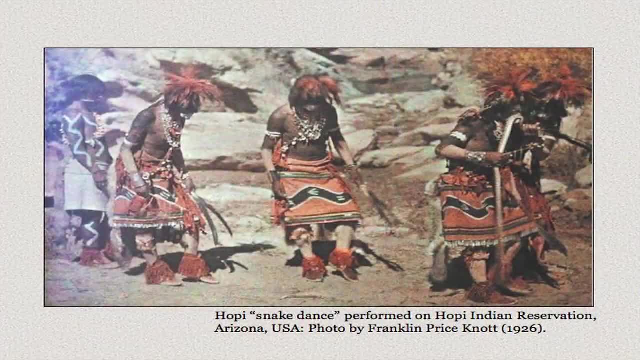 And one of the examples that I love to point out is this one about the Hopi of the southwestern United States, where, if you look at the snake dance that's being performed here, this is a photo from 1926, look at the icon there that's on the skirt there. 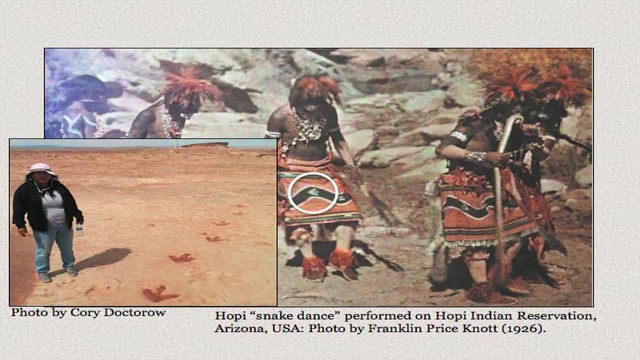 and that icon matches the morphology, the form of three toes. So these are the three-toed theropod carnivorous dinosaur tracks that are on Hopi reservation today. So we do think that a lot of native American tribes did connect with what was there in their area. 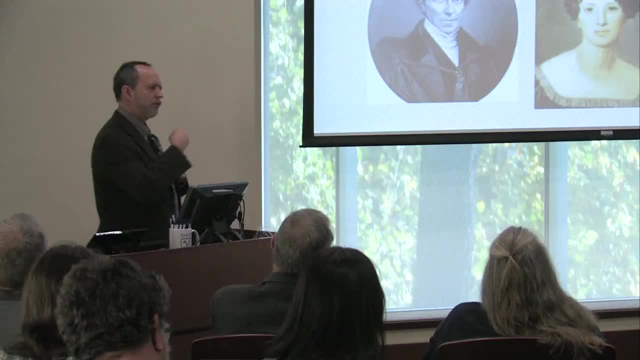 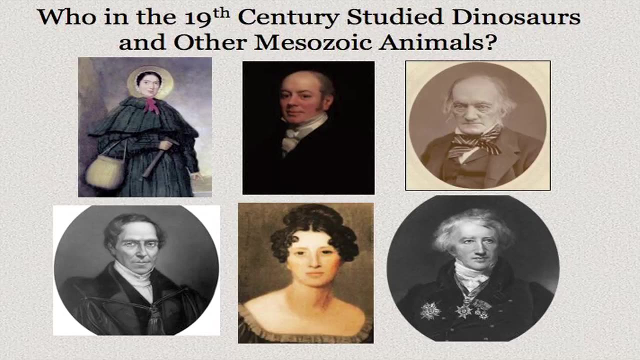 and then incorporated that as part of their heritage. Now, skipping ahead though, the more formal study is in the 19th century of paleontology, So indigenous people were aware of these, but the formal study in the western sense didn't really start until maybe late 18th century, early 19th century. 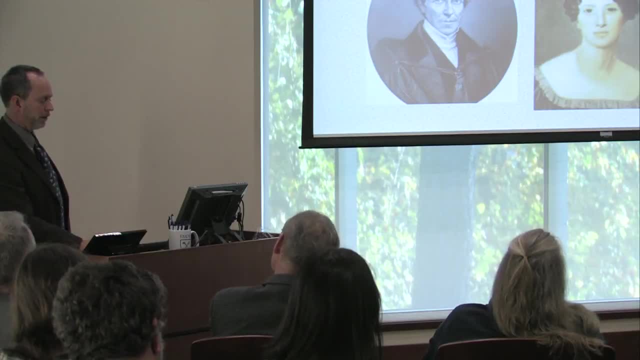 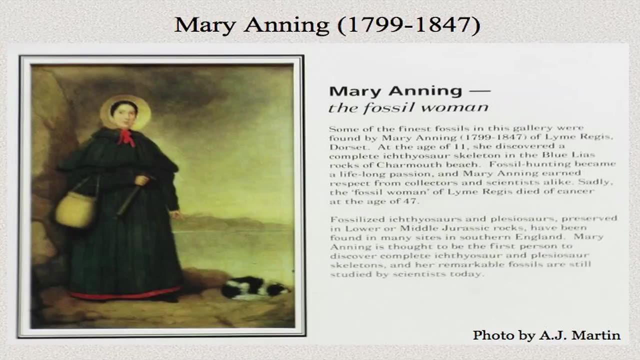 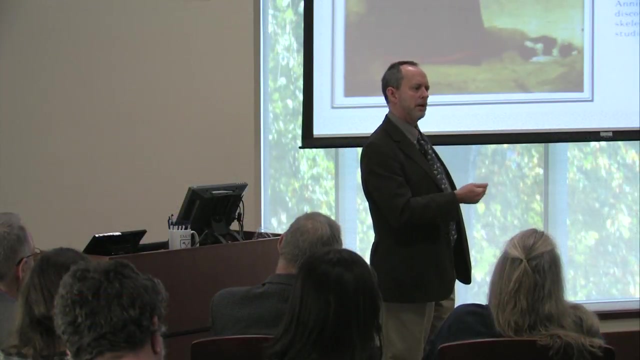 So I'm going to talk about each of these people here and how they contributed in their own unique ways. Mary Anning was probably the most important person for the beginnings of this paleontology because in the early 19th century she was near Lyme Regis in the southern part of the UK. 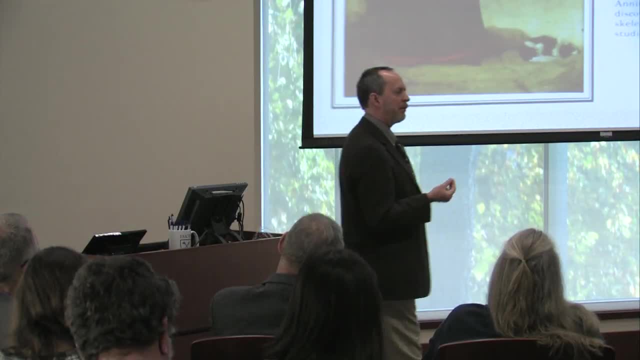 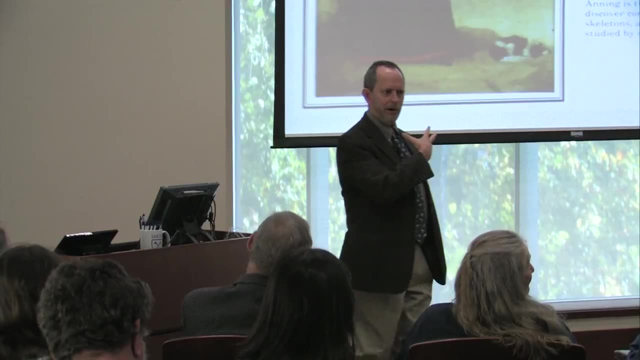 She and her father started collecting fossils. So how many of you have heard the tongue twister? She sells seashells by the seashore. This is supposedly credited to her, I've heard there's a little bit of doubt about that. 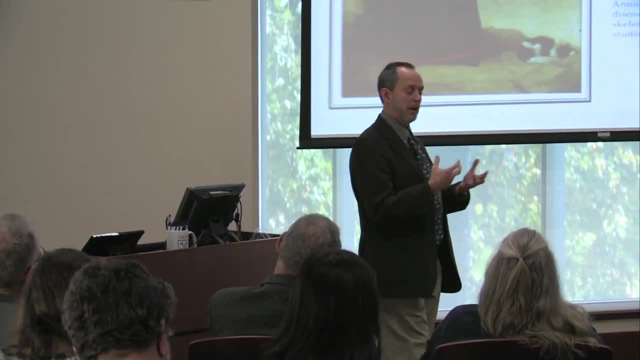 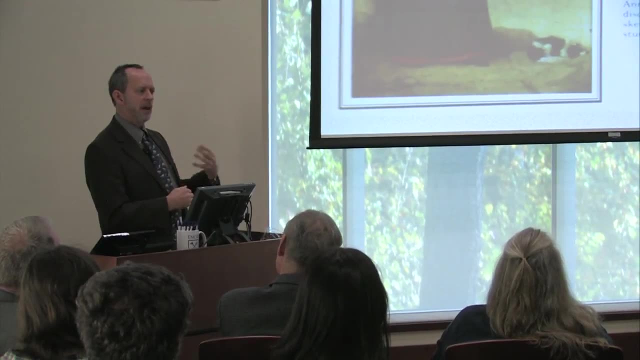 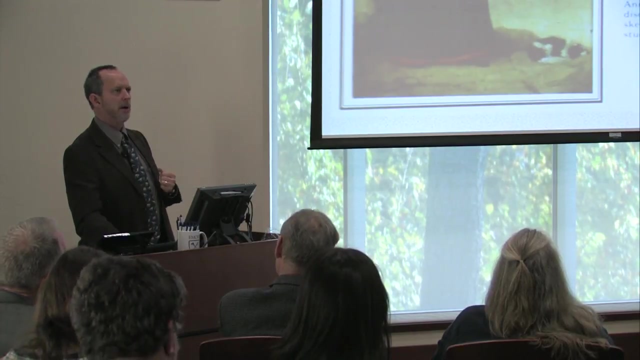 but it was about her in terms of her fossil collecting, where they collected fossils, sold them to the public and tried to make a living from that. Some of the discoveries she made of these animals, these fossil animals from the Lyme Regis cliffs, ended up being earth-shattering in terms of their science. 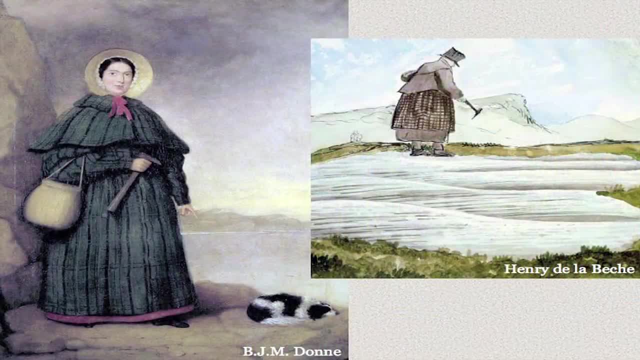 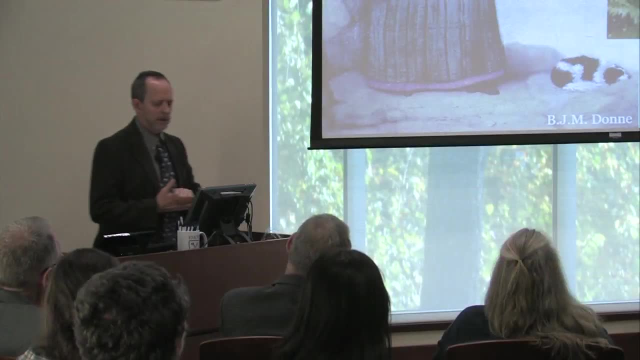 the science that came out of them. So some of the artwork depicting her at that time. she always has her trusty rock hammer with her and her faithful dog in this painting there. that was a companion with her when she went out and did field work. 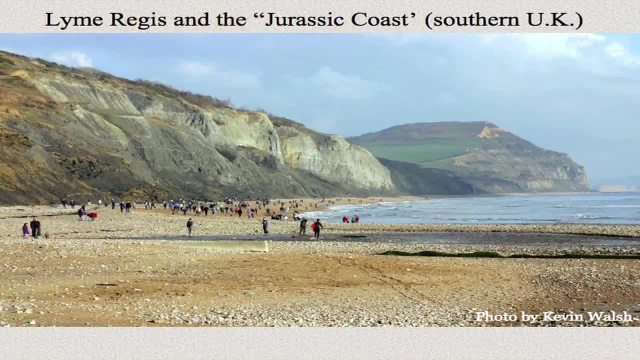 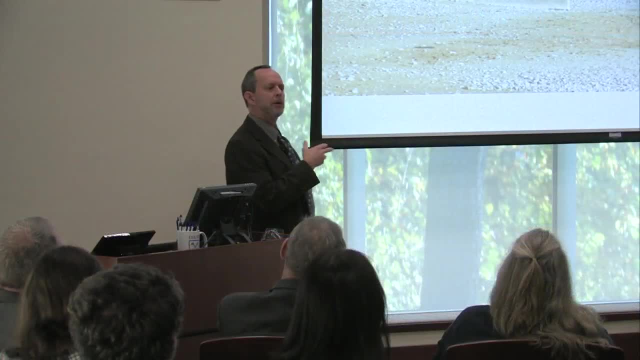 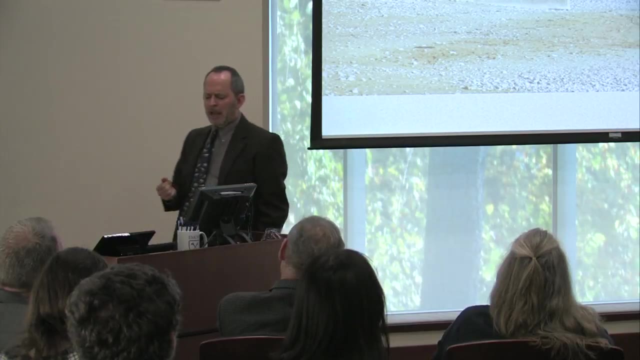 Now this area. unfortunately, I haven't visited this area. I have visited up by Scarborough. There are Jurassic cliffs there as well, But this is a world-famous locality for its Jurassic-age fossils- Fossils from about 200 to about 80 million years ago around in there. 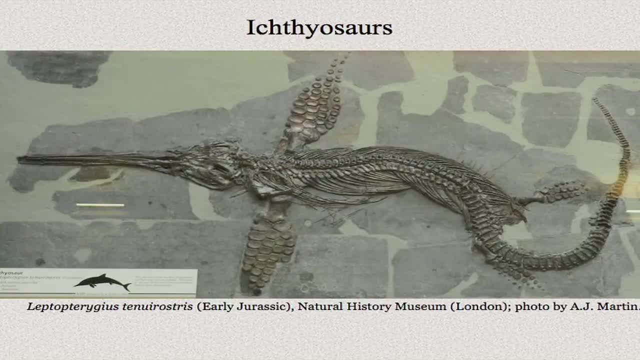 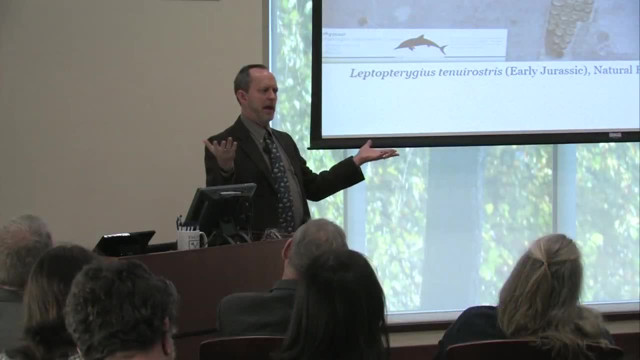 And this is one of the fossils. This is the first fossil she found. This is an ichthyosaur. So ichthyosaur literally means fish lizard, in that they recognized that it had these adaptations for swimming. So you see the big paddle-like fins. 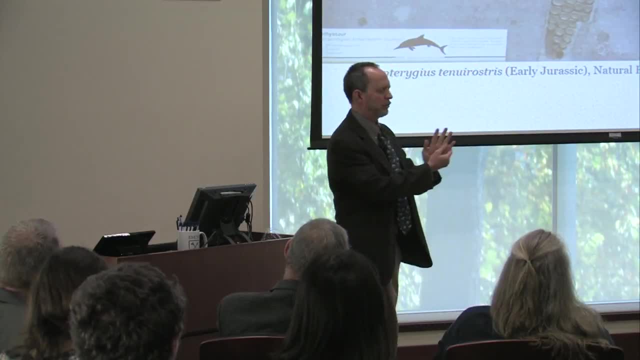 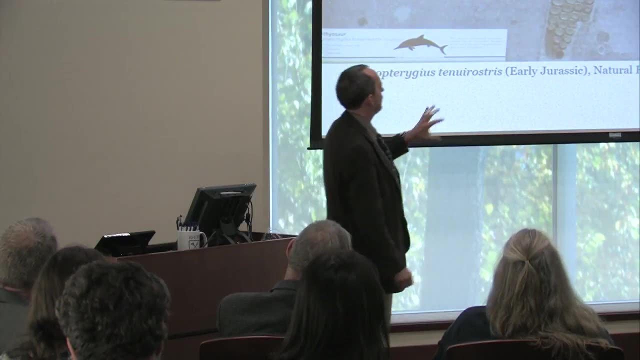 But if you count the digits, it's actually there's four digits there and there used to be a fifth one, a vestigial digit, there. So these are descended from land-dwelling animals that, in the Triassic period, then evolved into these fully marine reptiles. 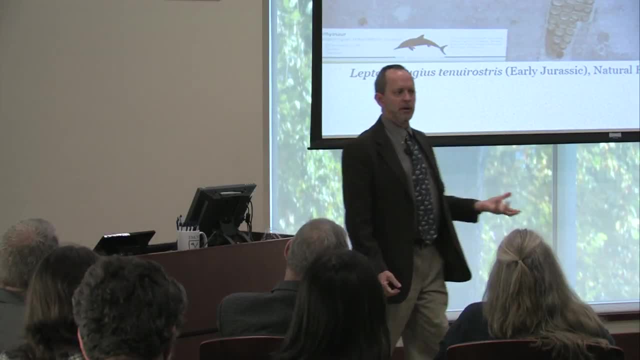 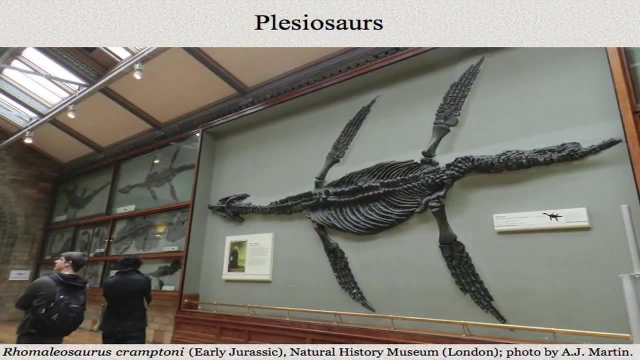 And we now have evidence that they gave live birth. These were some of the first marine reptiles we have evidence for giving live birth, So this was quite a discovery. with the ichthyosaurs, She also found plesiosaurs. Plesiosaurs were more of these long-necked ones. 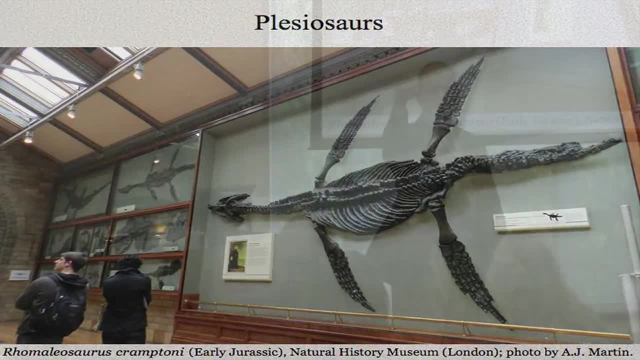 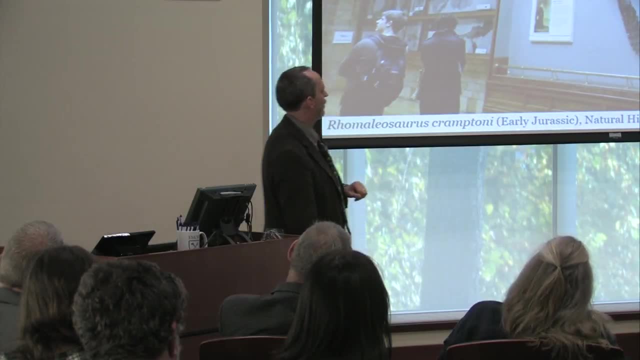 So you've heard of Loch Ness Monster, for instance. No Good, Okay, yes, a few of you Okay, which is totally fake, But a lot of people tried to credit the Loch Ness Monster to plesiosaurs. 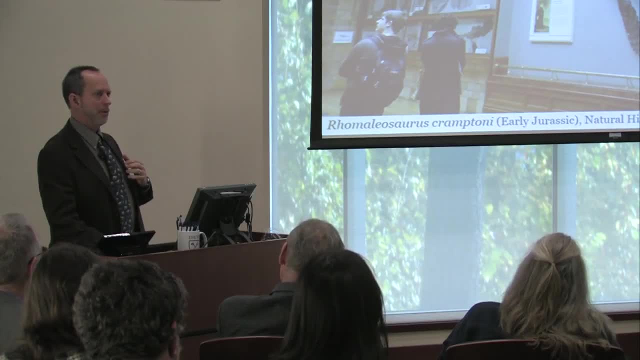 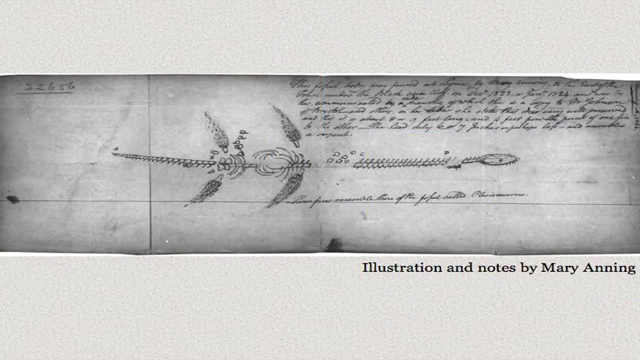 Plesiosaurs, though, were again these large marine reptiles. Some of them got huge, more than 20 meters long, and they roamed the seas eating fish. Mary Anning was also a skilled illustrator, So often when she took field notes with her discoveries. 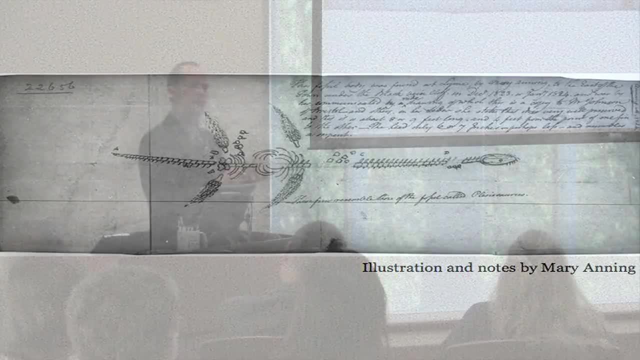 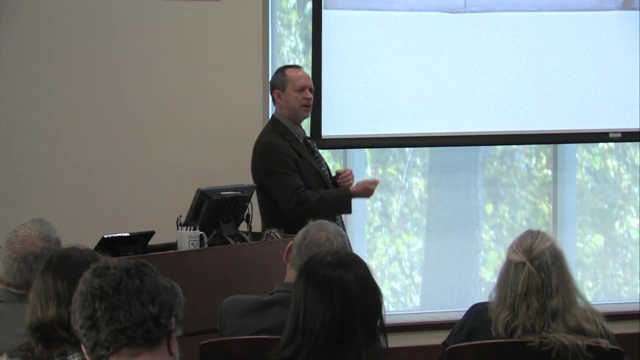 she also documented them by drawing, So you're going to see a lot of paleontological art throughout this talk. that's part of the humanities angle- is thinking about how this form of scientific documentation oftentimes was visual, that it did reveal. 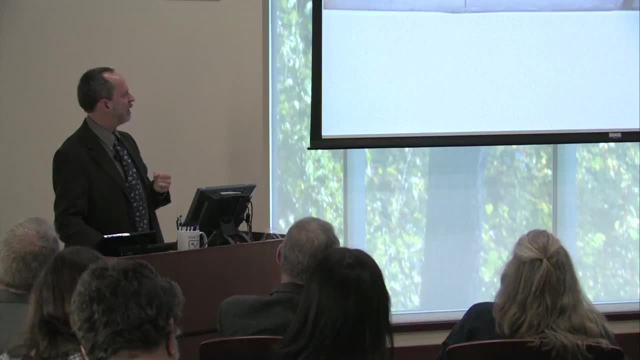 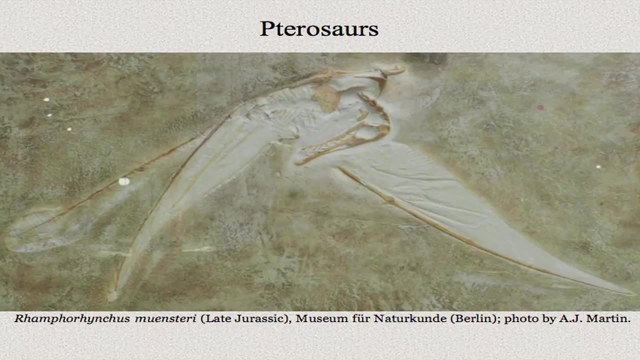 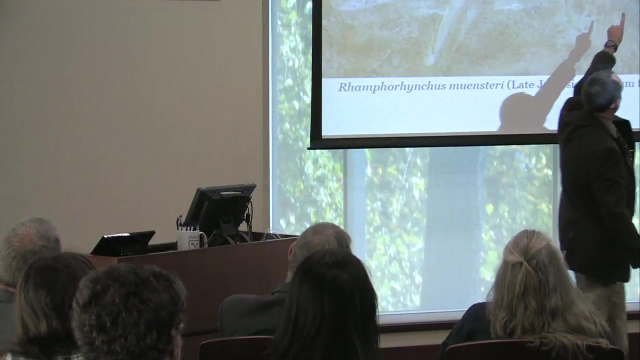 It did require a sort of graphic representation to be able to communicate the science properly. Now, pterosaurs are among my favorite animals from this time, because pterosaurs were the first vertebrate animals to be fully flighted. This long, bony protrusion here is one finger. 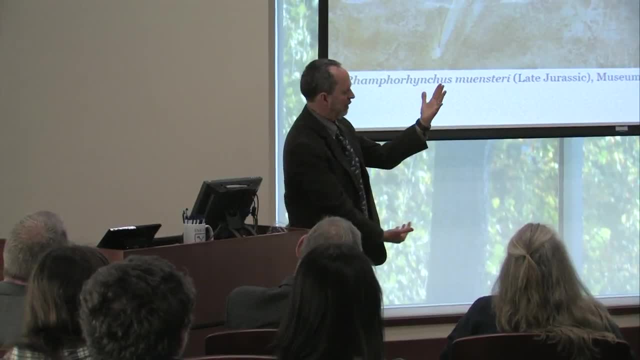 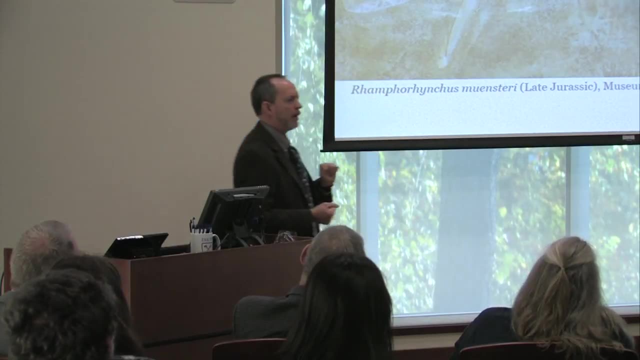 One finger and from that then it had a webbing that it was able to fly with. that had support from some of the other fingers, So they had support on that hand, And then these were worldwide in their distribution, all sorts of ecological niches that they filled. 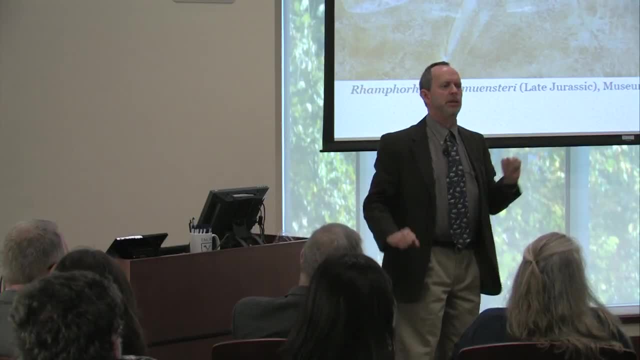 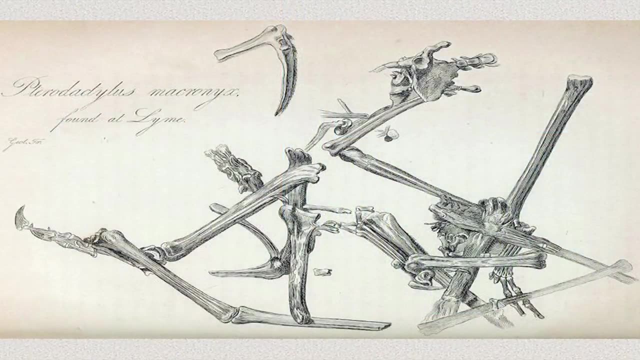 They went everything from sparrow size to wingspan, about the width of this room. Yeah, so some of these were the largest flying animals that ever lived. Some of the bones that Mary Anning found then were reported by some of the paleontologists at that time. 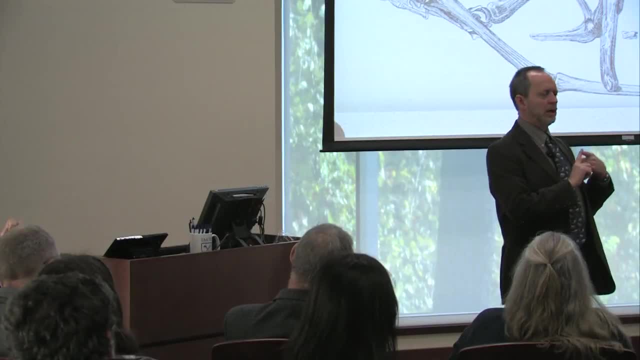 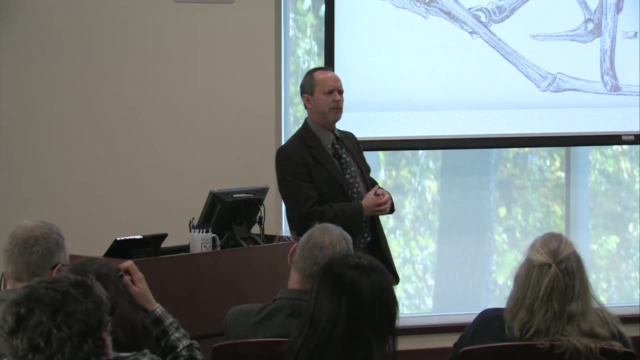 Now, something I should say about her is that she had no college education. She was from a lower working class family, So in a lot of ways she was not shunned but excluded from the paleontological and geological circles and scientific circles of the time. 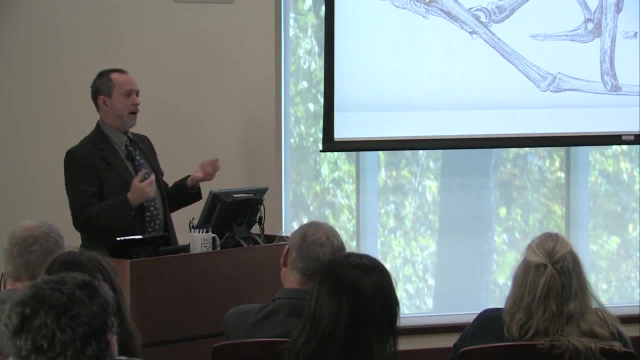 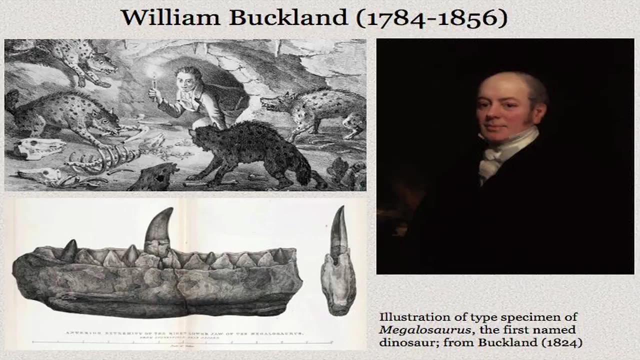 But her discoveries were supported by a few allies, and now I think she has her due as being a famous paleontologist in her own right, And one of her allies was William Buckland- Now William Buckland. he's been described as eccentric. 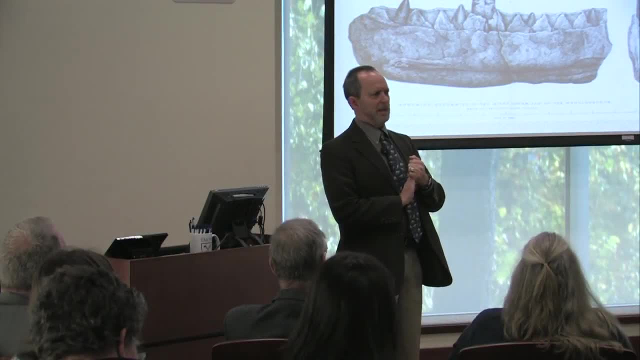 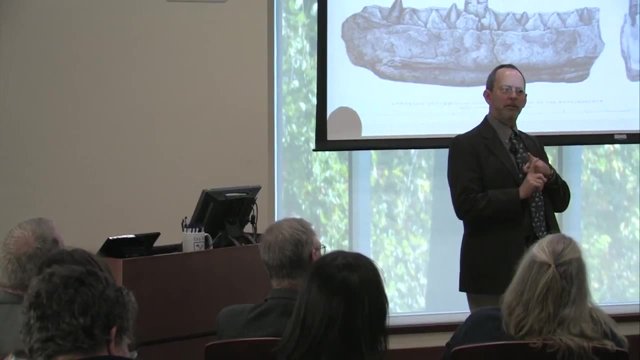 but that would be insulting to the word eccentric. He was downright weird, But he was brilliant. He was a clergyman and a paleontologist. This was really common at this time. Now we see this schism between science and religion by some people. 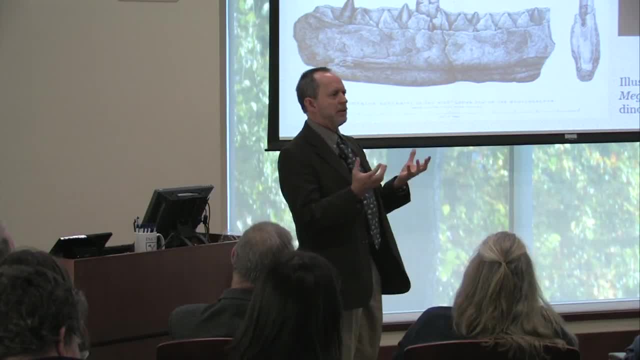 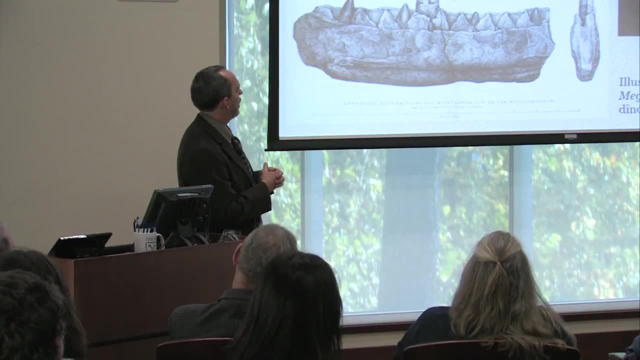 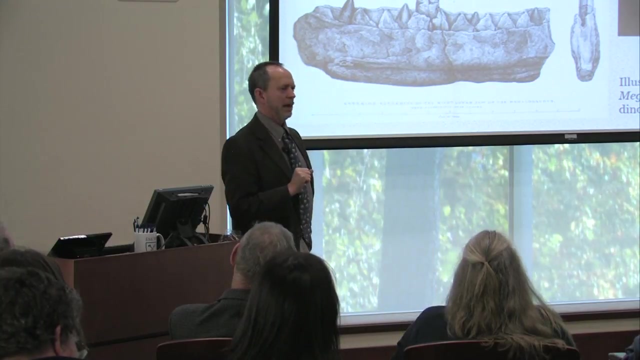 which is actually also mythical. But in this instance, he actually practiced his religion, he practiced his science and he found them compatible at the time. He was a strange guy because he wanted to classify all animals by taste. Yes, So he systematically would taste every animal he could. 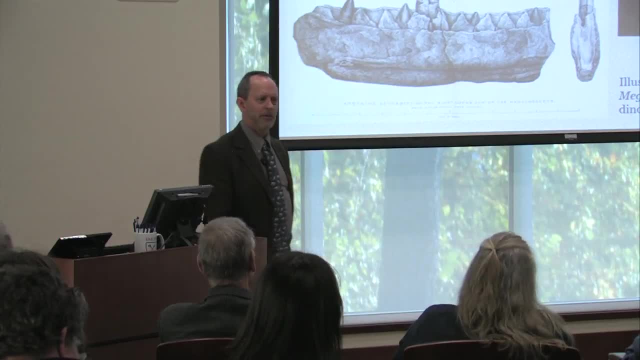 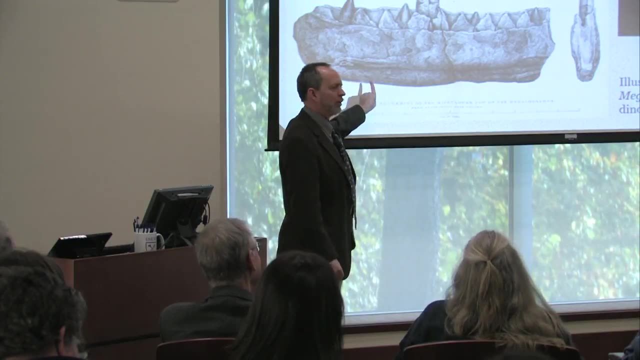 And there are stories of him seeing an animal and just popping it in his mouth. Yeah, so we won't get into the details of that. In terms of dinosaur studies, he actually described the first known dinosaur, Megalosaurus. He did not know it was a dinosaur at the time. 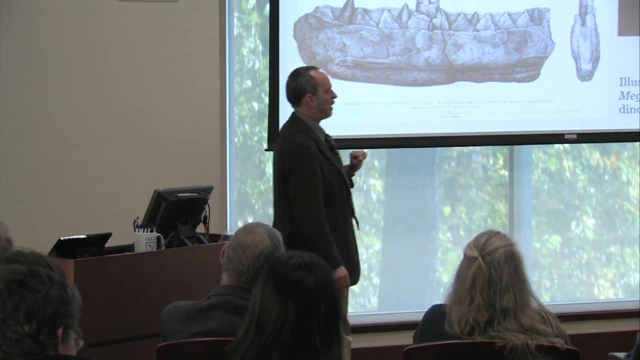 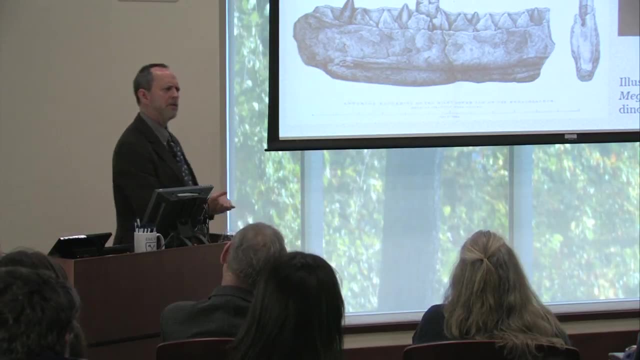 but he did know that it was a formerly carnivorous reptile. He described it as a very large reptile- This jaw was about this long, for instance- And he realized that, oh, this is a very large reptile. And he realized that, oh, this was something very different. 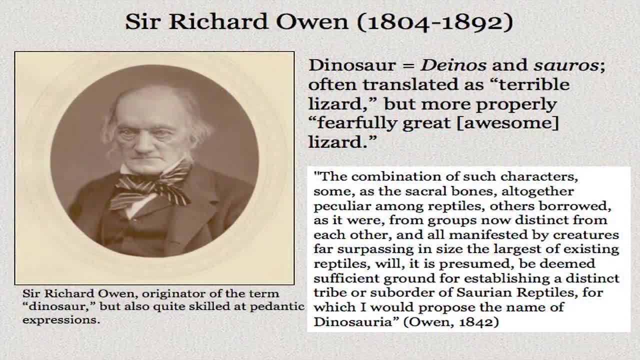 So he described that as a new species: Megalosaurus. Now this rather unpleasant-looking gentleman is Sir Richard Owen. Richard Owen was the originator of the word dinosaur, So if you ever wondered where that word came from, it came from him. 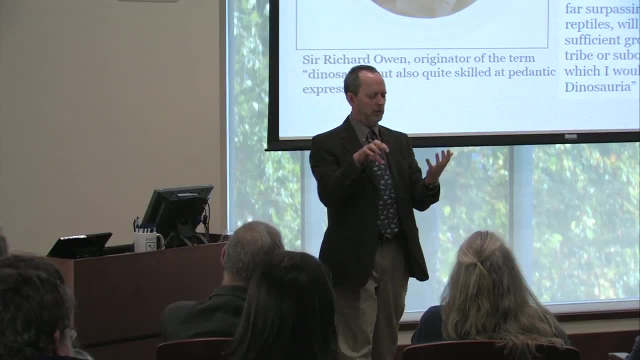 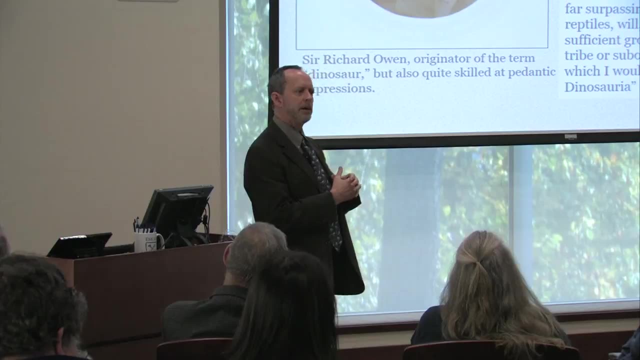 So he recognized, once enough of these fossils were found, that these fossils related to one united, and it turned out they were actually a family-related group. Now, at the time, he was rejecting what would later become Darwinian thought and Darwinian evolution. 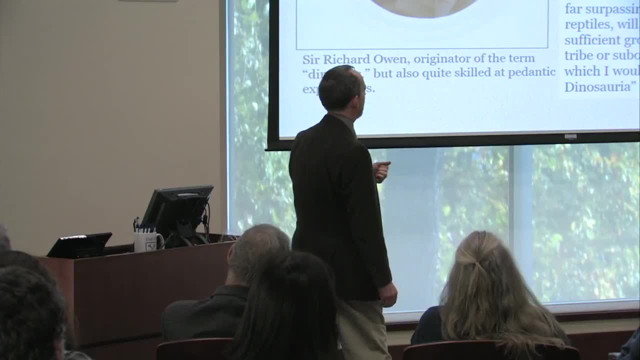 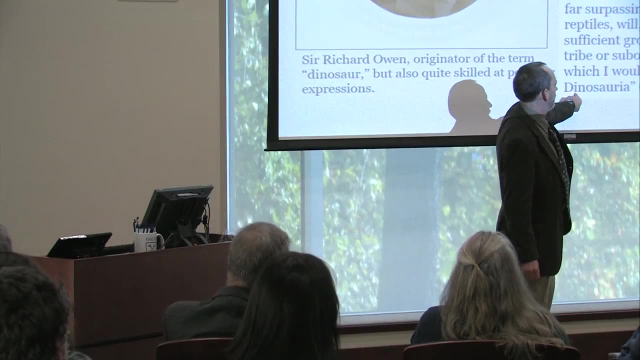 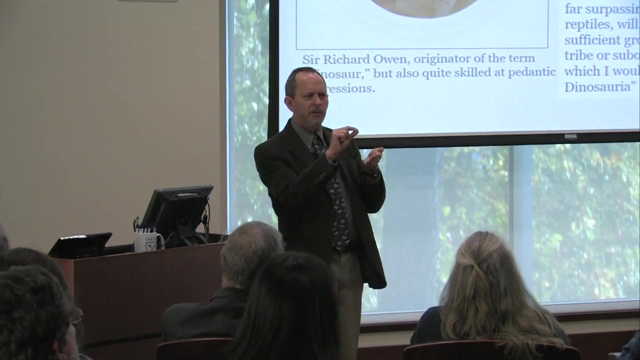 but he did recognize that these were very similar animals, based on their shared traits. So in this very wordy passage which I am going to spare you of, he eventually comes up with proposed the name of Dinosauria. The cool thing about Dinosauria is it translates as terrible lizard. 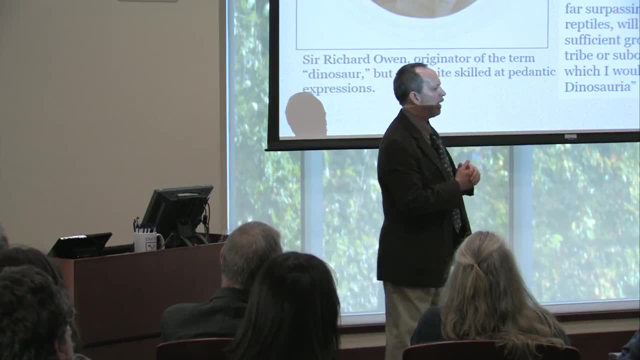 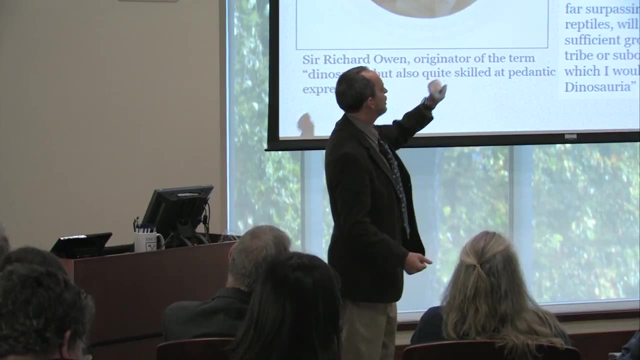 but you have to put it in the Victorian context: Terrible at that time was really really more like awesome whoa. It was more like that fearfully great. Fearfully great, as in you would stand back and admire that giant lizard. 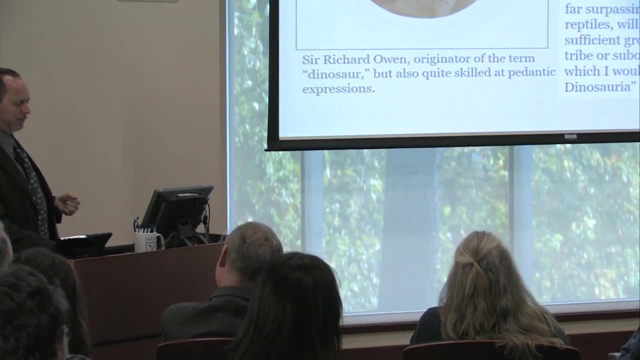 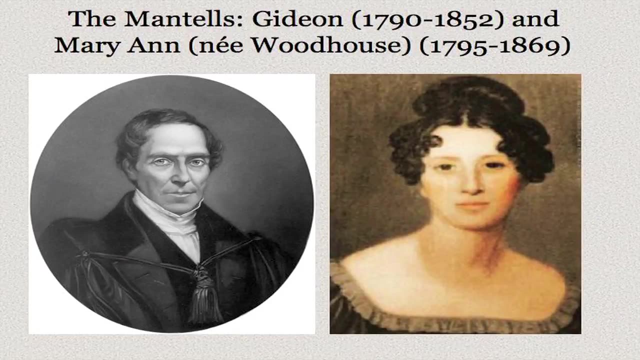 That's the way that it was meant originally. The Mantells also contributed as scientists to this. As a husband-wife team. Gideon Mantell wrote the books and Mary Ann Mantell illustrated them. Now as an illustrator. she had to know these fossils probably. 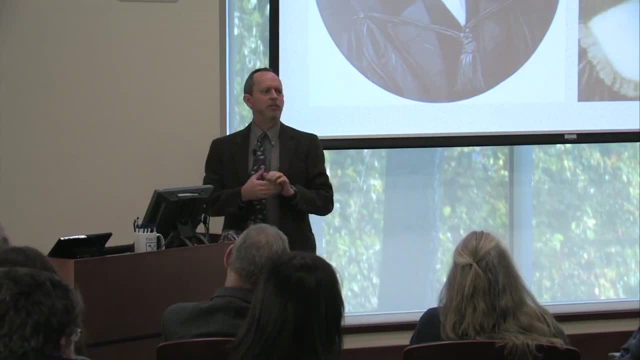 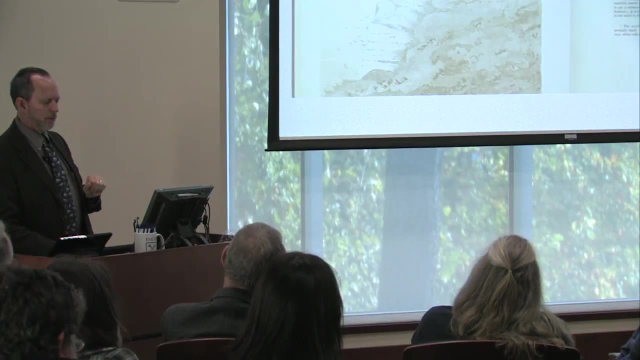 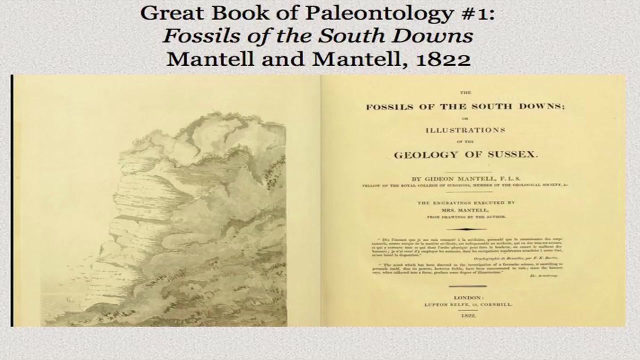 and probably knew the fossils better than he did by the time she finished illustrating them, but they often went out in the field collecting these fossils, and among those fossils they found were some of the first pieces of Iguanodon, A book that he wrote, and I think this is really the first important book for paleontology of this time. 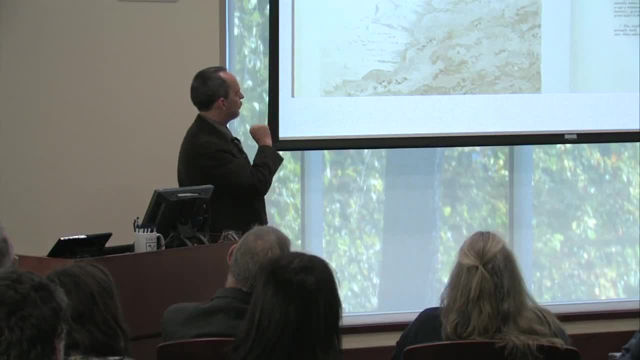 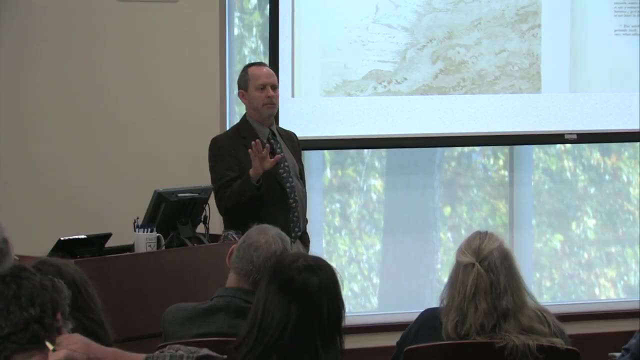 in this place is the Fossils of South Downs And it's more than 300 books, 300 pages. It's a book. I have to admit I haven't read it all. I don't recommend you try to read it. 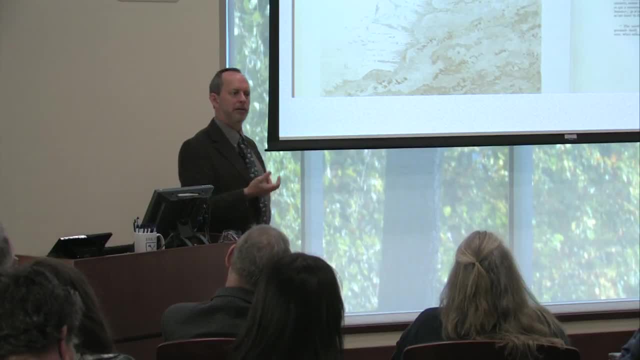 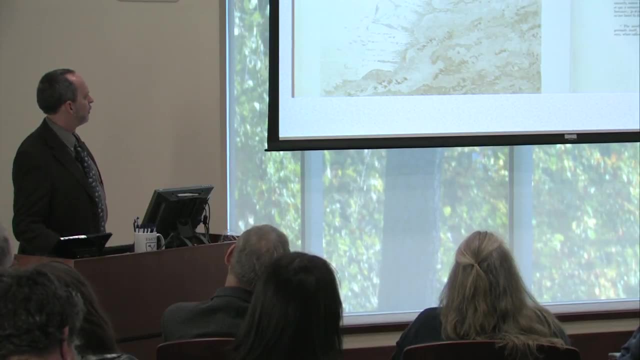 It's not exactly, let's say, the plot doesn't advance well on it, but it is an extremely important book for documenting a lot of these fossils in the southern part of the UK, And I think it's important also for those of you who are pre-med. 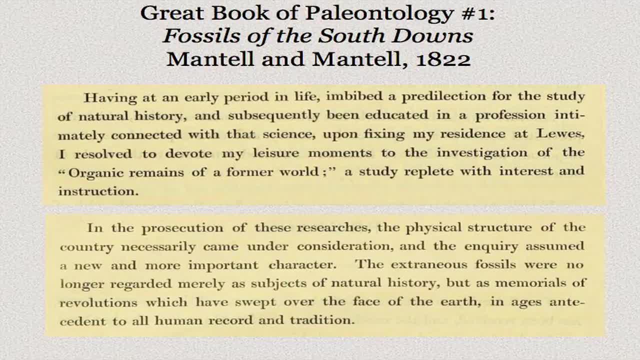 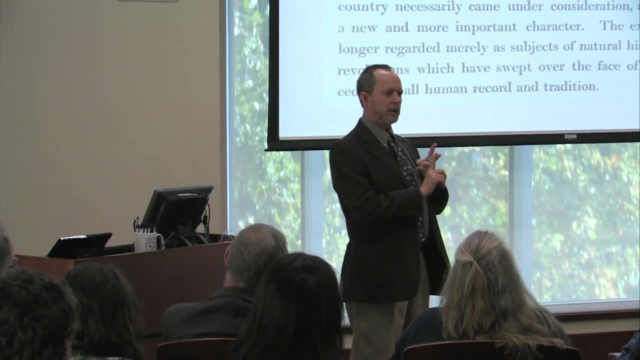 You're planning to be physicians. He was a physician. This was something he did in his spare time And this was also common. There were a lot of paleontologist clergymen and a lot of paleontologist physicians at the time. 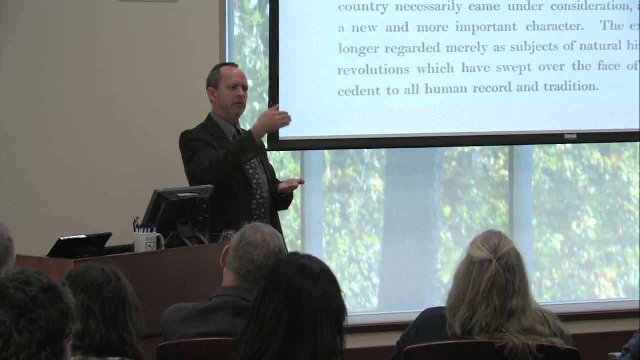 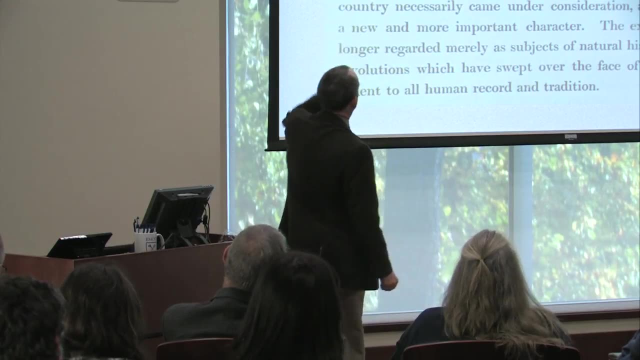 That this was something that they had some training in biology, so then they applied more of those biological skills as naturalists. So I like this first line where he's talking about how, as a physician, he doesn't say the word physician, but he's talking about how, in his profession, he's connected with the natural sciences. 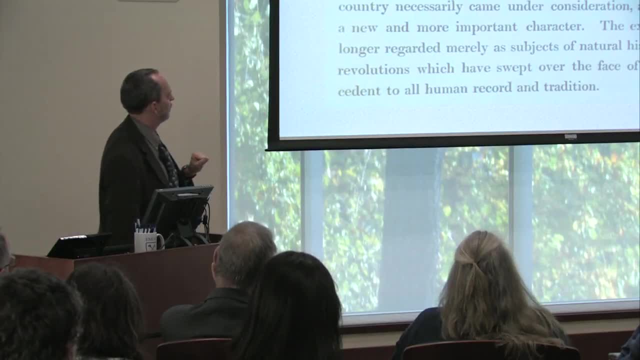 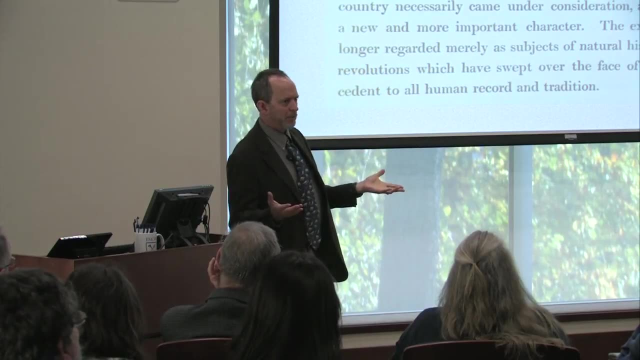 Down here. then he talks about the importance of this in terms of the extraneous fossils no longer regarded merely as subjects of natural history. later on that would be called stamp collecting. but it's not as memorials of revolutions which is swept over the face of the earth in ages antecedent to all human record and tradition. 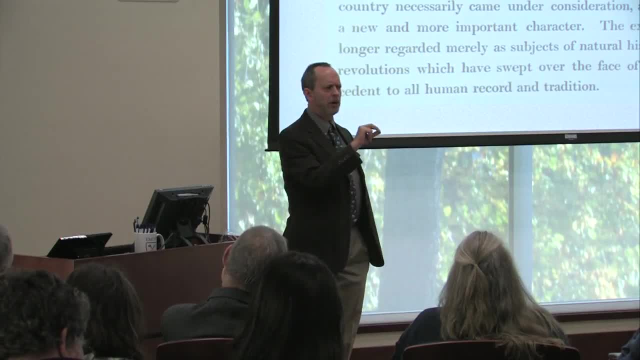 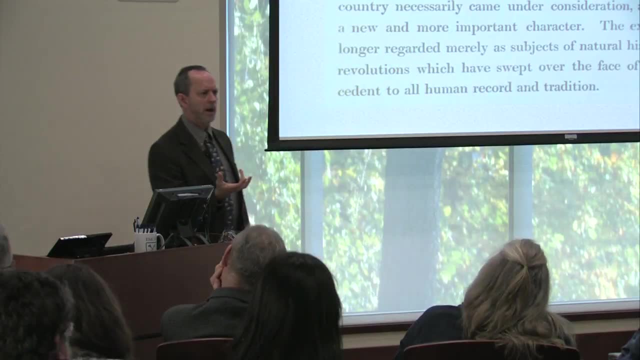 What's important about this, then, as a book, is he's starting to think about a time before there were humans, And this was going against a lot of the religious grain at the time that was saying that, well, there were some catastrophes. 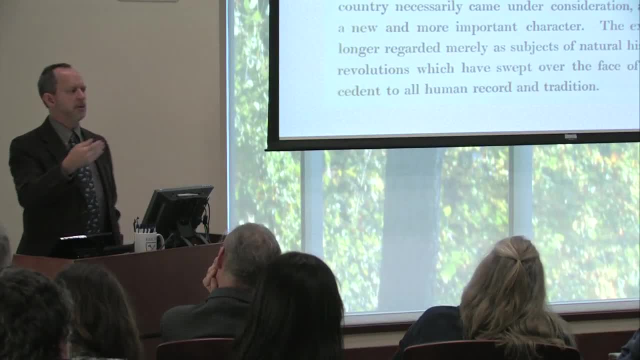 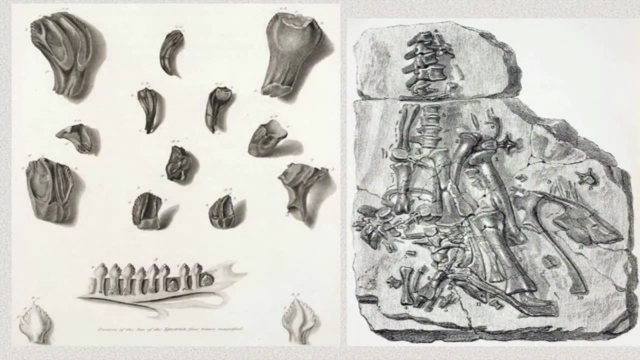 and humans were there right from the very beginning. Instead, he's hinting that here's a fossil record showing that there's a gap between those. So these teeth were initially identified by Baron Cuvier as being rhinoceros teeth. They were not. 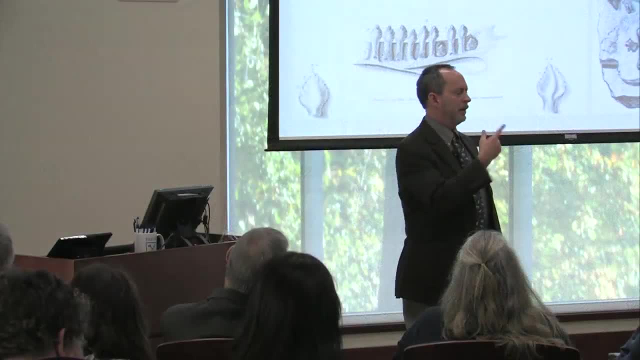 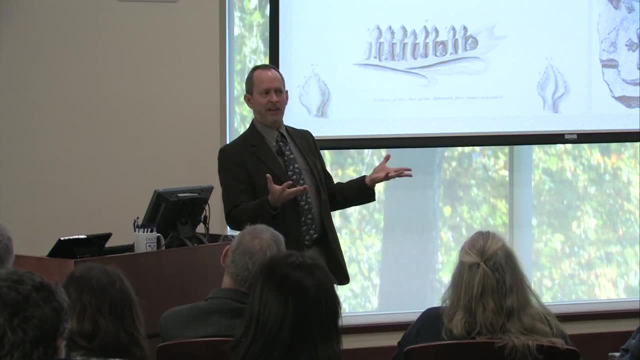 They belonged to a very large reptile. He thought Mantel thought these belonged to something like an iguana, but it was elephant sized, so that's not an iguana. He named it then iguanodon, which means iguana-like turtle. 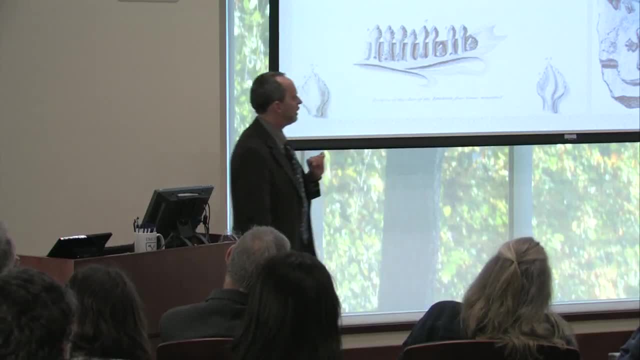 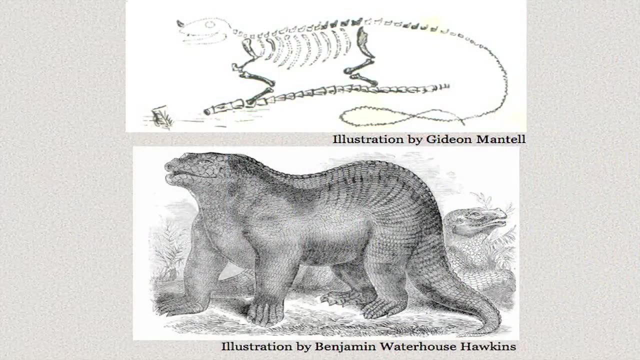 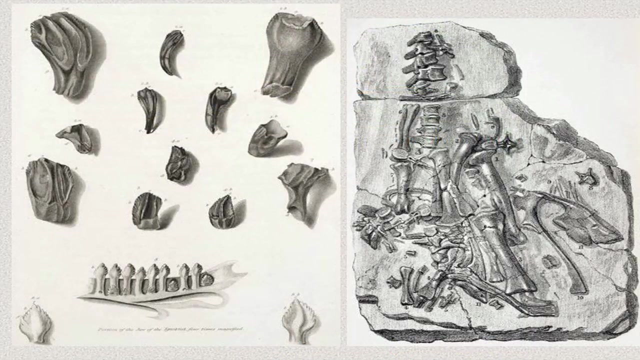 The bones that they found, in association with the teeth, were enough to describe the specimens. and this was the second named dinosaur called iguanodon. Now, as you can see that top illustration, he should have left the illustrating to Marianne. Look at her illustrations. 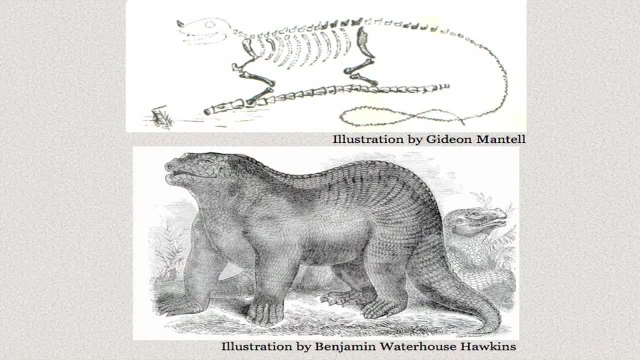 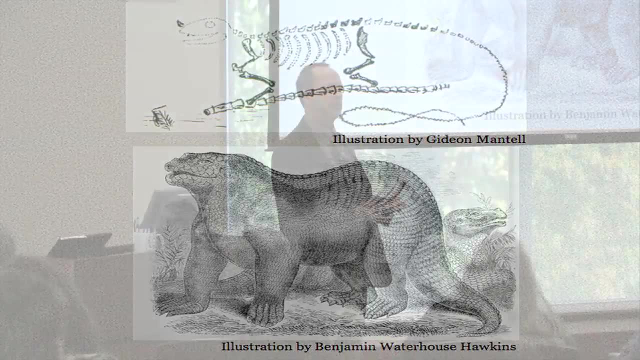 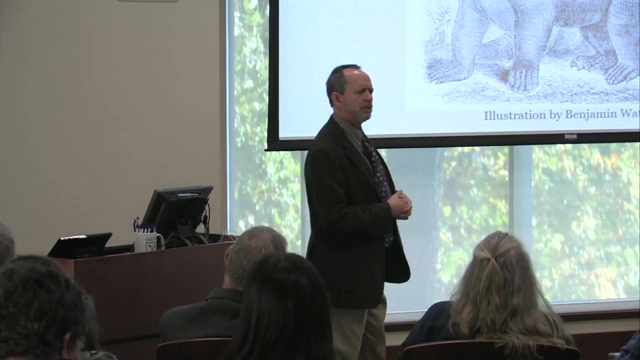 Look at his. Okay. but also you had very skilled illustrators at the time who tried to reconstruct these animals in life position. It looks kind of weird. It looks kind of weird to us now. It doesn't look like any dinosaur that we would see recreated today. 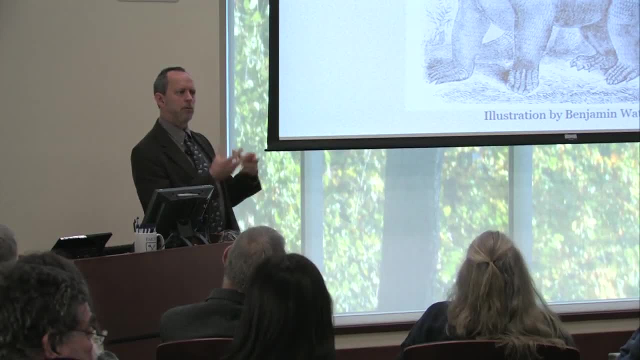 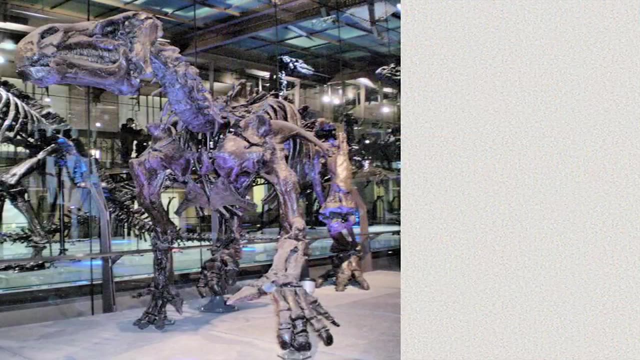 But nonetheless this was some of the first attempts to reconstruct these animals based on just their fossil remains. This is what iguanodon looks like. It turned out that there were complete specimens found in Belgium. more than 50 or 60 individual iguanodons found there. 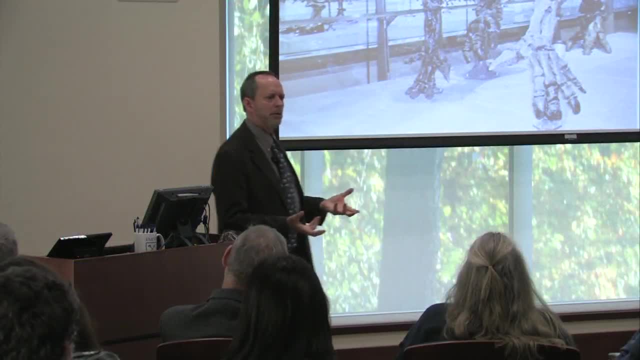 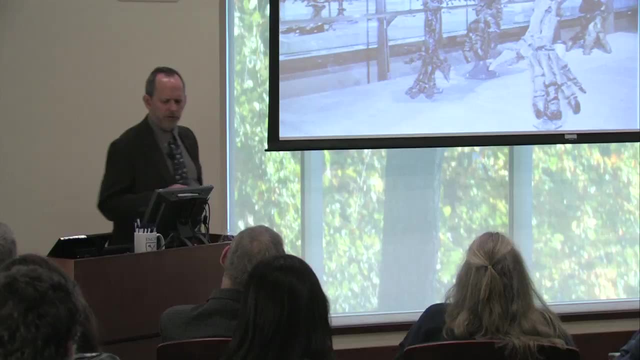 whole skeletons, entire skeletons that they were able to reconstruct. I understand there's a museum in Brussels you can go to and see dozens of these mounted specimens there. This is from about 100 million years ago, Large herbivore with these more grinding teeth here. 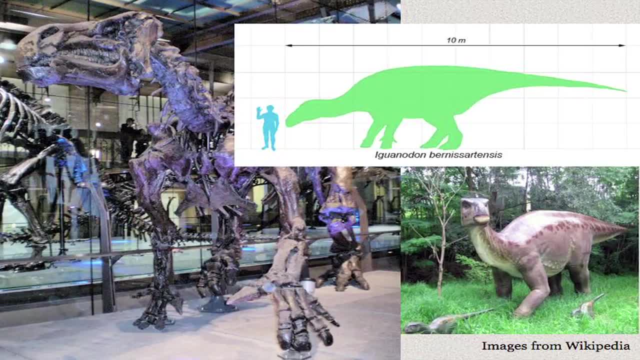 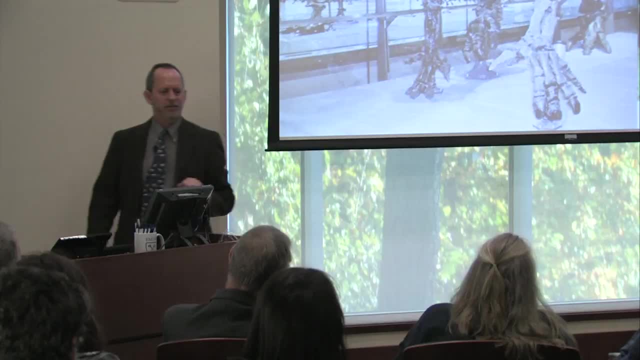 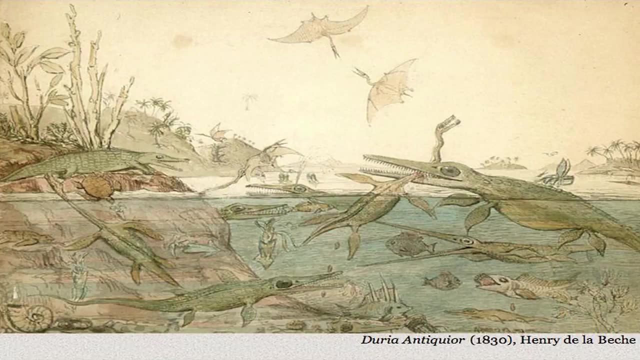 About six to seven ton animal. That's how it would look compared to clueless waving guy there next to it, And then a life reconstruction there as a statue. I love this illustration because this is a statue. I love this illustration because this is the very first attempt at recreating an ancient ecosystem through art. 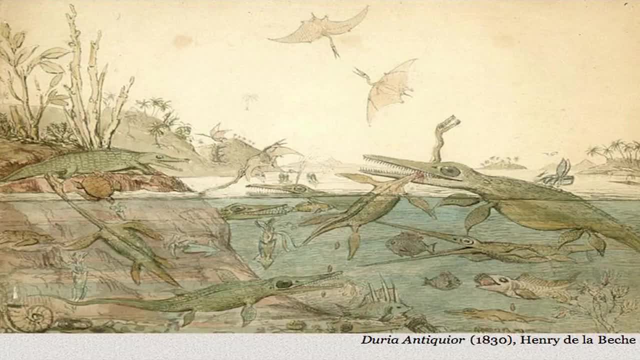 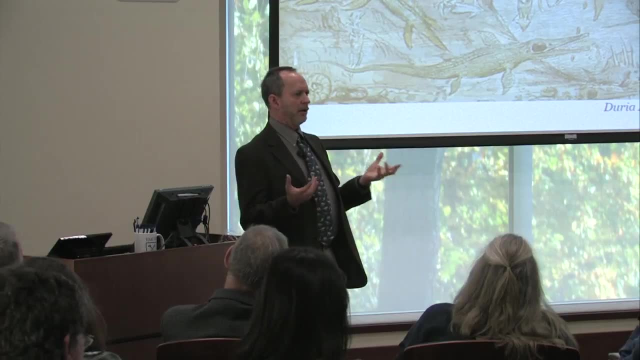 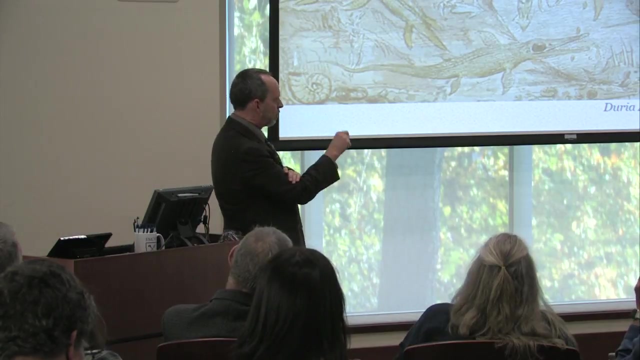 This was 1830.. The artist is: he was a paleontologist, geologist and an artist. This, again, was very common at that time. A lot of artists also did science and there was no division between those two In this reconstruction. I love the completeness of it because, thinking ecologically, 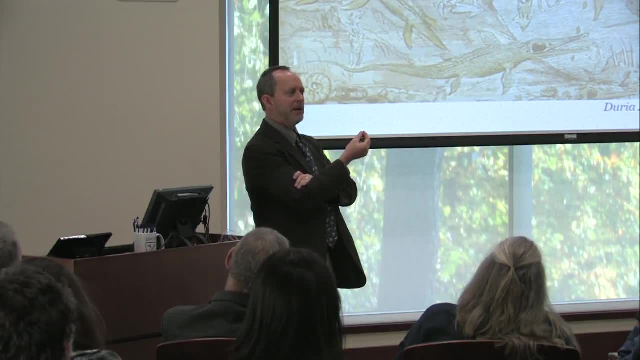 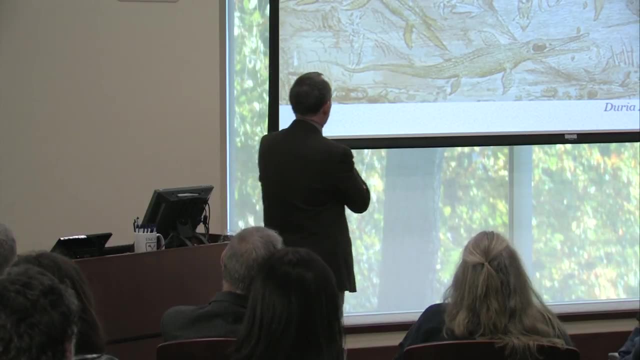 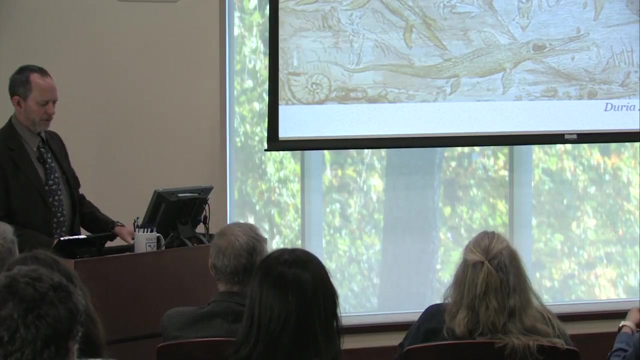 you see a pretty fierce food web going on. Everything is trying to eat everything else. So yeah, it looks a little Hobbesian, too Hobbesian for me. I also like the. I appreciate the detail of this. one is extruding some future coprolites or fossil feces there as well. 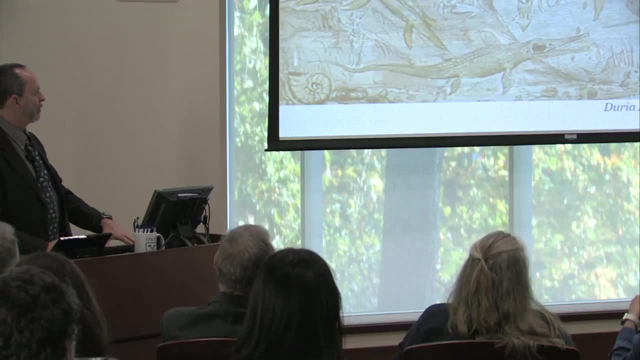 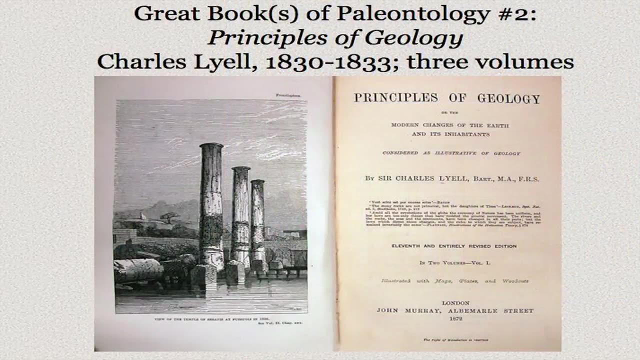 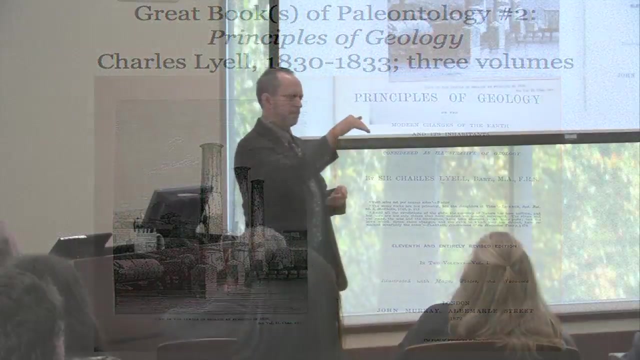 So he really has good attention to detail all throughout this. But the first reconstruction of an ancient ecosystem by using art. The second classic book of paleontology and geology is actually more geological, but paleontology is woven all through it because those two sciences really intermesh with one another. 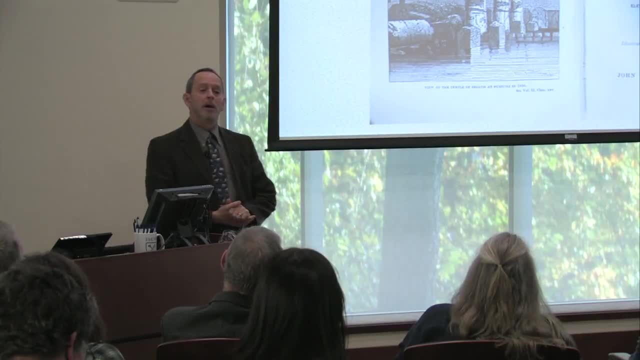 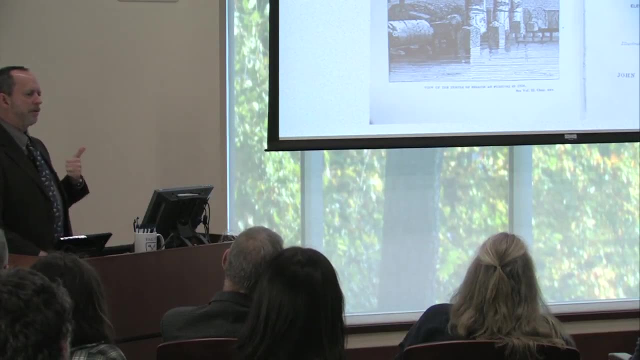 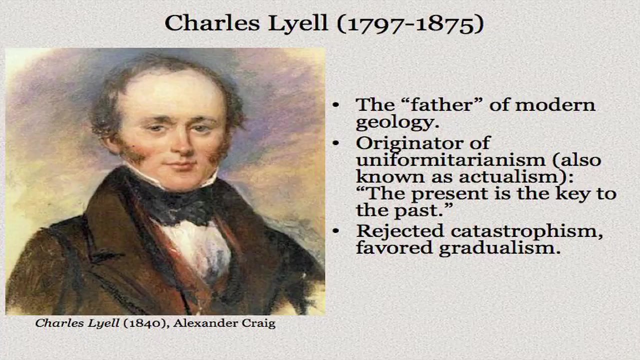 And this is Lyell's Principles of Geology, Three volumes. three volumes: Very thick, thick book in terms of laying out the modern principles of geology. So oftentimes he's called the father of modern geology And the originator of a very long word: uniformitarianism. 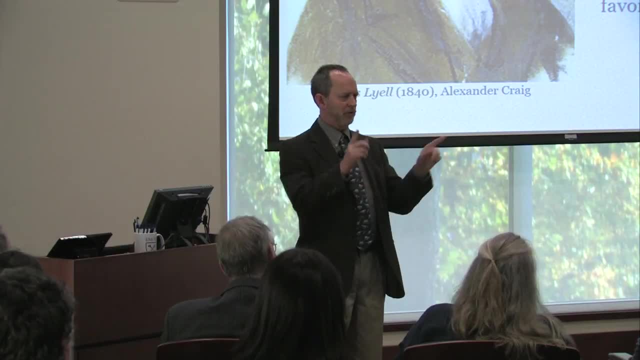 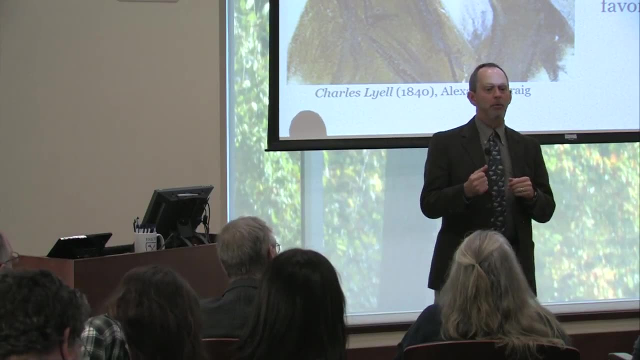 How many of you can say that uniformitarianism? A couple of my students in the audience probably can, but I'm not going to have you do that. Sometimes we use a shorter name: actualism- that in what we do is we look at the actual environments today. 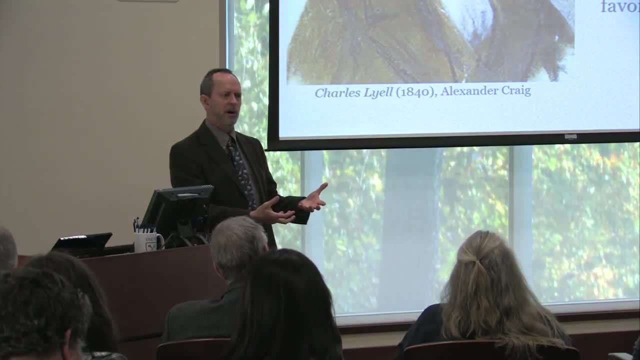 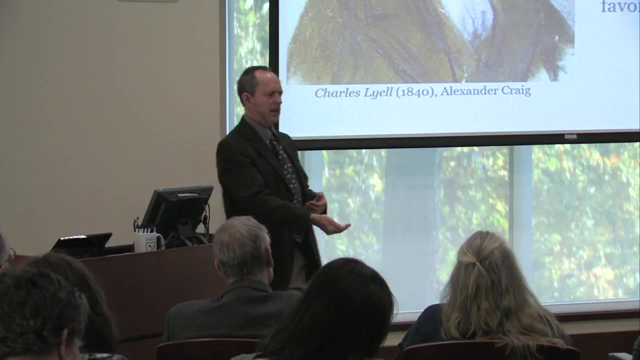 and we use the processes that we see today in those environments and assume they were uniform in the past And we apply them to what we see as the products of those processes in the geologic past. So footprints, ripple marks, mud cracks. 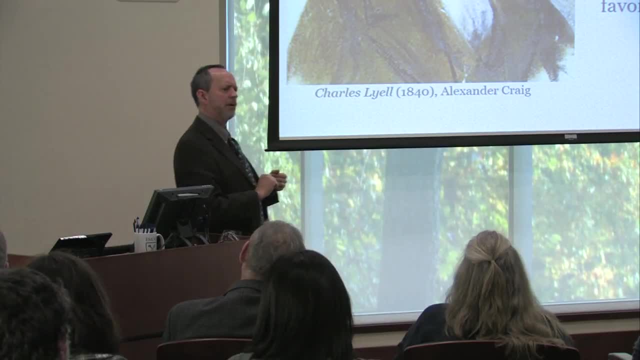 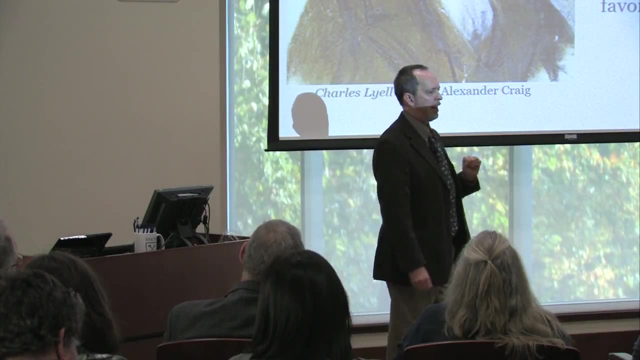 If we see those in rocks, we can assume that they're very similar to how they form today. Now, an important thing philosophically about Lyell was that he rejected catastrophism Because before the religious thinking in Christianity-based religions at the time in Europe. 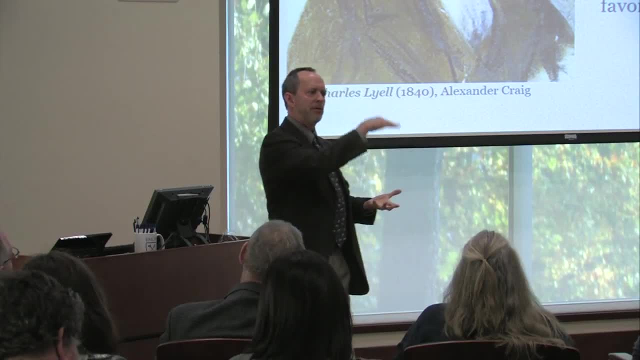 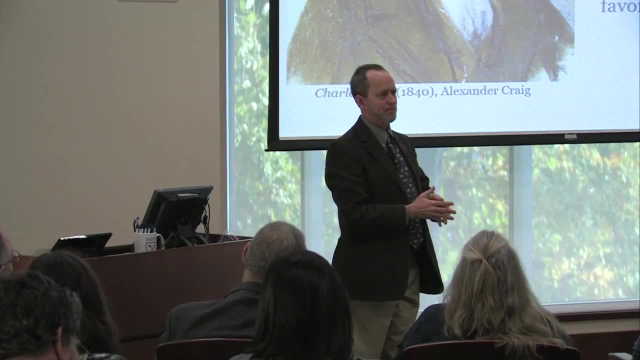 were that there was a great flood And the great flood was responsible for everything we see in the geologic record. He rejected that and favored more of gradualism, Gradualism. Gradualism requires time, And this is the big revolution then that happened in scientific thought. 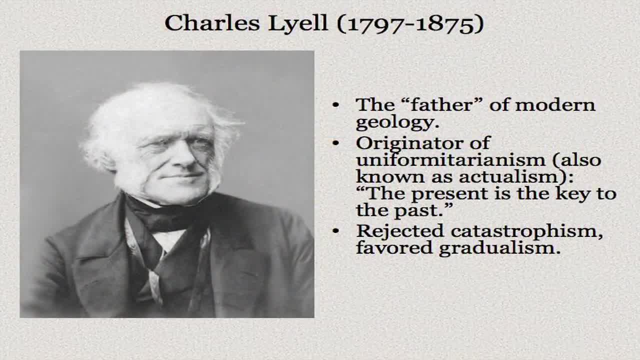 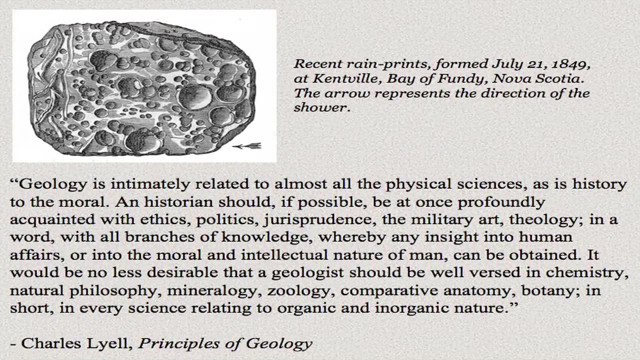 was thinking about time and this fourth perspective. So there's Lyell, from a young man to an older man And as a geologist, he is still in our minds today, in that I and every other geologist, we are still applying those principles from that book. 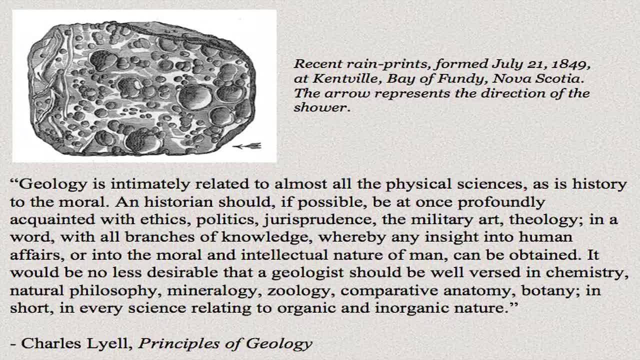 And just a quote in here. I love It is how geology is the most eclectic of the sciences And we're very proud of that. And he makes an allusion here to looking at how history a historian- how about that? huh? 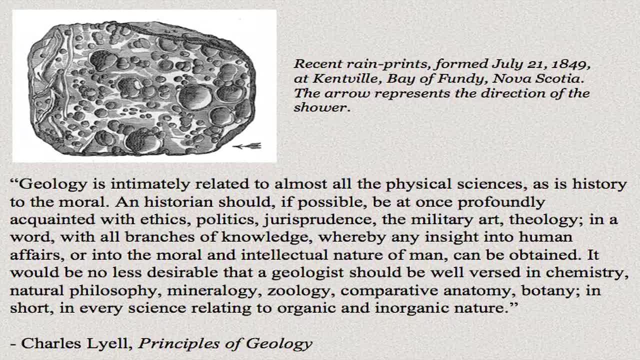 A historian should, if possible, be at once profoundly acquainted with ethics, politics, jurisprudence, military art, theology- all branches of knowledge. You got that covered right. Good, Okay. And into the moral, intellectual nature of man. 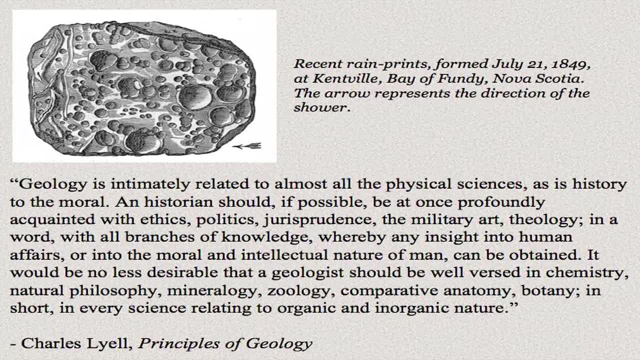 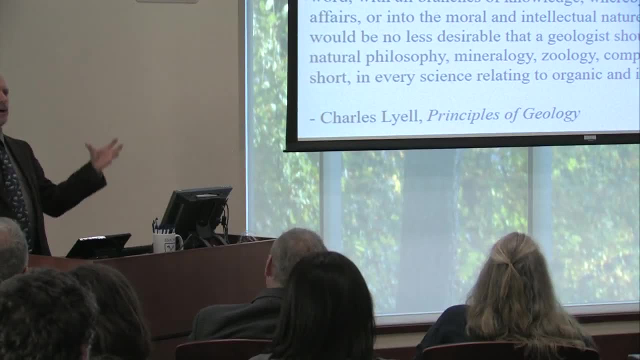 Look at geology, Chemistry, natural philosophy, mineralogy, zoology, comparative anatomy, botany. In short, every science relating to the organic and inorganic nature. Yeah, we're kind of cocky about it, Geologists. we are proud of this, in that we do try to touch on all the sciences and unite them. 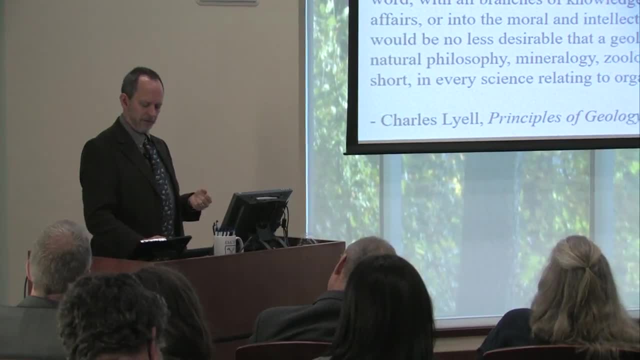 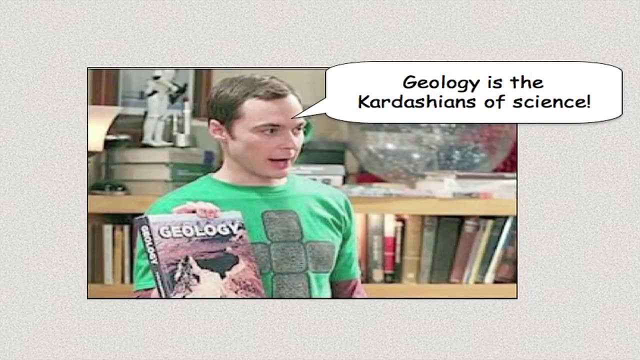 And I think Lyell in this book was able to articulate that for the first time. Now some people might disagree with him on that, And we do get some pushback from our physicists And our physicists friends And our chemists friends. 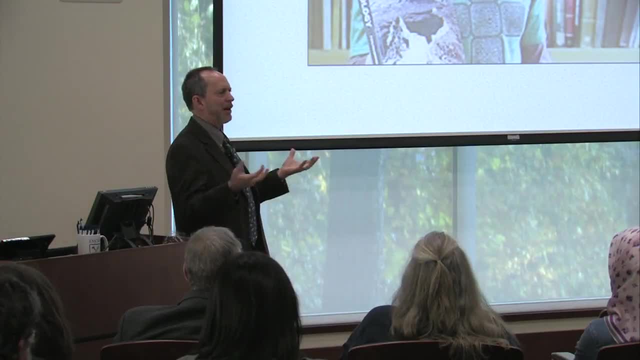 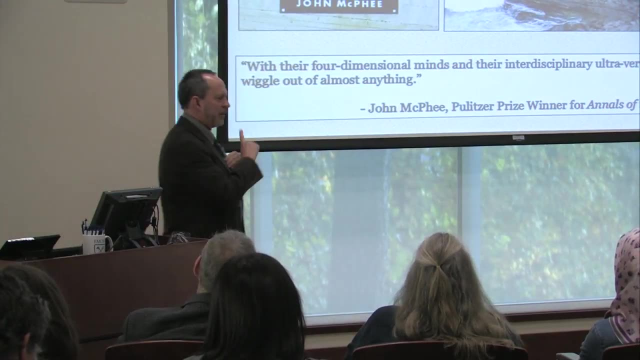 And our biologists friends, But we're fine with their pushback because we work with all of those sciences too and admire what they're doing as well, And I like what John McPhee in this book- and it's actually a three-volume book- Annals. 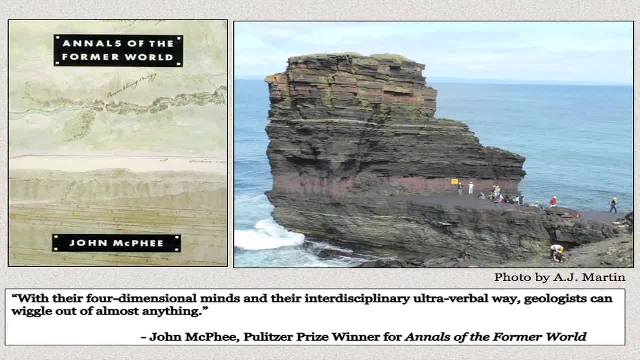 of the Former World. John McPhee is a famous non-fiction writer who oftentimes has written about geology and geologists with their four-dimensional minds- the fourth dimension being time- and their interdisciplinary, ultra-verbal way. Yes, we are quite verbal. 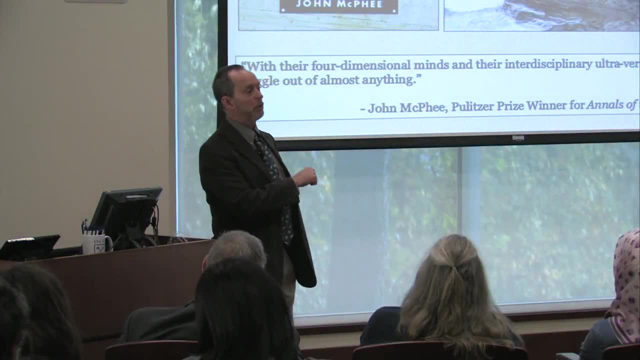 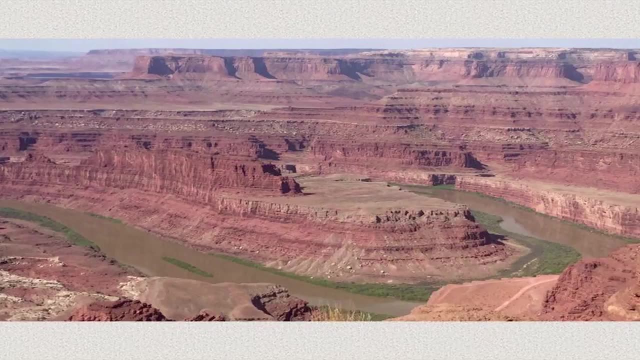 Geologists can wiggle out of almost anything. Also, true, Guilty, I will admit to that. But here's what happens when you get a geologist out in the field. They look at the landscape and they see time. So I look at that and I go ooh, ah, wow, that's cool. 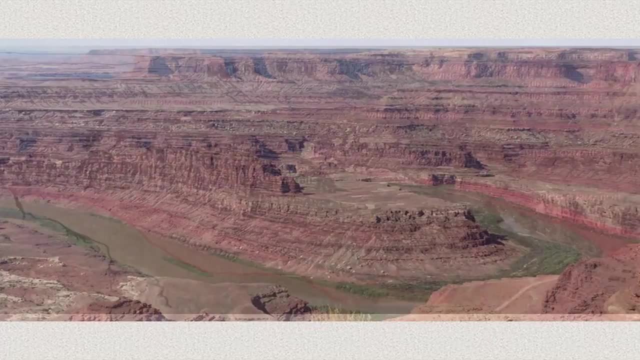 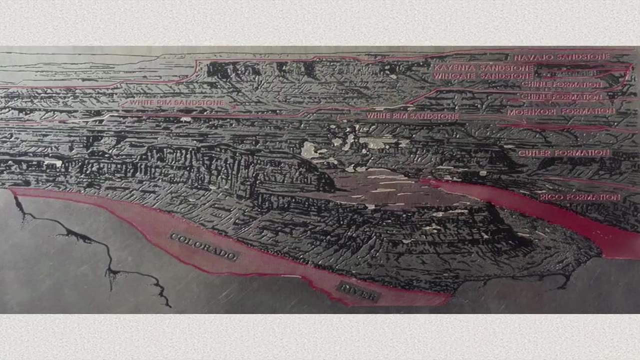 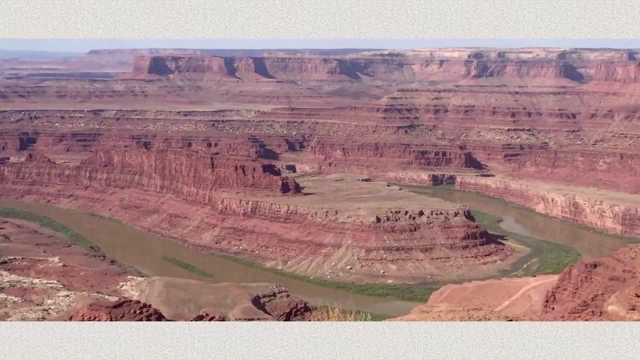 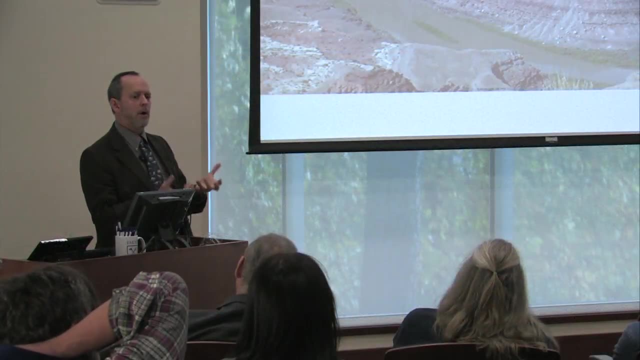 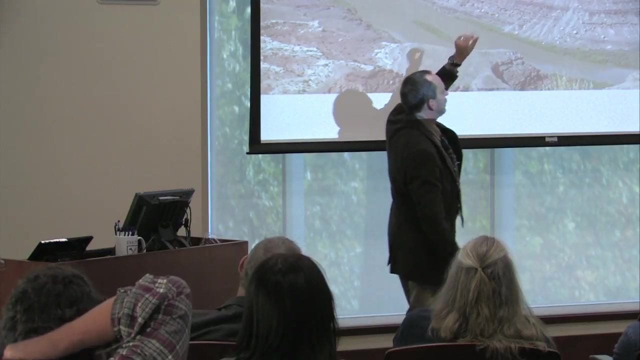 And when we look at those sequences of rock- this is in Dead Horse Point Canyon State Park in Utah, near Canyonlands National Park- When we look at these rocks, we see a book, that this is a book of rocks, where the story starts down here and it goes up from there. 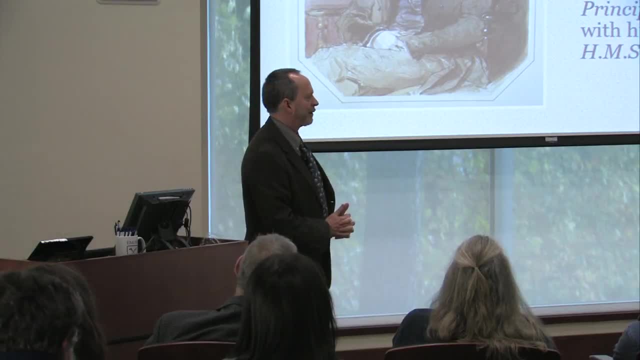 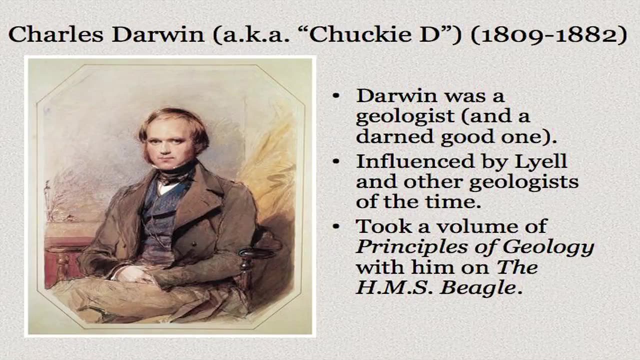 This is where we get to Chuck E D. OK, Charles Darwin was a geologist. How many of you did not know that? Come on, There should be more hands going up. There you go. Good Yeah, The biologists like to claim Darwin. 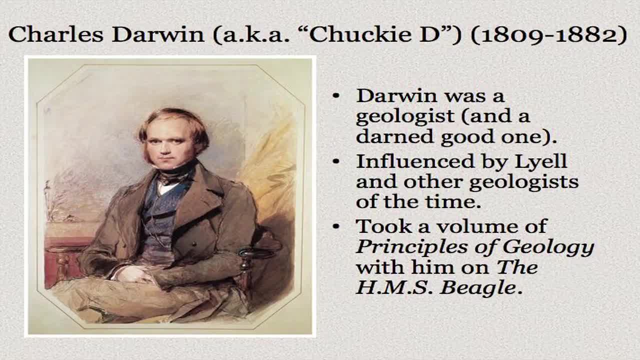 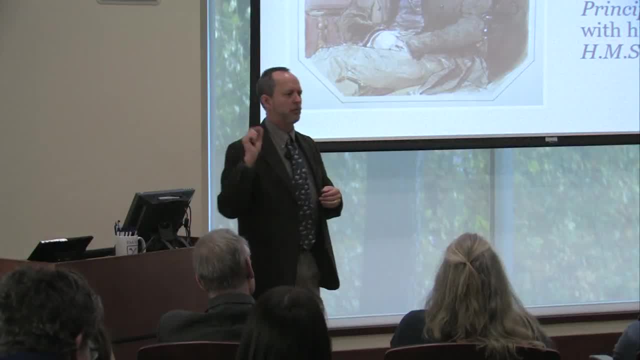 And that's fine. He was a biologist. Yes, He was a fantastic biologist And he's credited with the theory of evolution. He was also a fine geologist. He won medals for his geology knowledge, So he was trained as a geologist. 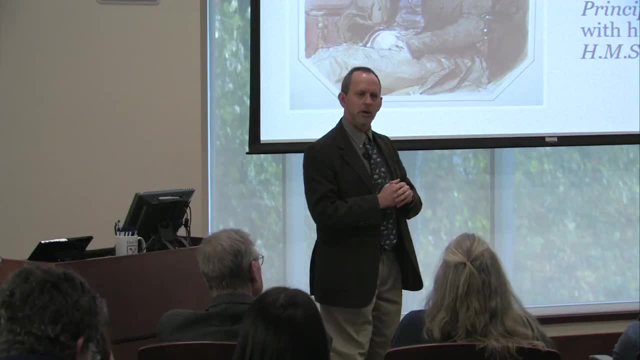 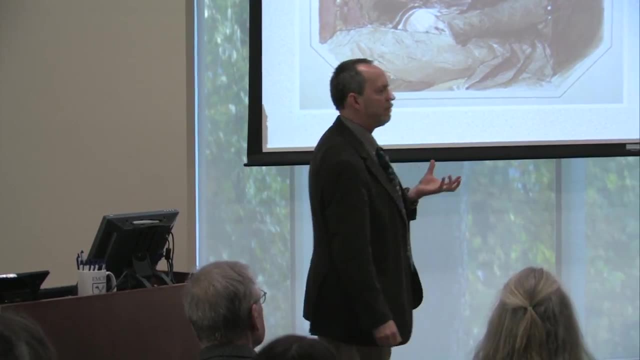 He followed the principles of geology. He took a copy of Principles of Geology on the HMS Beagle with him when he went around the world, So he was influenced by geologists when he was coming up with the theory of evolution during this five year journey. 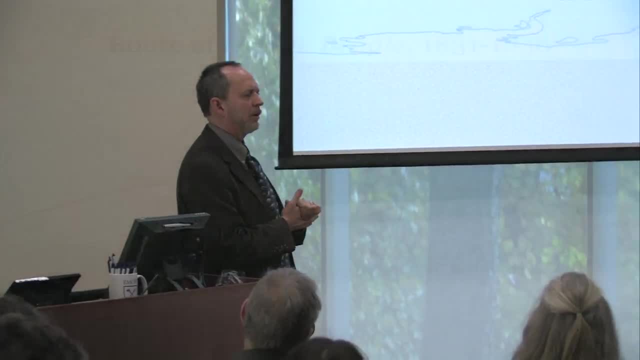 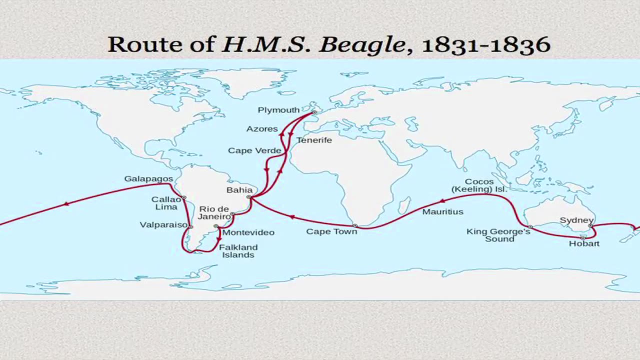 So I've included his book, The Voyage of the Beagle, because I think this was a really important book, for if he had not done this journey, if he didn't have the geological training, if he wasn't aware of fossils, that he would have had a tougher time coming. 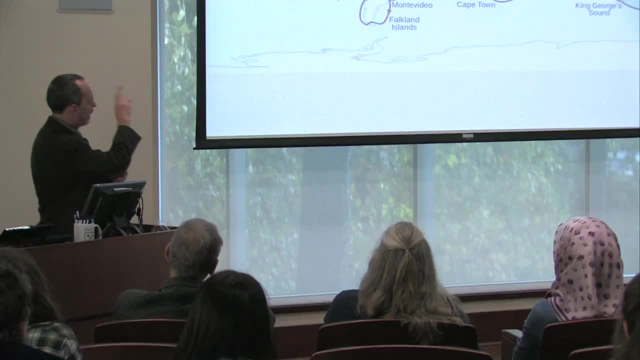 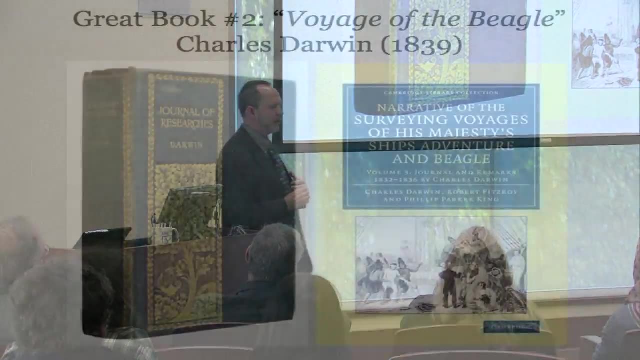 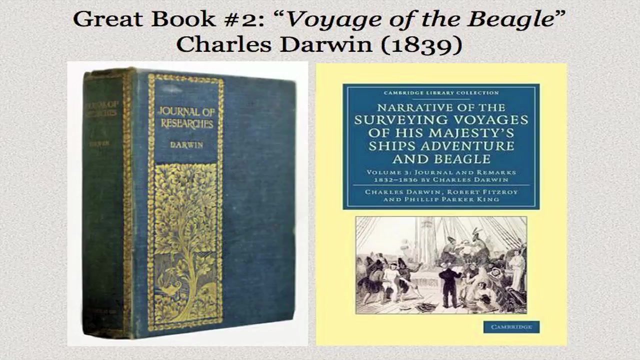 up with theory of evolution, And this shows where his root was, where he went around the world for five years. So I put this book in here instead of his The Origin of Species, because I feel like this was a more important book in terms of his having this five year adventure. 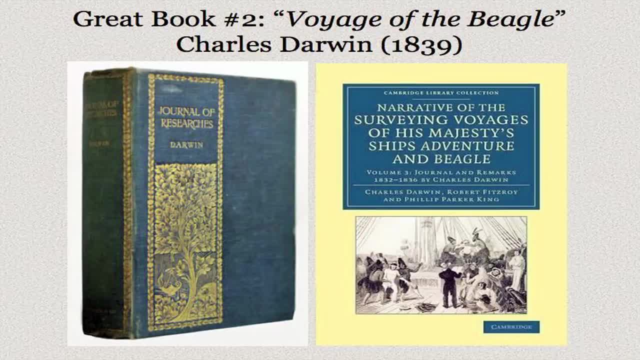 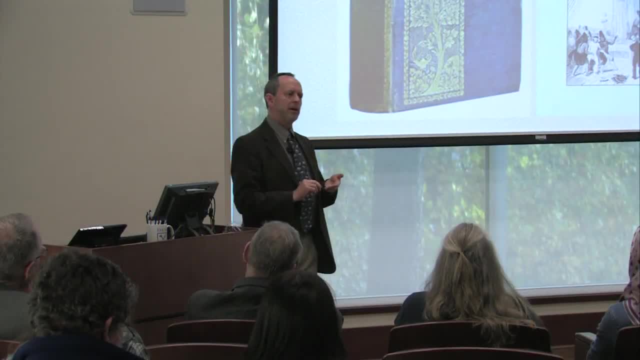 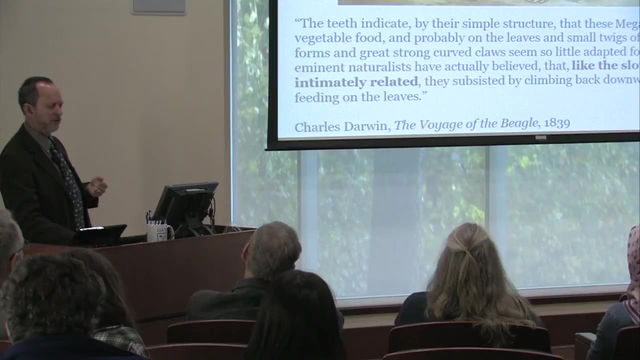 And there really should be Darwin action figures. There really should be Because this five year adventure he had sailing around the world where he was documenting all of his observations That paleontology is a very important thing, That paleontology and geology were both intrinsic to his observations. 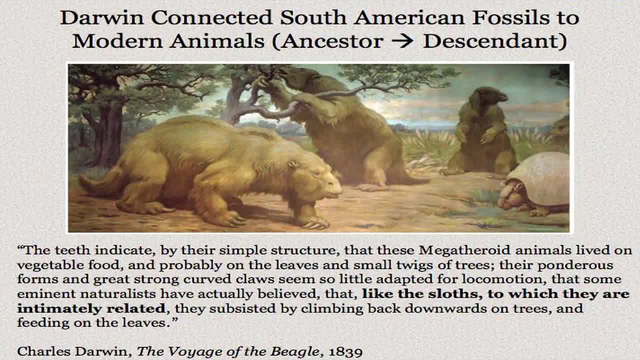 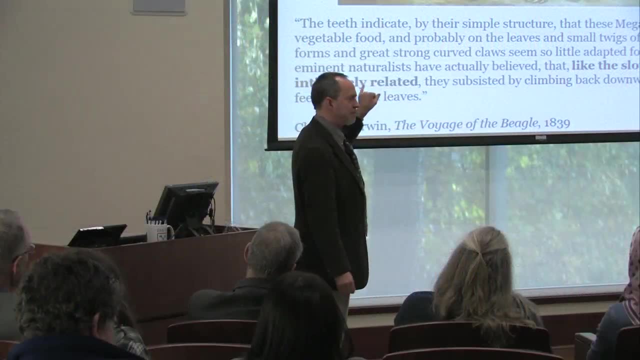 And one of the best connections I thought that he made during this journey was these giant ground sloths depicted here in this painting by a famous paleo artist, Charles Knight of the 20th century. These giant ground sloths that these were four to five ton sloths and, as you can see, 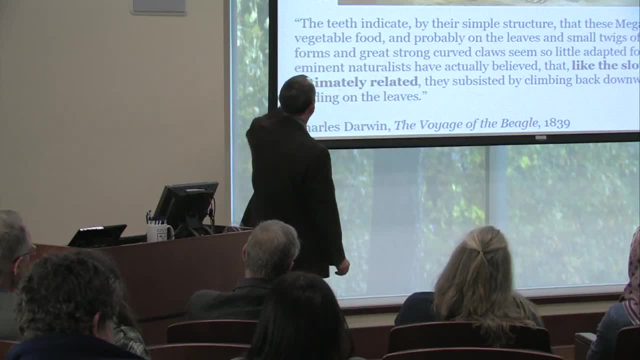 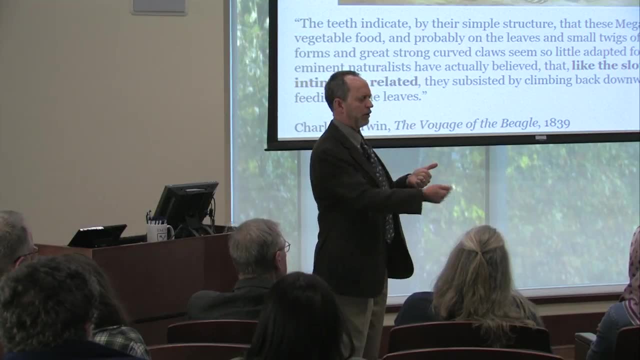 ground dwelling and eating from the trees. Darwin is making some interpretations of the fossils he saw in South America. So these fossils of giant ground sloths, we have them in North America as well that he saw these fossils and he inferred some of their abilities. 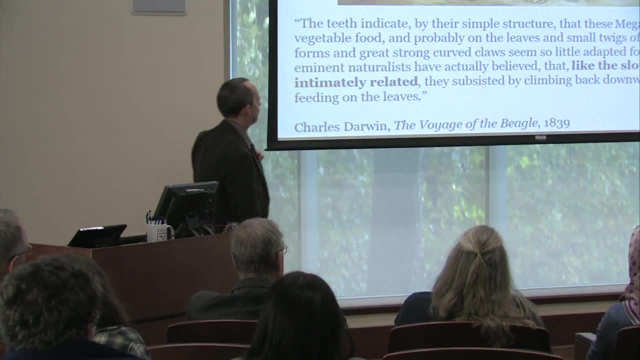 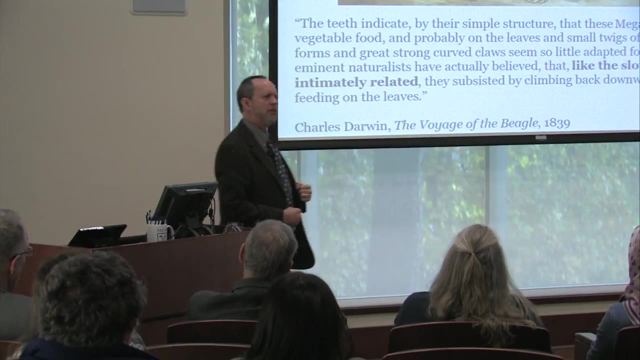 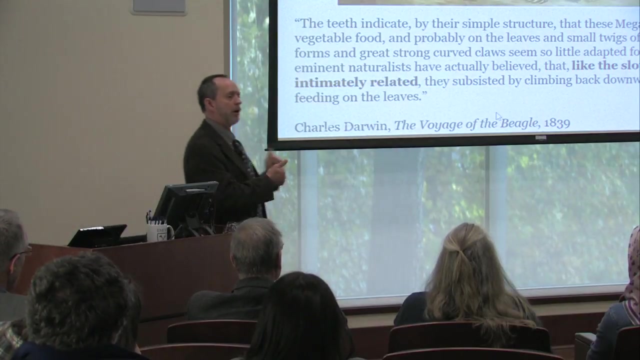 So the great, strong, curved claws seem not so well for walking but very good for tearing off vegetation and eating, But also- and I bold, faced it here- like the sloths to which they are intimately related. Here's where he started doing what's called biogeography. 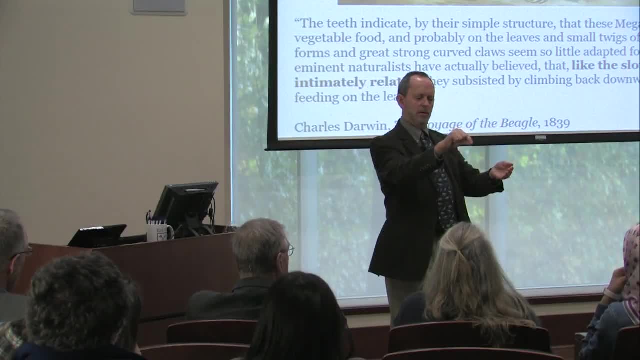 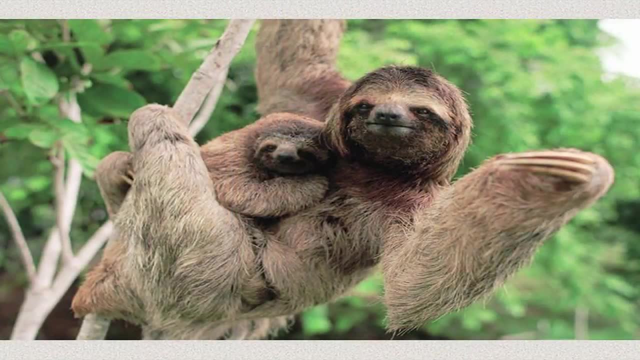 He started connecting the fossils where they were with the modern animals in the same places, Because in South America and Central America you have these right, And who doesn't love a sloth right? So these tree sloths are descended from some of those animals and then we get other aberrant. 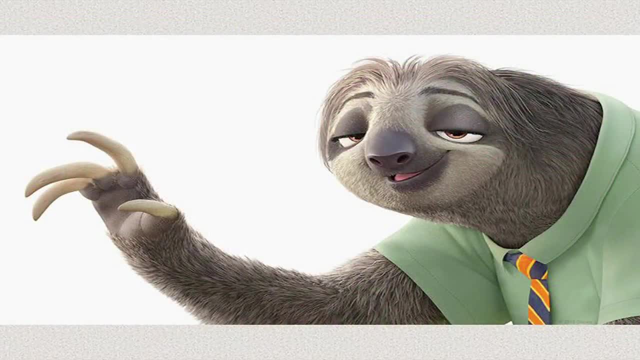 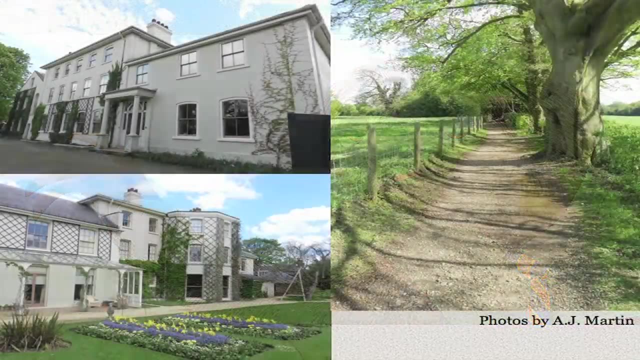 forms like these that we might see, And I'll do the rest of the talk then imitating this. No, I'm kidding. No, I'm not going to do that For those of you who saw the movie. Okay, So, while Darwin was at Down House, this is just south of London- you can go there, visit. 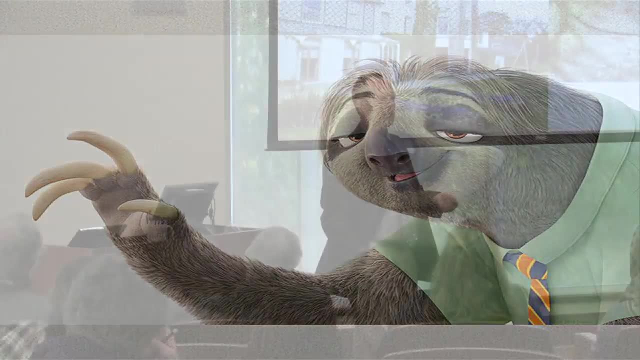 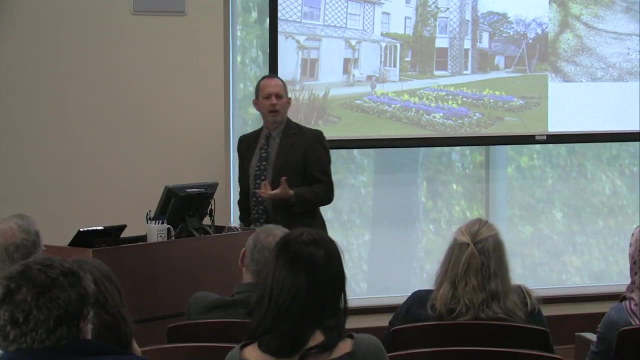 where Darwin wrote this book, also wrote Origin of Species and a bunch of other books, And when he was out for his daily walk on the sand walk, he was thinking about these ideas, and many of these ideas involved what he learned originally from Charles Lyell. 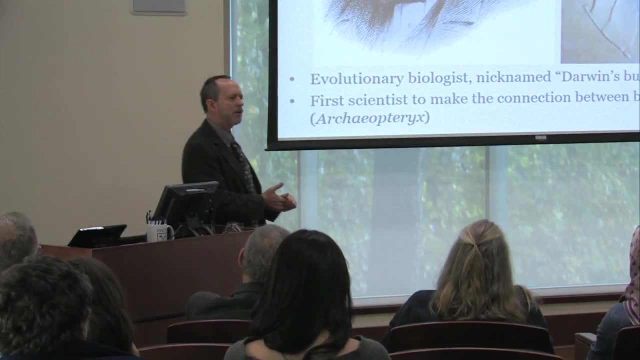 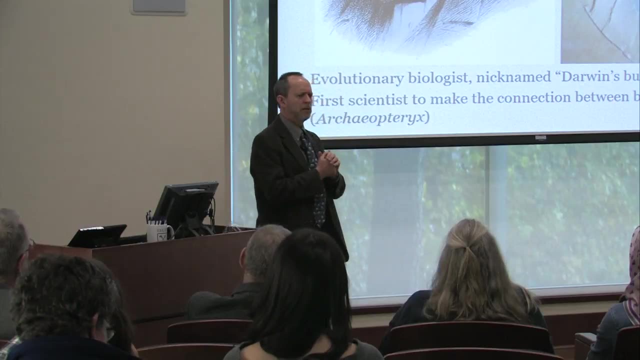 Principles of Geology. He had a good friend and a colleague, Thomas Huxley. Huxley is one of my favorite scientists because he was a big supporter of Darwin. Darwin was a little shy of controversy, didn't want to get out and argue with anybody. 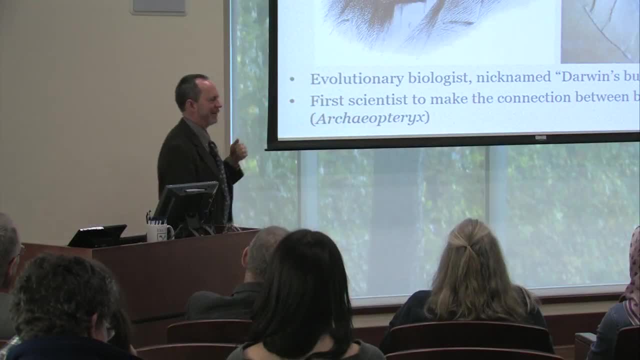 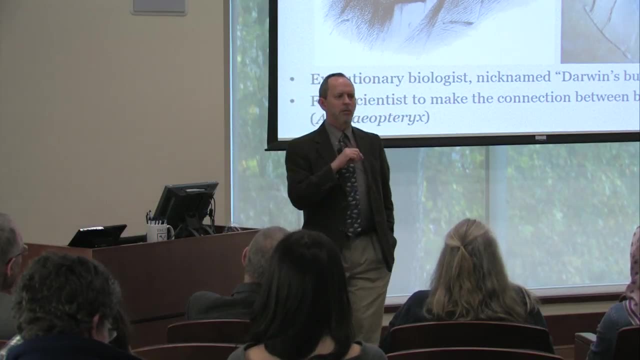 Huxley did. Huxley went out there and fought for him, So he's often nicknamed Darwin's bulldog. A cool thing that Huxley did was with the discovery of that fossil on the right which you can see in the Berlin Museum of Natural History: Archaeopteryx. 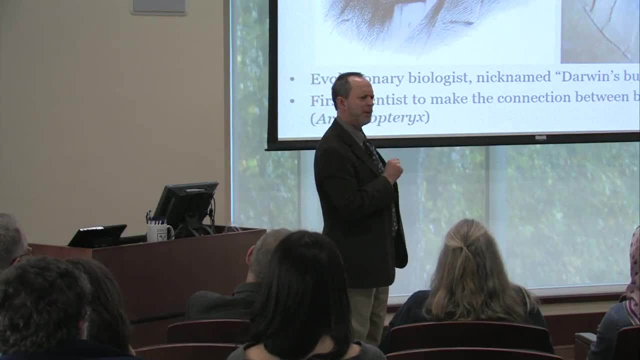 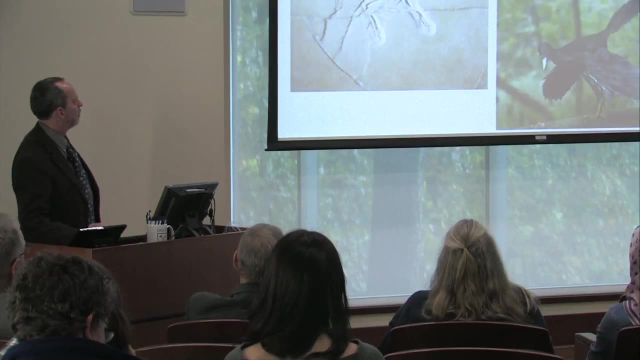 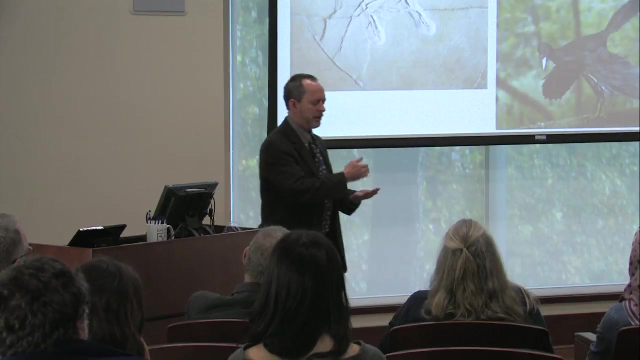 With the discovery of that fossil just a couple of years after Darwin's Origin of Species came out. this was the first fossil in which we're able to link the traits between birds and dinosaurs, And Huxley did it then. It was an idea that really didn't revive until the 1960s. 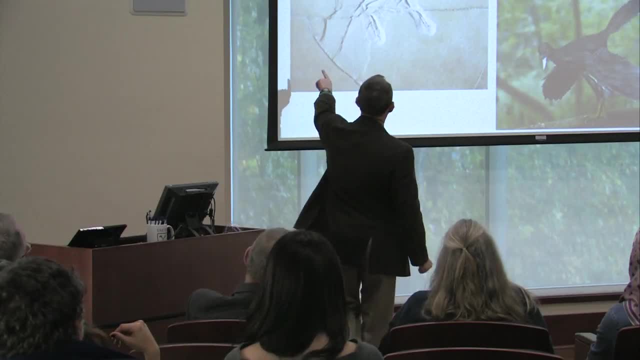 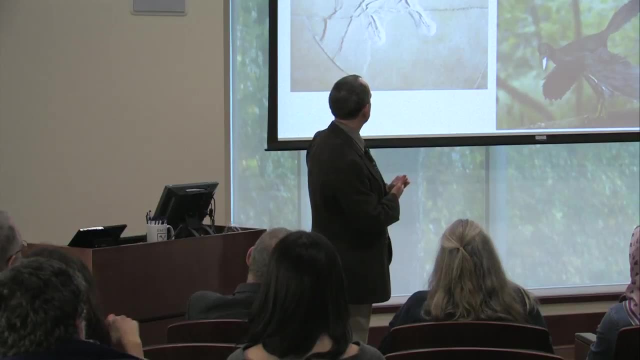 But Huxley, at that time, was able to connect the anatomy of this, which is classified oftentimes as the first bird from 145 million years ago, Jurassic of Germany- And that this bird, though, has all of these dinosaurian traits. 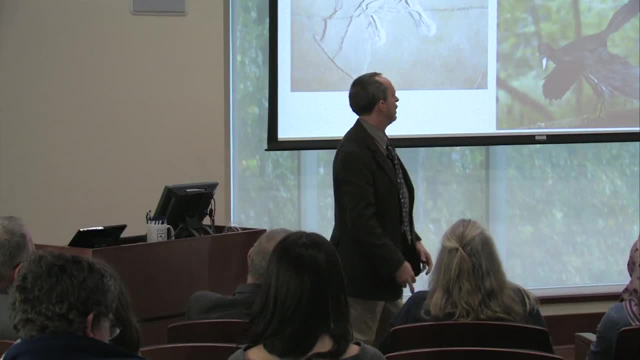 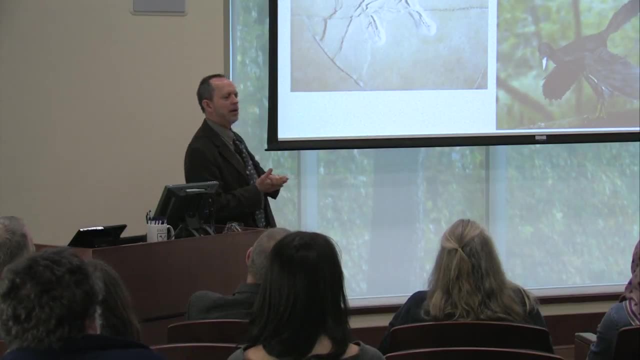 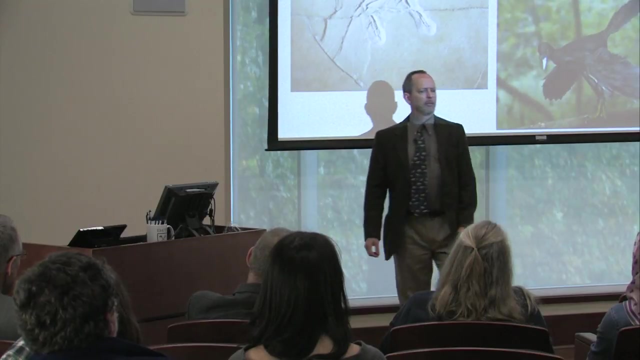 Look at that long bony tail, Look at the teeth, Look at the hands. Those characteristics are more dinosaurian. whereas you look at a modern bird, you see that many of those traits have reduced over time. We now also know the color of Archaeopteryx, based on fossil pigments that are preserved in the feathers. 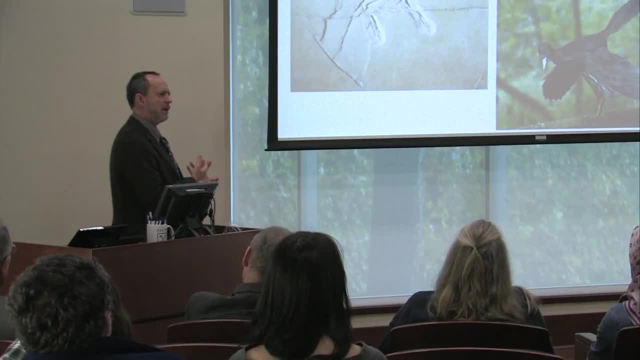 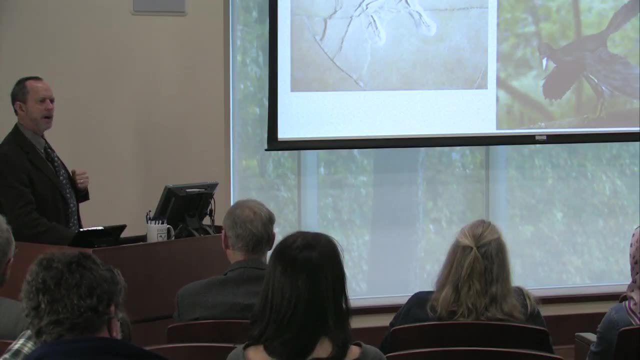 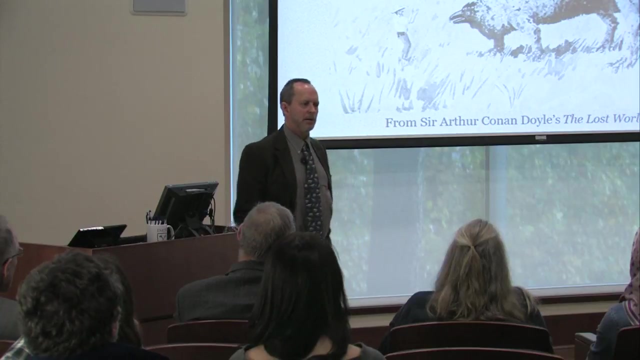 So with Huxley doing this, making this leap, we were able to have an advance in the science of paleontology, and it was helped then by Darwin. along these lines. Now let's get to popular culture again, And here's a pretty neat thing about dinosaurs and other animals from the Mesozoic. 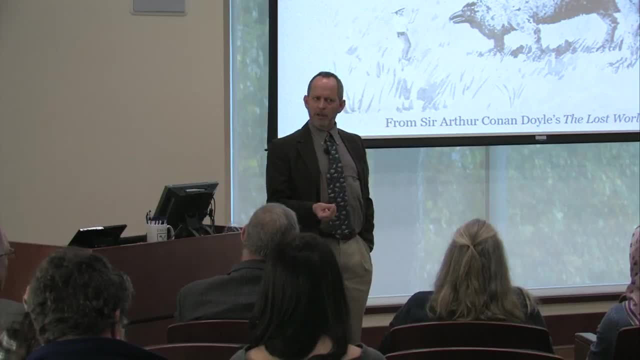 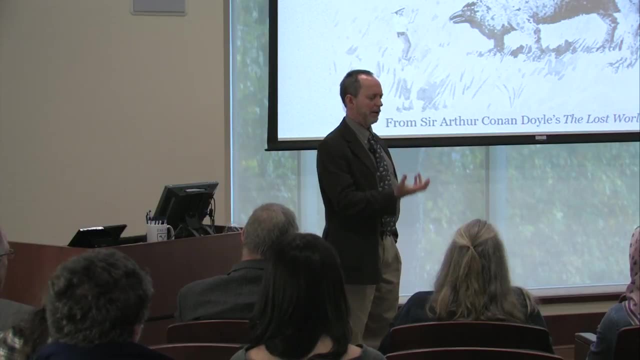 is that as soon as they started being discovered, as soon as they started being named and described scientifically, that's when people in the creative arts took those and acquired them and used them for their fiction And for their art. So I have this illustration from Sir Arthur Conan Doyle's The Lost World. 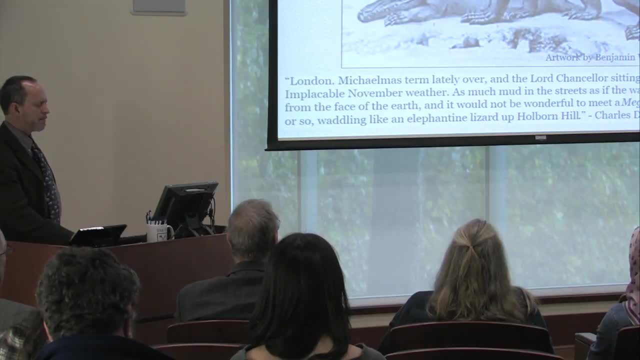 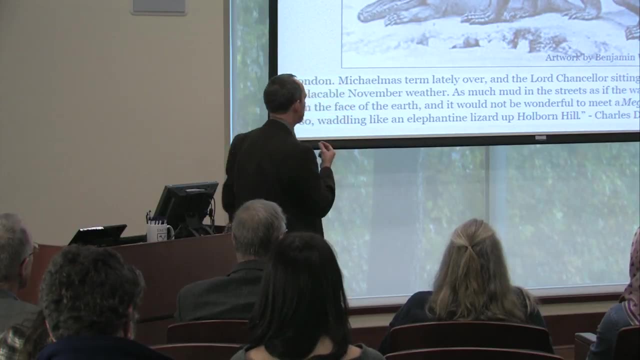 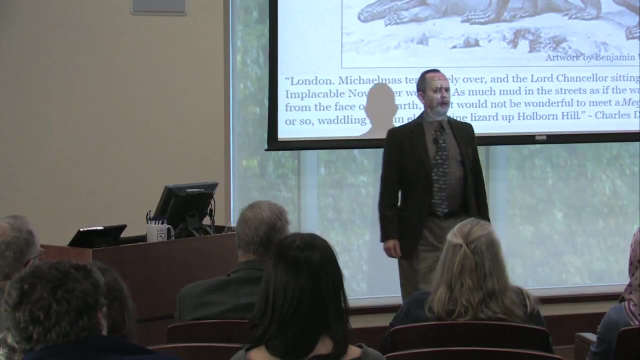 which I'll get to in a bit, But I love this in terms of connecting it to Charles Dickens, That Charles Dickens was one of the first people- he wasn't the first, but one of the first people in 1858 to use a dinosaur as a metaphor. 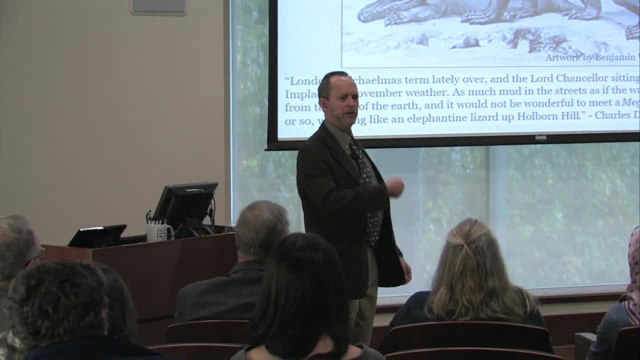 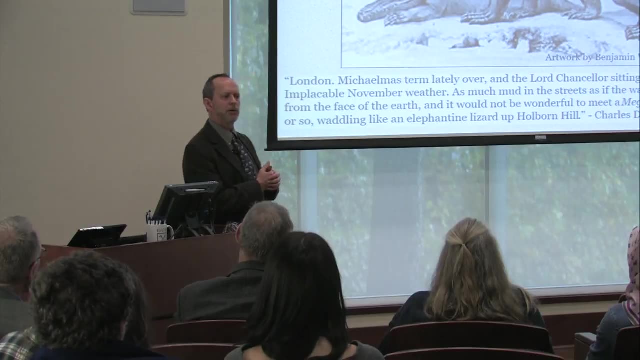 So nowadays we say, oh, dead as a dinosaur, oh, they're dinosaurs, And we use that as a metaphor. we use that as a metaphor in everyday life, But Dickens was one of the first people to use it in literature. And here he's saying: 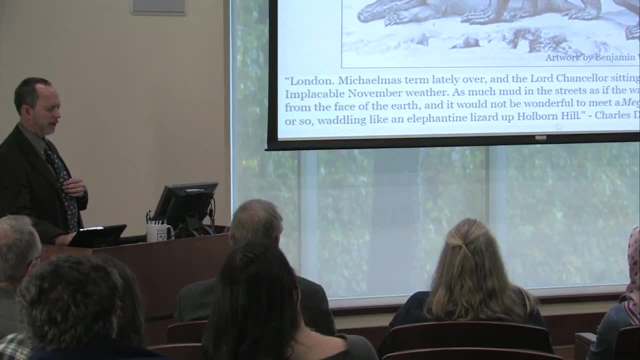 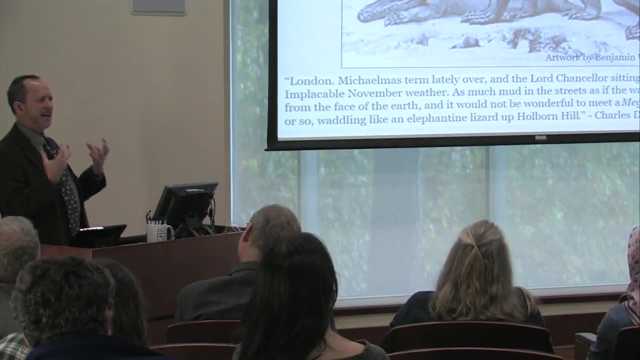 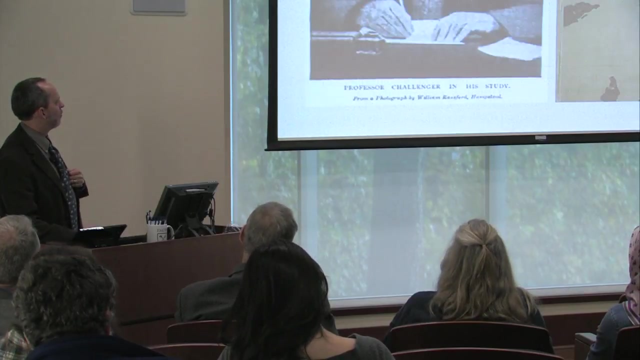 40 feet long, waddling like an elephantine lizard up Holborn Hill. So using that in that context, that gave the readers a vision of something that totally did not exist before or was available as a metaphor in literature. Fast forward just a little bit. 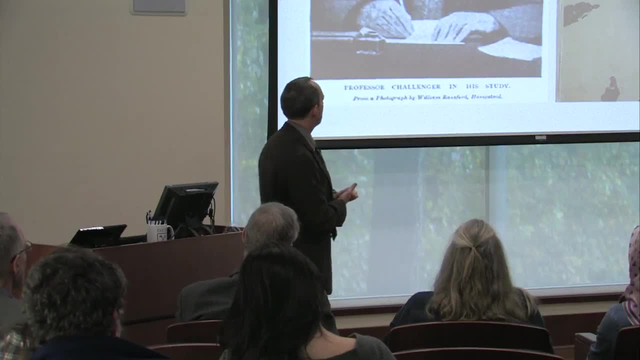 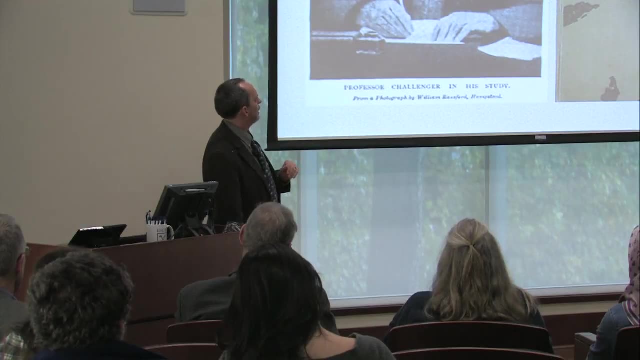 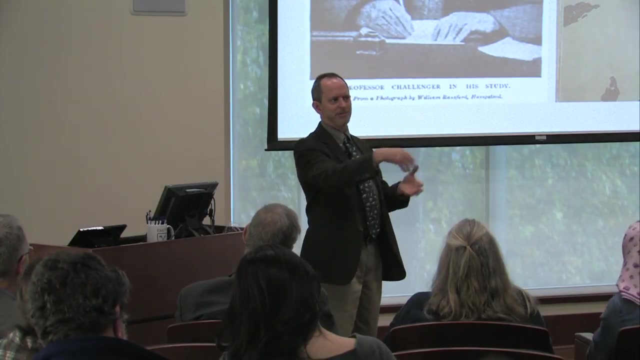 Sir Arthur Conan Doyle is most famous in Sherlock Holmes as the creator of one of the most- yeah, I think, the most famous fictional character- we could argue about that in history. But he also wrote this book, A Lost World, which then Michael Crichton stole the title. 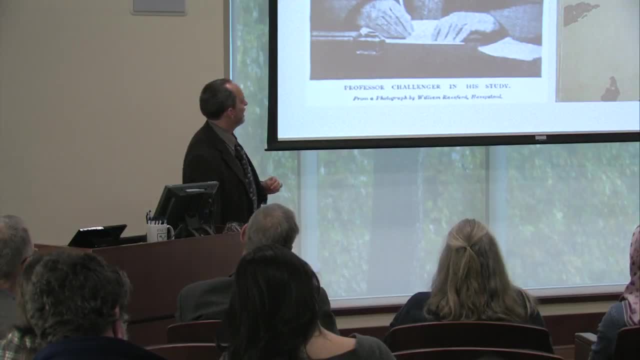 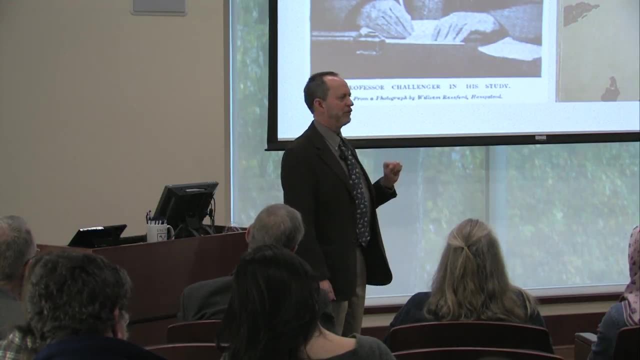 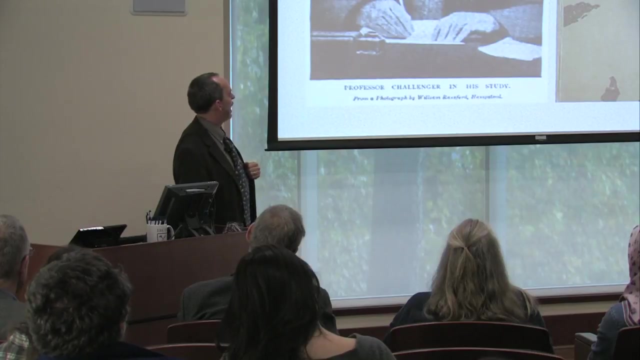 and used it for the sequel to Jurassic Park. This is actually Sir Arthur Conan Doyle cosplaying as his character, Professor Challenger. That is Sir Arthur Conan Doyle underneath the beard and with the professor outfit there. So in this fictional story, there were dinosaurs in South America. 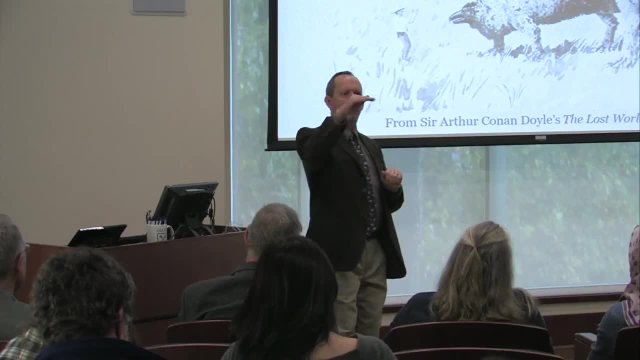 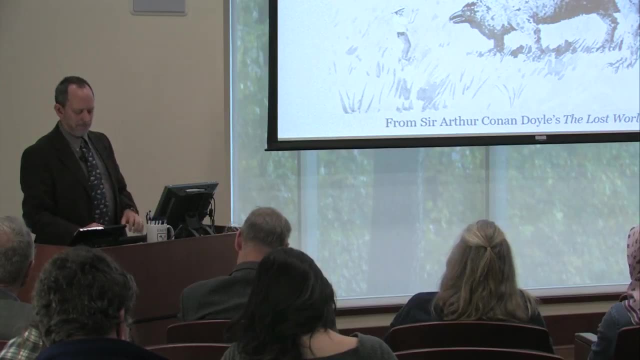 We'll go back here: Dinosaurs in South America, on an isolated plateau- which there actually is an isolated plateau in Venezuela, but there are no dinosaurs there, sadly- And these explorers go in and they document what's there and have grand adventures. 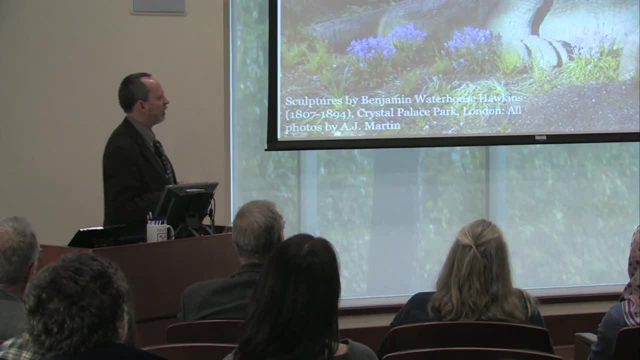 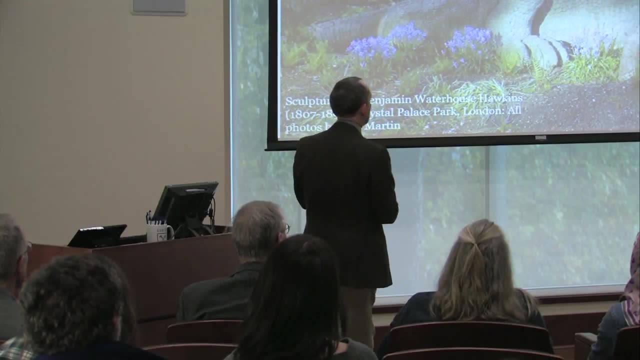 Wonderful book. I'd recommend reading it. That's from 1912.. Artists also started depicting these as sculptures And this was, I think, in the 1860s These were made. you can still see these sculptures. These are in Crystal Palace Park, just south of London. 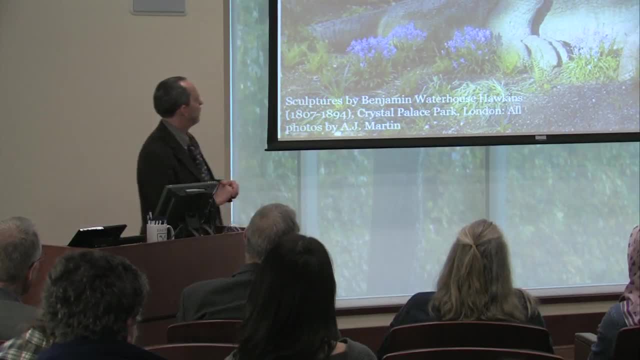 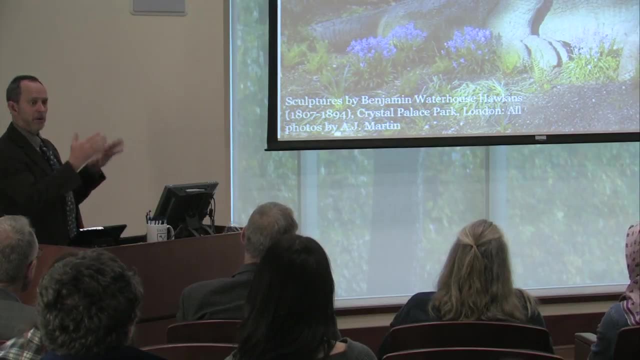 You can take a bus or the rail down there and check them out, And these were built to what was thought to be life size. This is Iguanodon. Think about what you saw previously. Iguanodon as it was thought. 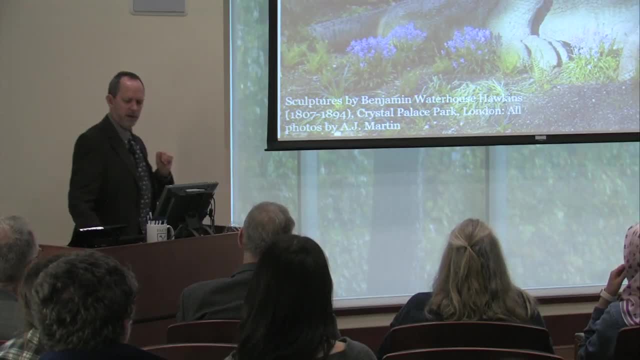 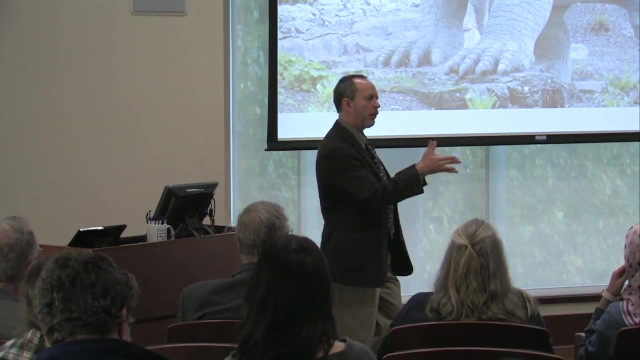 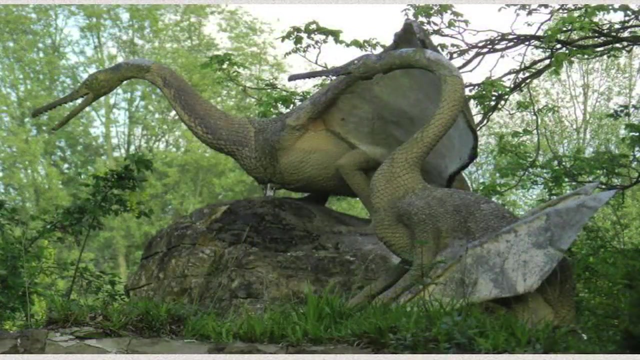 and this was by the artist Benjamin Waterhouse Hawkins who created these, And this was Megalosaurus. Now Megalosaurus, we know later, was more of a two-legged carnivorous dinosaur, but at the time this was made as this gigantic carnivorous, lizard-like animal. 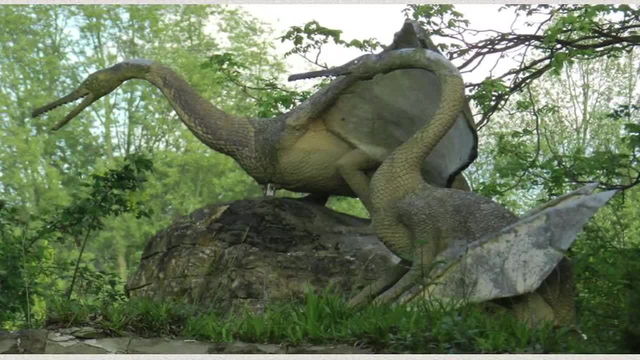 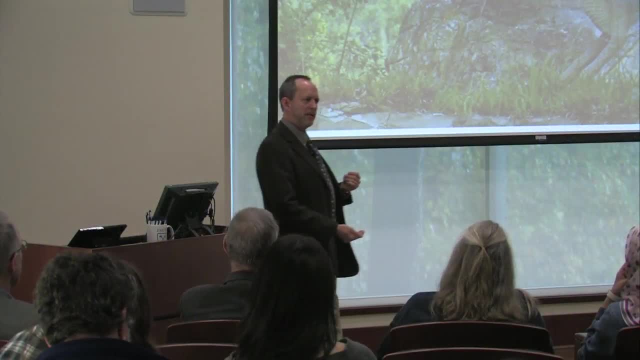 And I don't know where he got the hump from, but there it is. And then pterosaurs: We also have pterosaurs there too, So these are recreations of these animals made at life size by the 1860s. 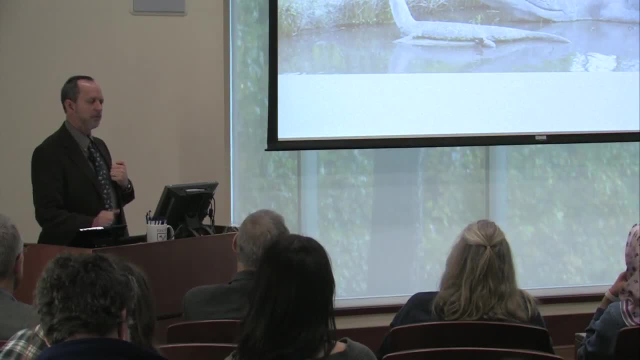 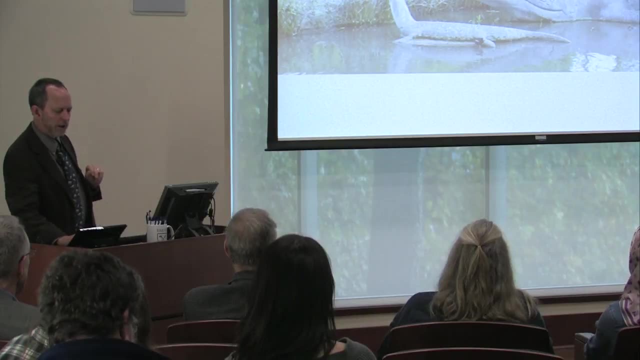 and being put on display in London at the time, so becoming part of the pop culture. And then you recognize plesiosaurs and ichthyosaurs and there's some crocodilian-like animals over here on the right. I know what you've been thinking. 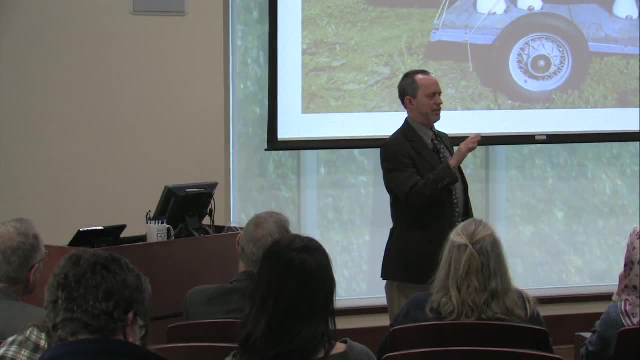 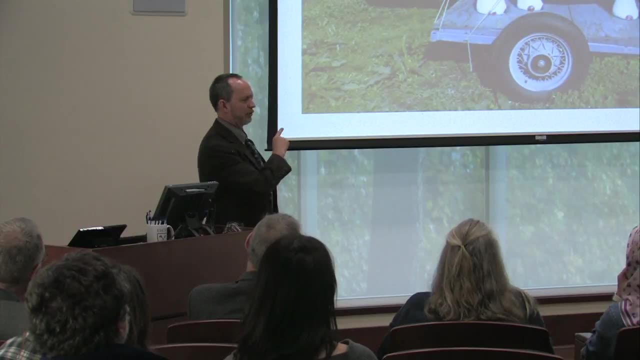 You're like: where are the American dinosaurs? I'm tired of those foreign dinosaurs, I want to see American dinosaurs. Well, you got it. okay, There are a few dinosaurs more American than Stegosaurus. Okay, that's an all-American dinosaur. 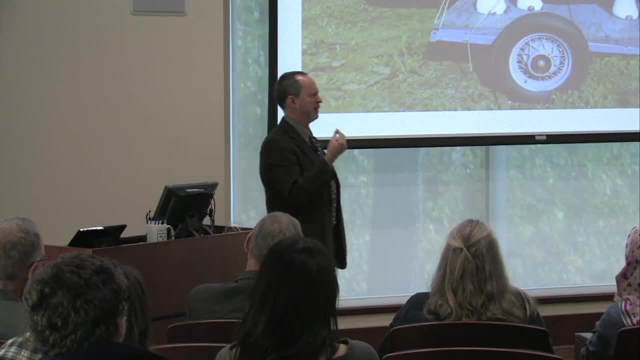 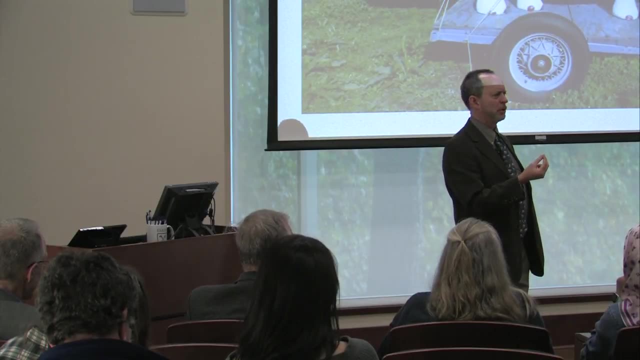 Triceratops is an all-American dinosaur. What's another all-American dinosaur? Just name it The biggest, baddest, fiercest, most American dinosaur ever. Please don't say Coelophysis, No. What's a person hiding inside that? 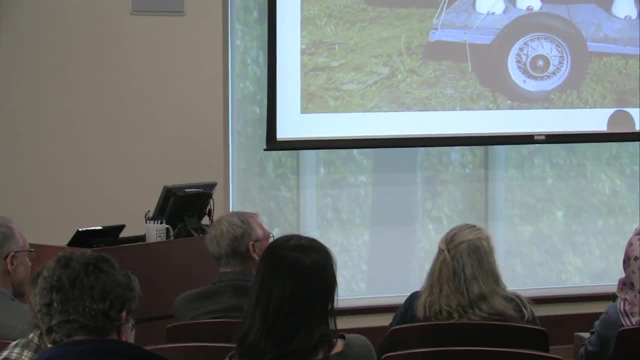 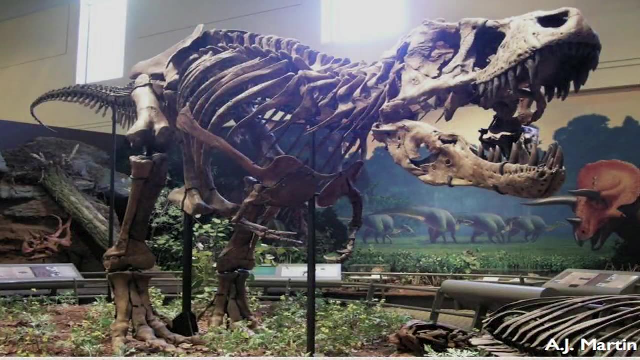 I've seen the x-rays. No, which dinosaur- Tyrannosaurus Rex. Okay, so Tyrannosaurus Rex. this is actually the original specimen. This is the type specimen of Tyrannosaurus Rex. You can see it in Pittsburgh. 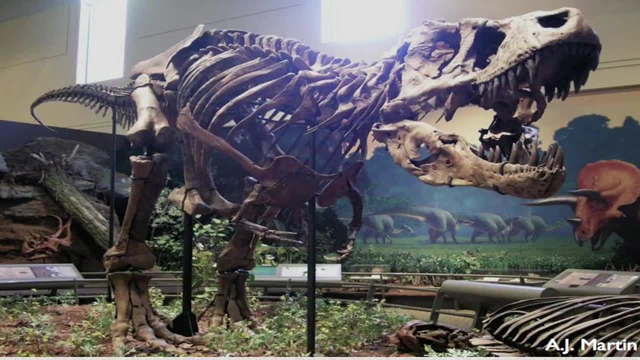 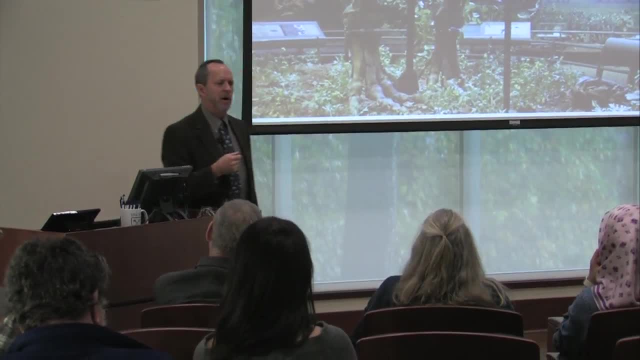 So go to the Carnegie Museum of Natural History. Here's the mounted specimen there. This was probably a seven- to eight-ton carnivore, and it is arguably the most famous fossil in the world, although I like to argue that, because I think Archaeopteryx is actually more famous. 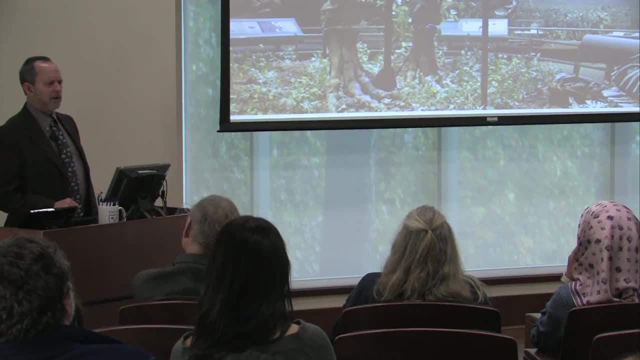 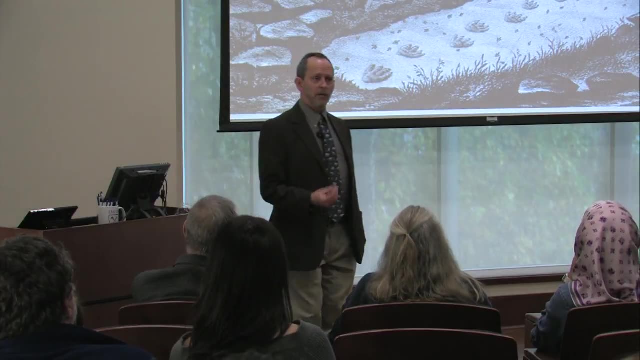 has the link between dinosaurs and birds. So this is an American dinosaur. But here's a pretty neat thing about dinosaurs in the United States is that the first fossils of dinosaurs in the United States were not bones. The first ones found were tracks. 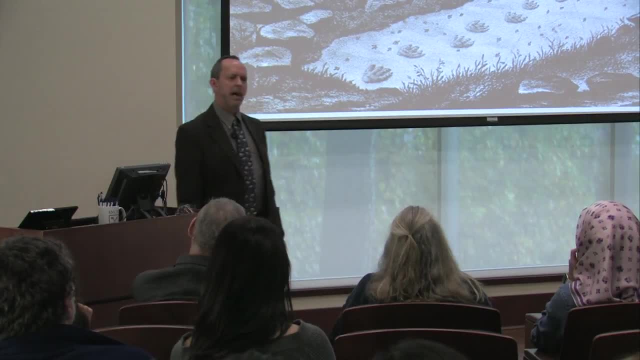 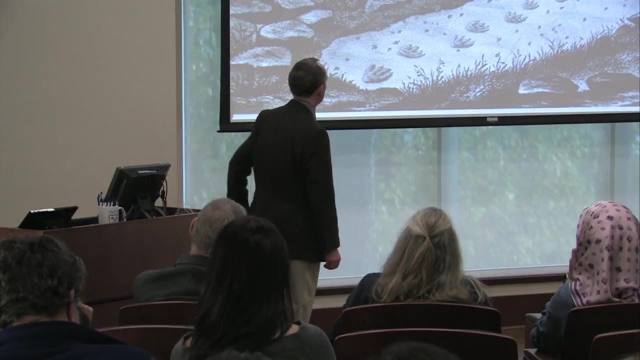 This was in 1802.. There was a schoolboy in South Hadley, Massachusetts, in the Connecticut River Valley, fairly close to Amherst. So if you're from that area, you know that area well And look at all the dinosaur tracks there in the rock. 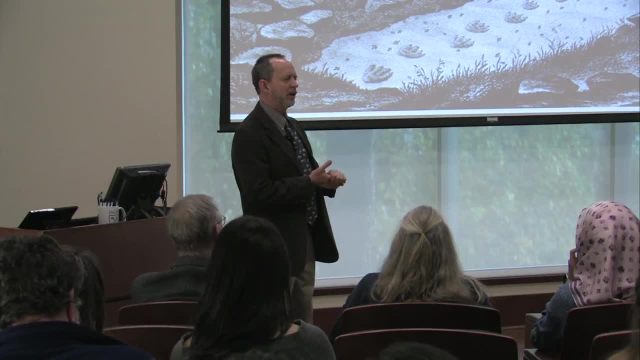 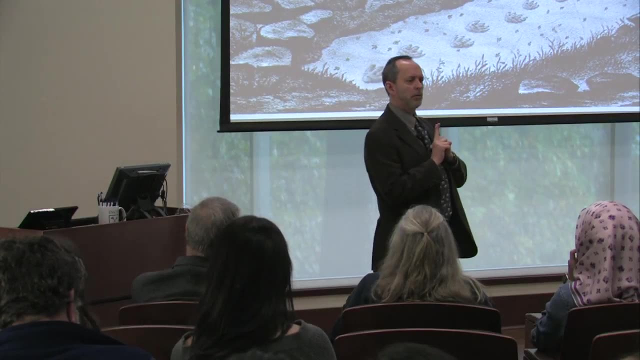 1802,. he found these tracks, He reported them. Some of the local professors they documented them. They had no idea what made these Remember. the name dinosaur didn't exist until Richard Owen came up with it in 1842.. 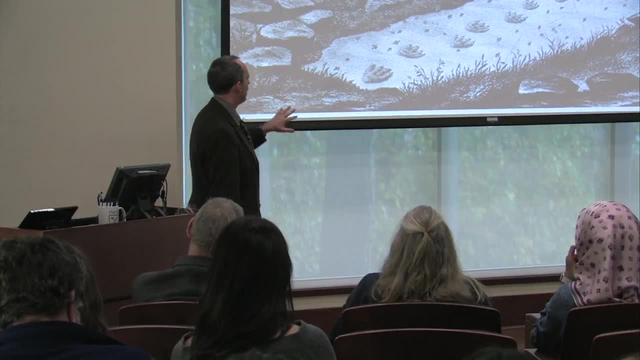 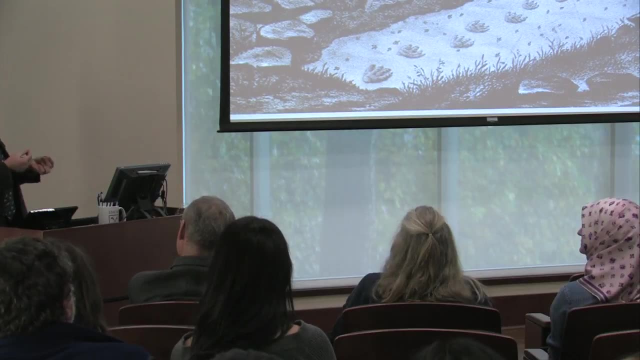 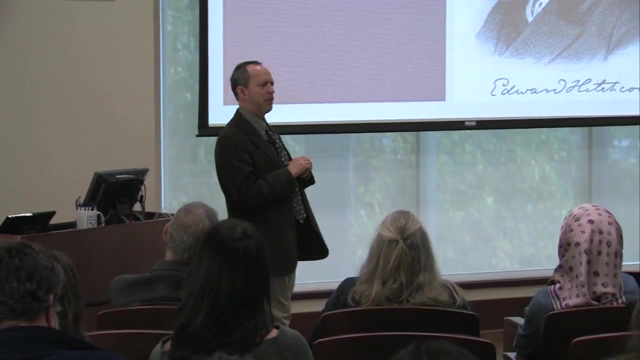 So there was a 40-year gap between the discovery of these tracks in New England and then the name dinosaur. So there was not a connection between these tracks and the bones that were being found elsewhere. This is the third great book I want to point out. 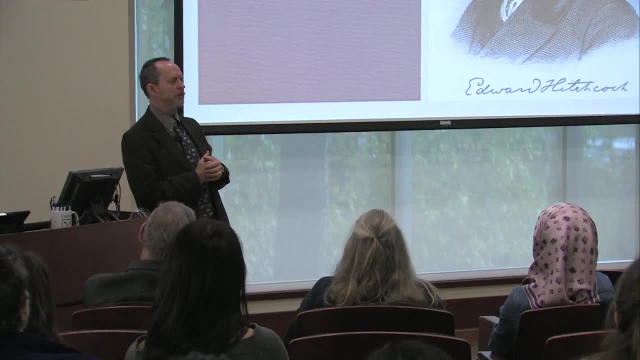 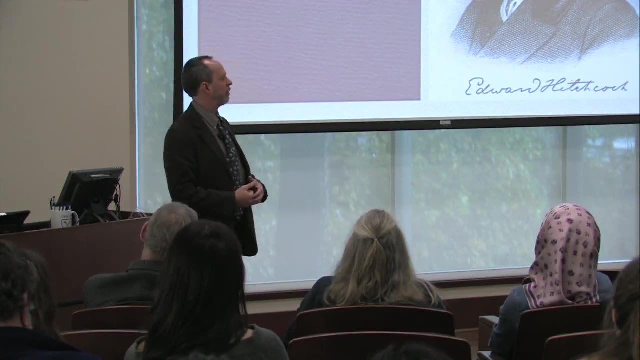 and it's one that ordinarily a lot of people might not include in such a list, But I include it because it started connecting the much bigger fossil record of dinosaurs from tracks to their bones, Because if you think about it, how many bones do you have in your body? 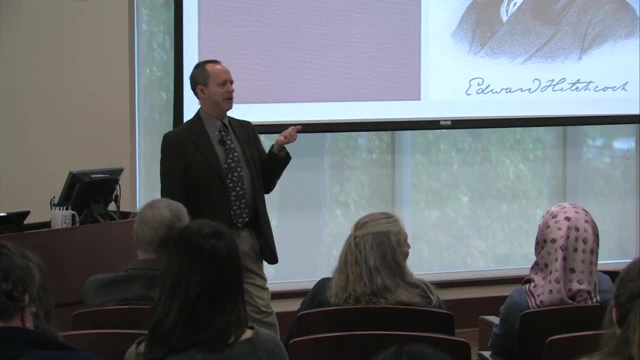 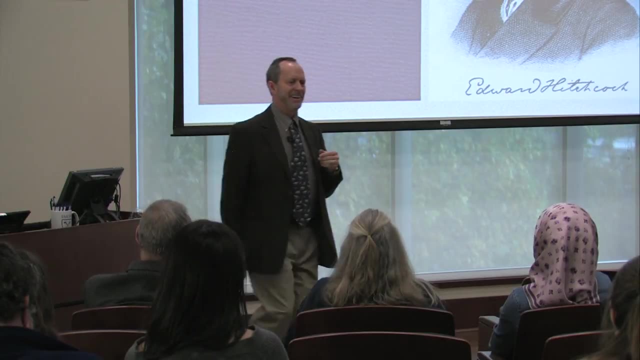 This is probably on the MCATs, so you all should know this. How many bones are in your body You're going to do? well? I don't want you operating on me. No, it's about 200.. Around in there. 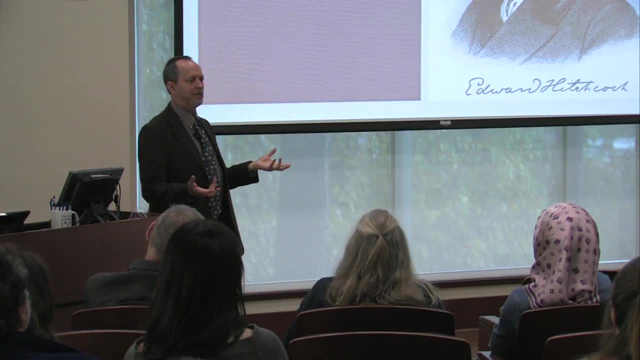 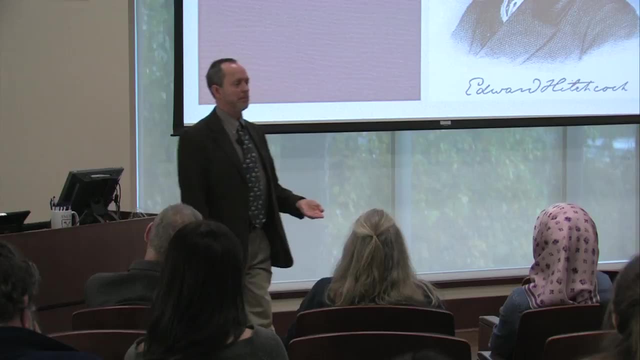 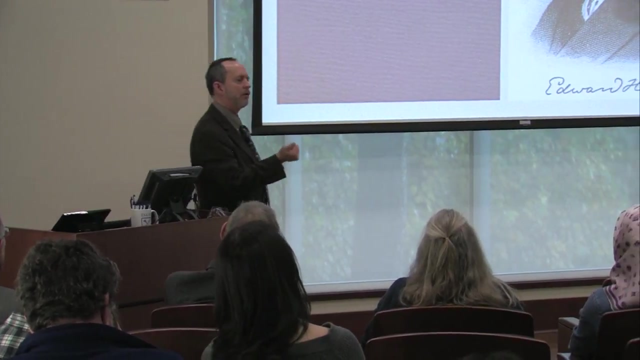 But about 200 bones in a human body, actually about the same, in a lot of dinosaurs about 200.. Then think of tens of thousands of footsteps it took during its lifetime. So a fossil record for tracks is actually better than bones. So Edward Hitchcock, who is the founder of Amherst College, 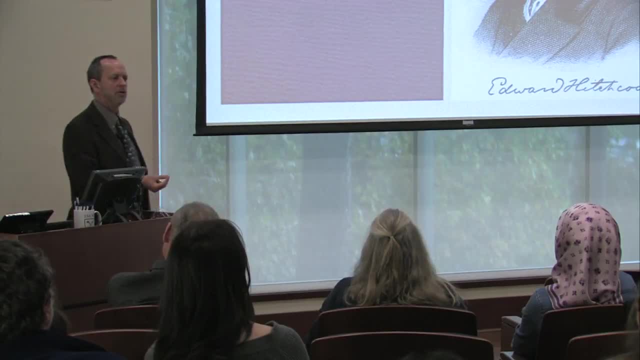 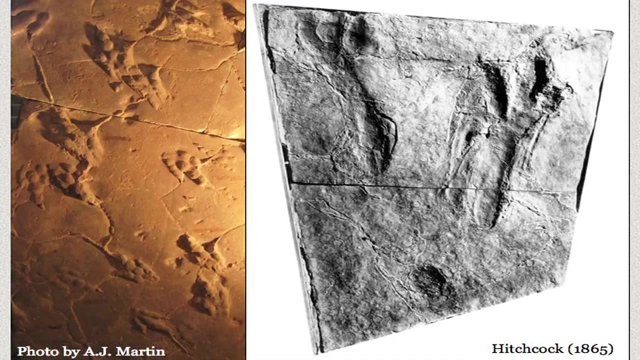 and was a clergyman and was a paleontologist, studied these in earnest and did this very thick book reporting on these trace fossils, These traces of dinosaurs from that area, from about 200 million years ago, from the early Jurassic. This was actually a pavement stone. 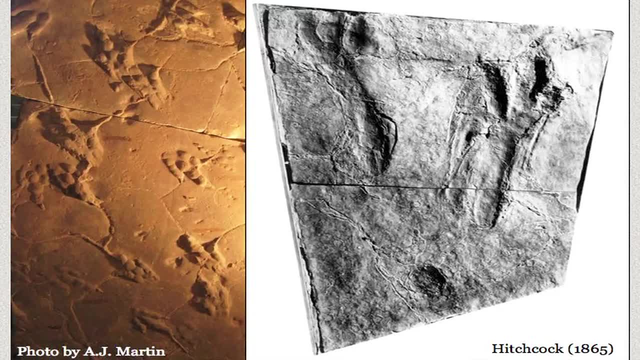 It was a pavement in one of the towns- I can't remember if it was in Amherst or South Hadley- And then he had it put in the museum because of these theropod, these carnivorous dinosaur tracks that were all over the slab. 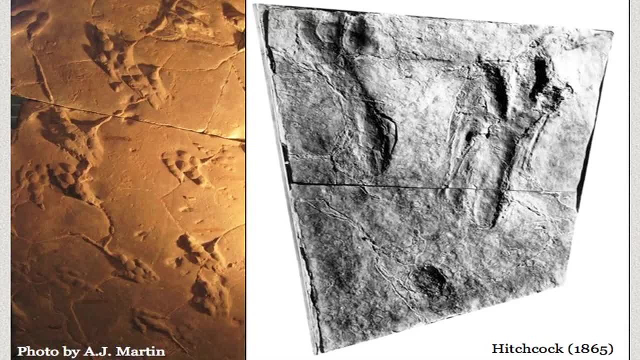 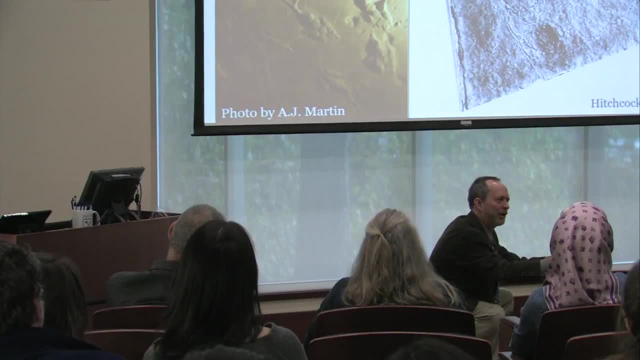 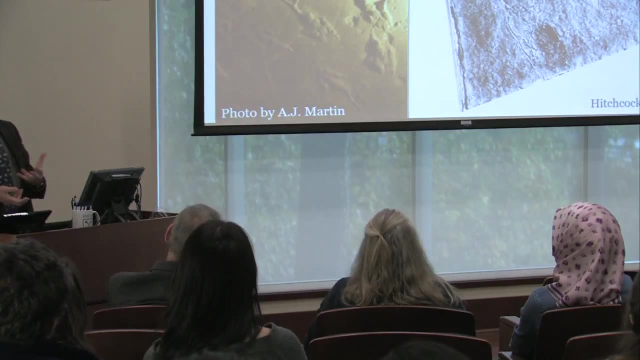 The one on the right is a sitting dinosaur trace where a dinosaur sat down on a lake shore, And I will imitate it now. When it sat down on a lake shore about 190 million years ago and left those impressions, His photograph. this is one of the first uses of photographs. 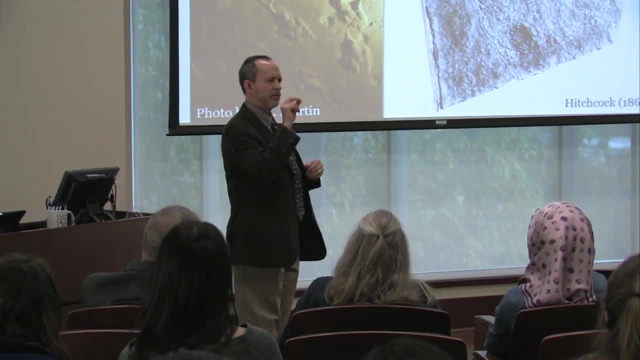 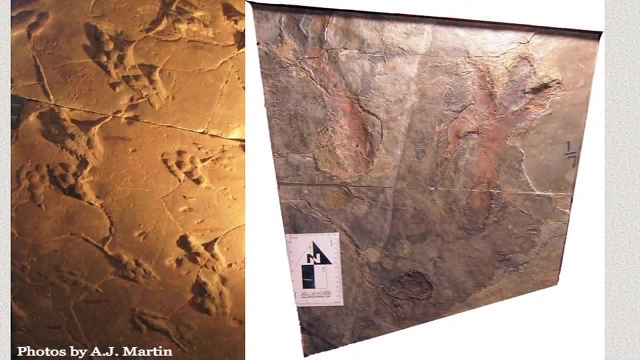 in scientific illustration was of these dinosaur tracks, So that's an actual photograph from that. That's my photograph in 2004,, taken almost 150 years later, of the same specimen, the sitting dinosaur Here's a neat thing- was Hitchcock and Darwin wrote to one another. 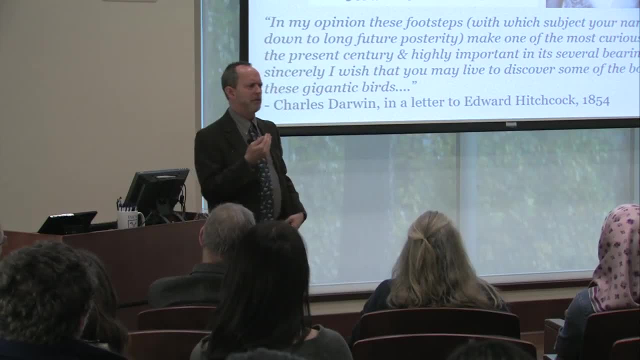 And a lot of people I talk to are surprised at that. But if you read anything about Darwin, he wrote letters all the time because people wrote him letters And he wrote them back. So there's this. you can find it online, this huge collection of Darwin's letters. 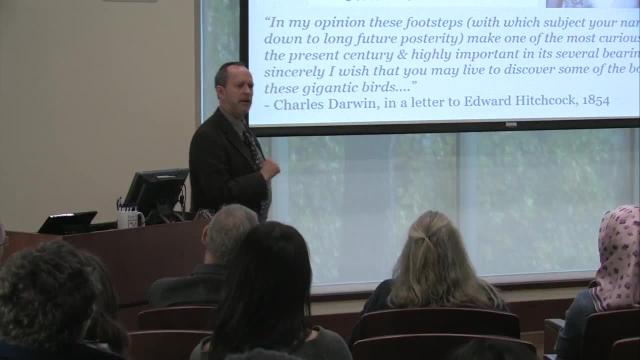 This online you can look up where he corresponded with Edward Hitchcock And Hitchcock told him: I want some tracks And Darwin was like cool. So I may be paraphrasing a bit, But it was an exchange like that. 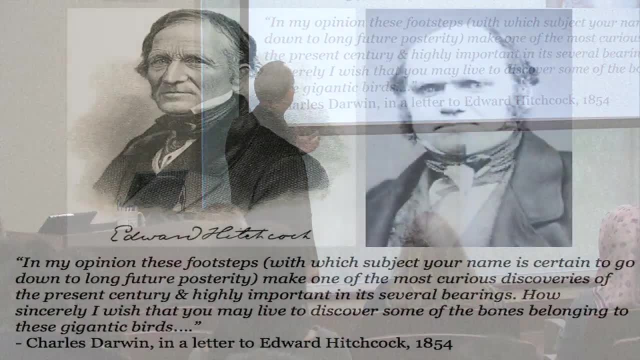 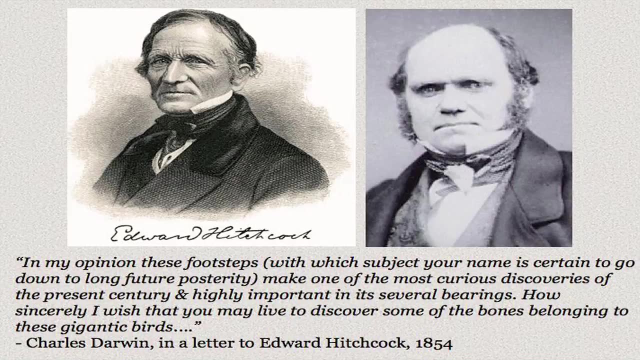 in that Charles Darwin was reacting to this. in my opinion, these footsteps- footsteps being the tracks with which subject your name- is certain to go down in the long future: prosperity. Yes, that is correct. Hitchcock is still famous for these discoveries. 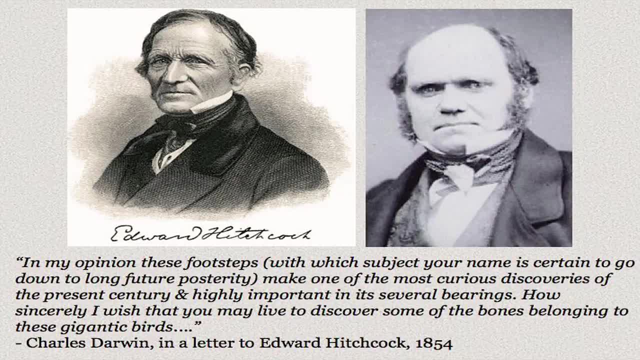 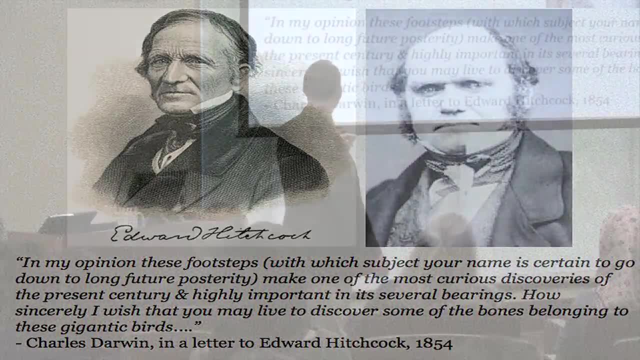 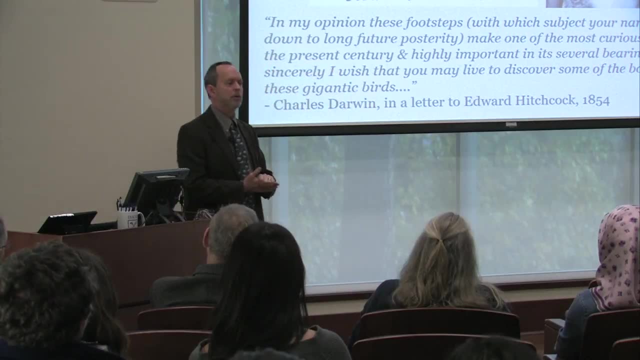 Make one of the most curious discoveries of the present century. Yes, true, still true. Highly important in several bearings. how sincerely I wish you may discover some of the bones belonging to these gigantic birds Birds. What's with the birds? Hitchcock believed these all belonged to gigantic birds. 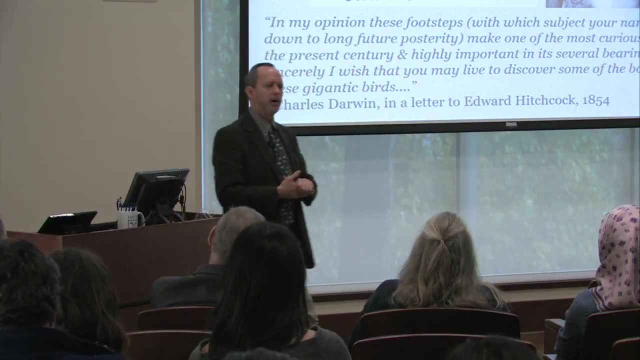 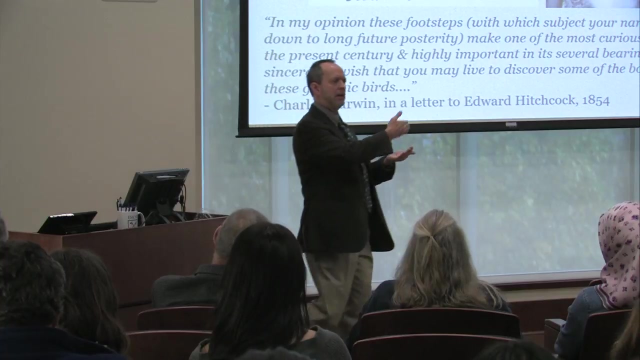 And throughout this book he relates them to birds, and very odd birds that also had tails and also had these other traits that we didn't see in modern birds. So he was very perplexed by this. but later on- and think about Huxley connecting birds to dinosaurs- 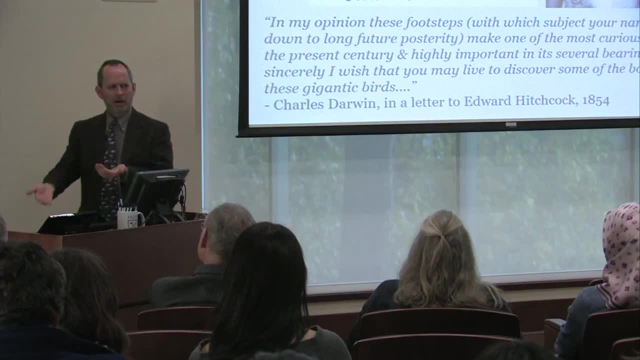 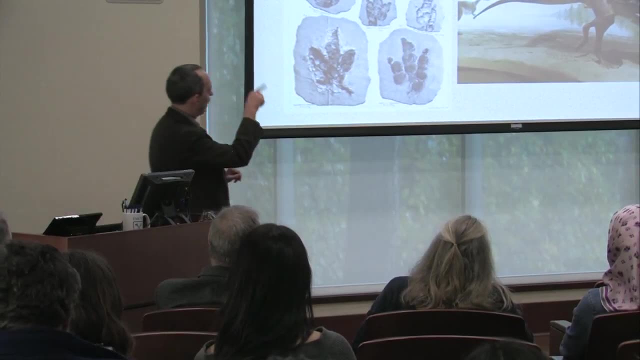 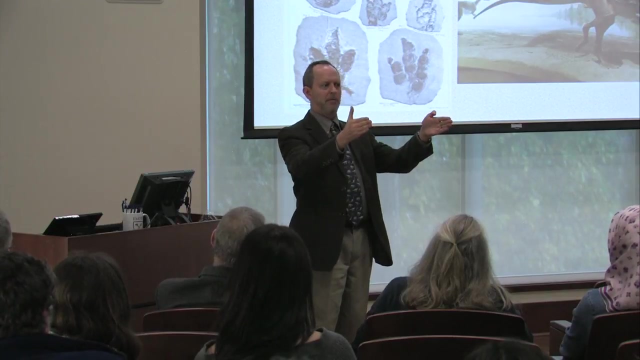 that Hitchcock, independently, was actually connecting the traits of these tracks to what we see with modern birds. So this excerpt where he's talking about how strange his appearance must have been: it had a foot 16 inches long, so think about feet that big. 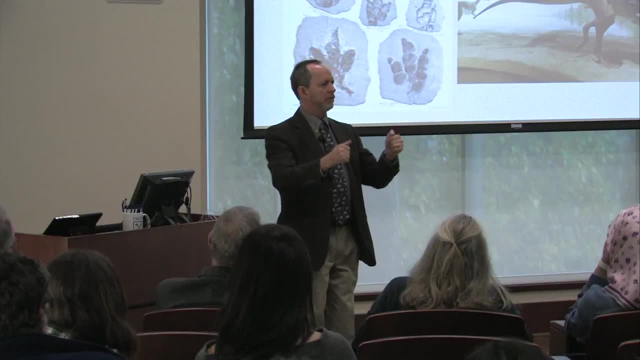 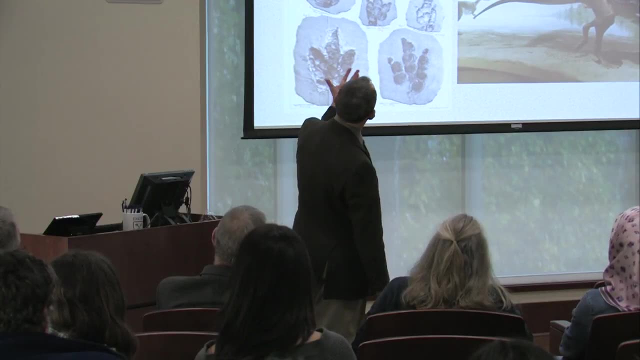 and some of these tracks were about like that, So these were from very big animals. They're three-toed tracks. They have claws at the end, So these were from very big animals, So they look very much like bird tracks. It has a huge body. 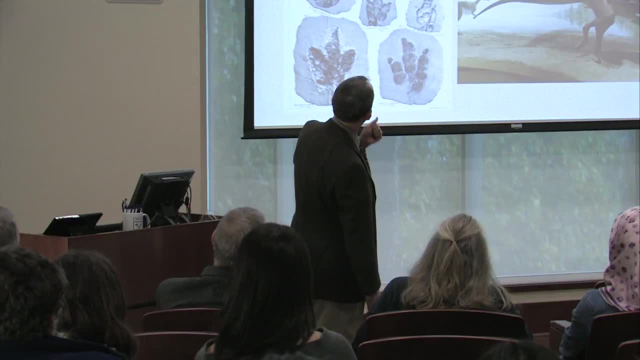 and then see that it has a fourth toe. so that's like a bird that has like a perching toe And then it's a biped. but it also- some of these- had a little tail trace behind them, like what birds have a tail behind them too? 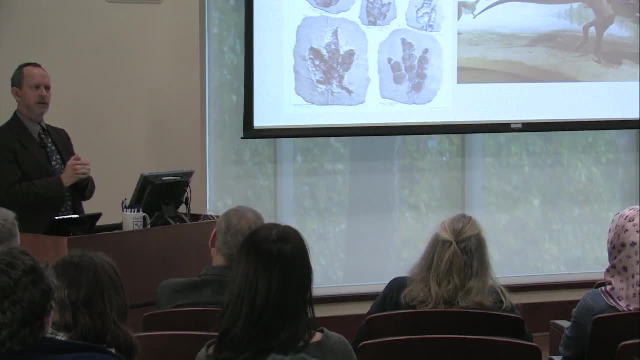 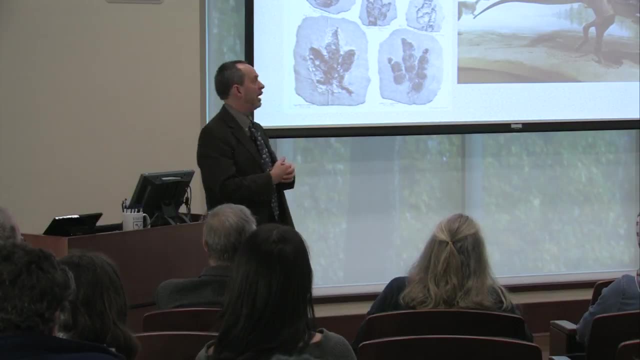 So you can tell from this paragraph, he's very confused. He's not quite sure what these animals look like. But it wasn't until later on we were able to put together the bones with the tracks and then realize, ah, that's what made these. 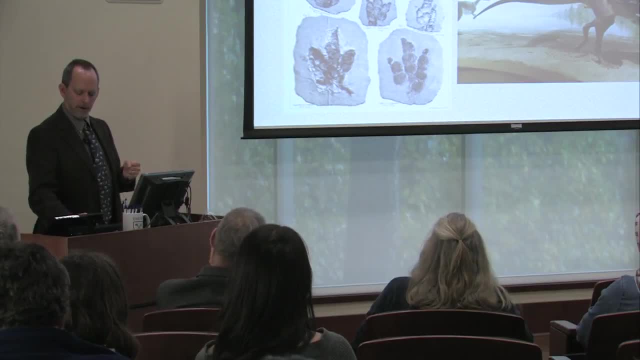 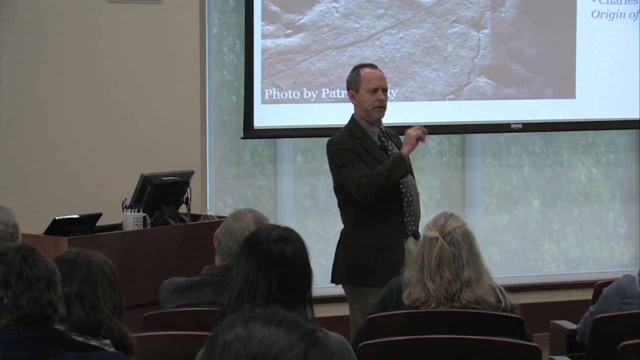 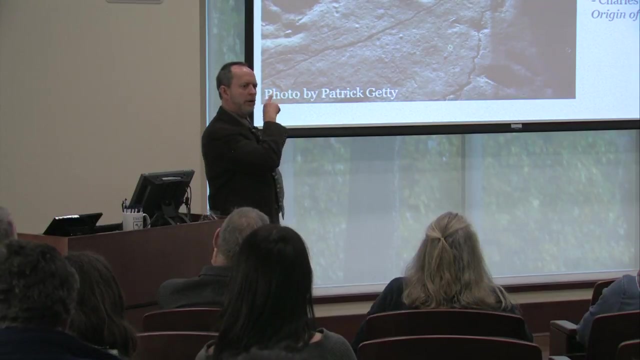 and now we have a more complete fossil record of these animals And you can go to Rocky Hill, Connecticut, and there's a little dinosaur state park that you can go to a building that has these tracks down there Now to get down and look at them, like I did, very dramatically. 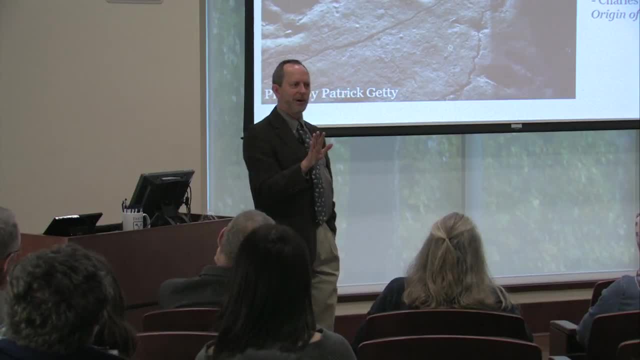 you do have to get permission to do that, so don't just do it. But there are about 500 tracks exposed on that surface, just within a relatively small building. All throughout the Connecticut River Valley, this is actually one of the world's most famous sites for dinosaur tracks. 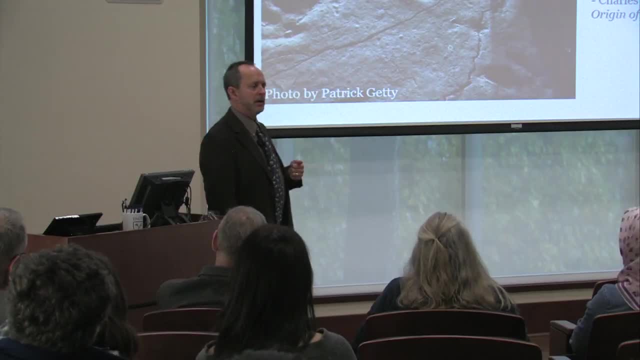 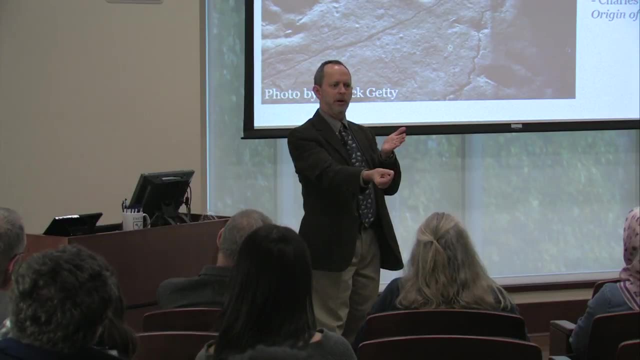 and Amherst College has one of the best dinosaur track collections in the world. So I love what Darwin then took from that. what he learned from Hitchcock he then incorporated into Origin of the Species, He said, had it not been for the rare accident of the preservation of footsteps, 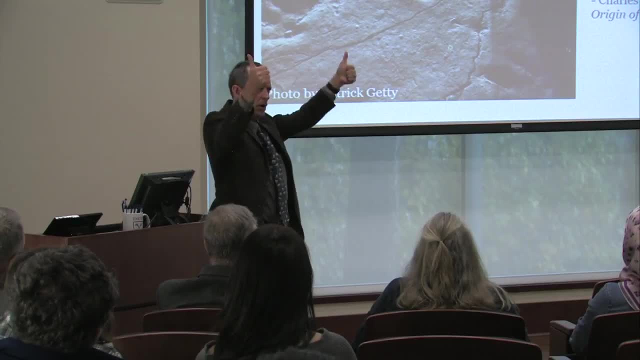 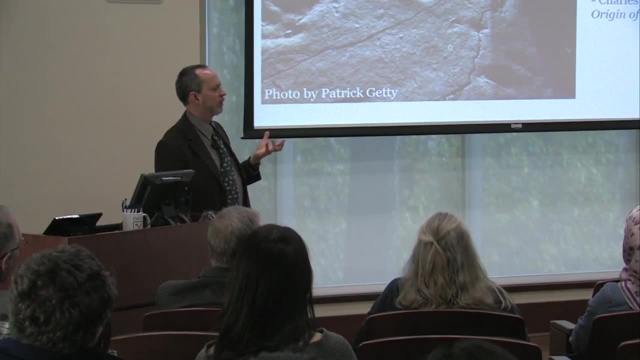 in the new red sandstone of the United States. yeah, okay, who would have ventured to suppose that no less than at least 30 kinds of bird-like animals, some of gigantic sizes, existed during that period? So Darwin at that time then was connecting what we had with trace fossils? 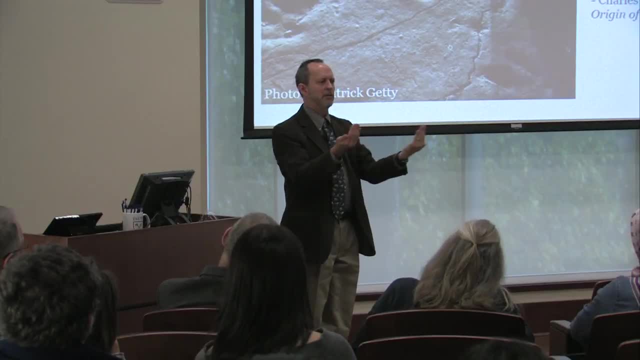 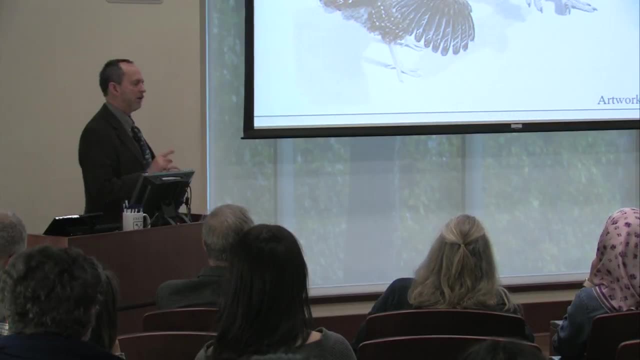 body fossils and showing these give us a complimentary record of the ancient life of the Mesozoic era. Now we know birds are dinosaurs, So when you see that you're going to go home for Thanksgiving, you're going to have turkey, and what did dinosaur taste like? 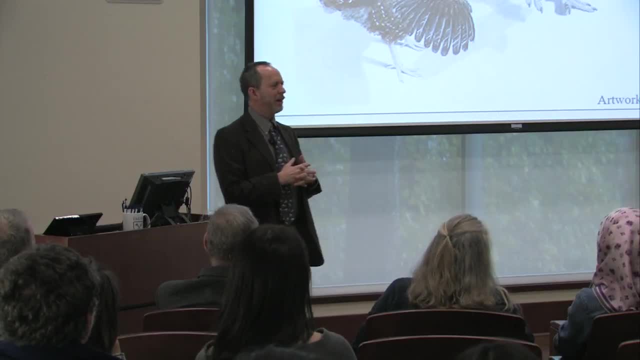 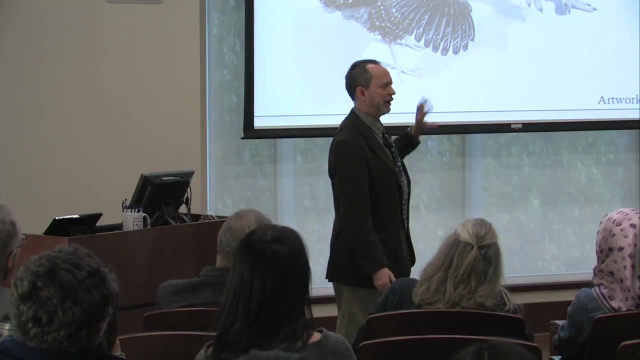 Chicken Turkey. Okay, so you're going to be eating a dinosaur for Thanksgiving? Think about that. And now you will see artistic reconstructions. This is a big change in how dinosaurs are depicted. Dinosaurs are being depicted theropod. 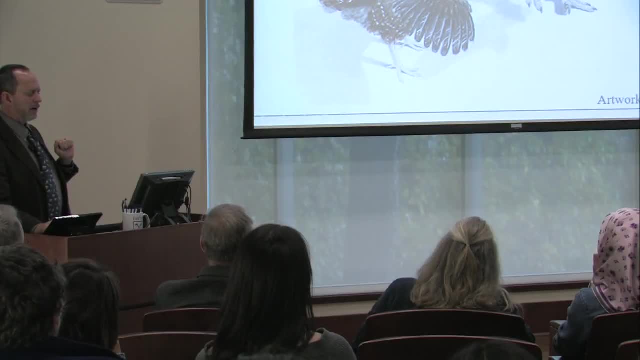 carnivorous dinosaurs in particular are being depicted with feathers, So you recognize this dinosaur right? Yes, that's a rooster. This is actually a Cretaceous bird. This is a Cretaceous bird from China, So you can't see it. 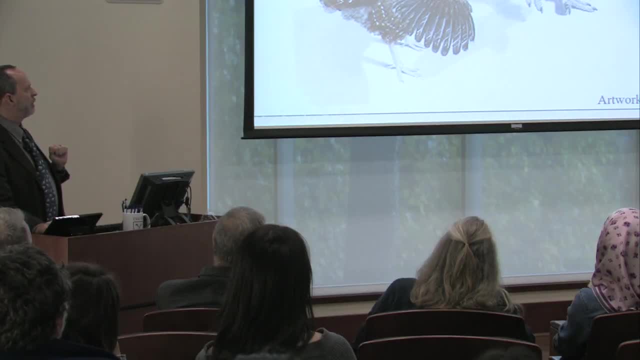 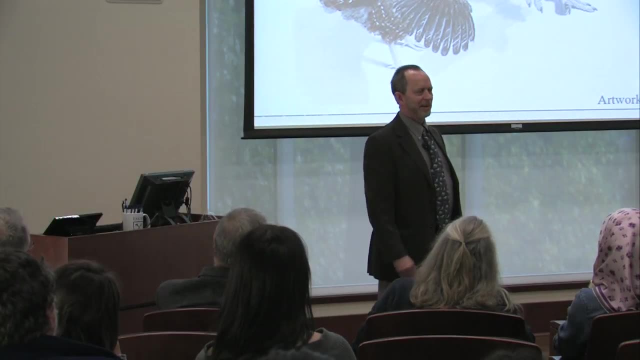 but it has a bony tail going all the way down that way and it has teeth in there too. This is Velociraptor. Yes, Spielberg got it wrong. okay, Because Spielberg had the Velociraptor like that, because he's like. 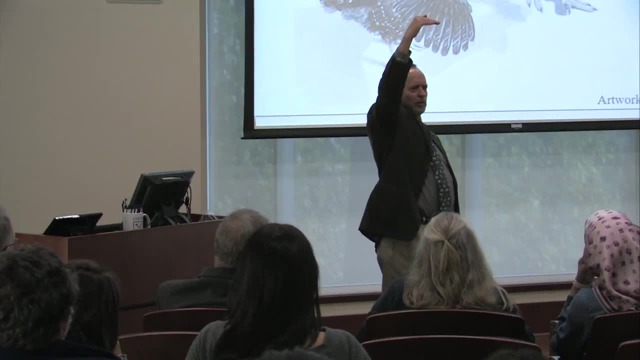 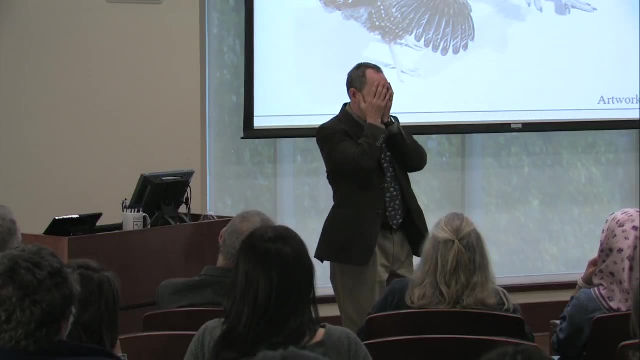 oh, the real Velociraptor. not scary enough? Okay, let's make it twice as big. And they're naked. I know it's kind of embarrassing for me as a paleontologist to watch Jurassic Park. I'm like, oh, they don't have feathers. 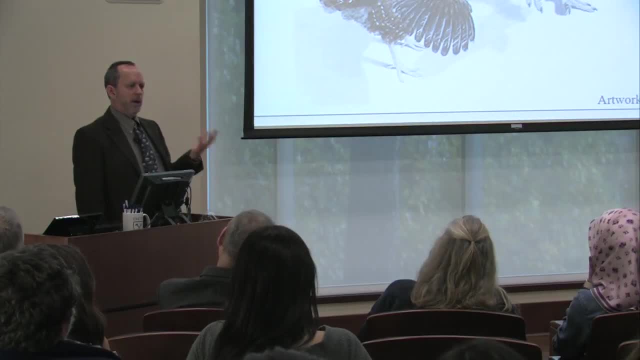 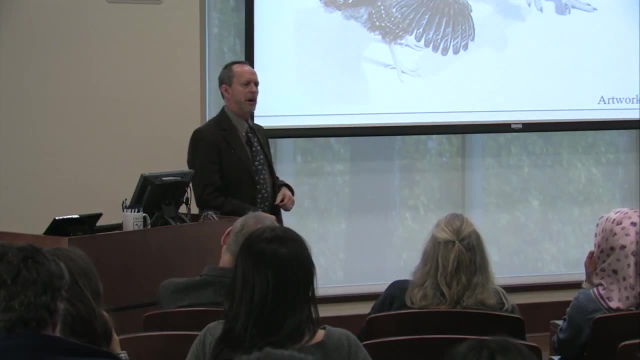 But now we know that Velociraptor had feathers. We can actually see the feather insertion points on the ulna and we can see other places on the body that it definitely had feathers. We have more than 40 species of feathered dinosaurs. 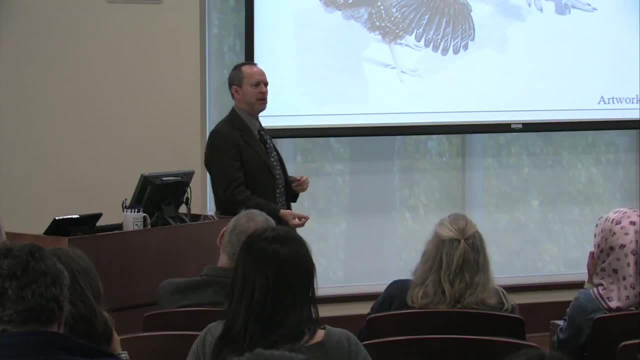 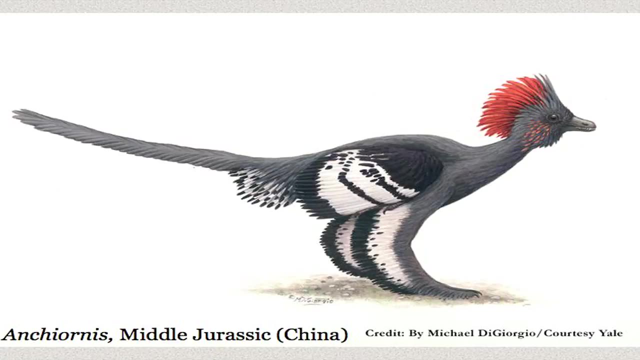 that have come out of China, and we have several species from North America that have been found in recent years too. We even know the colors of some of these dinosaurs. now, too. This is a Middle Jurassic non-avian, not a bird non-avian dinosaur that we actually have. 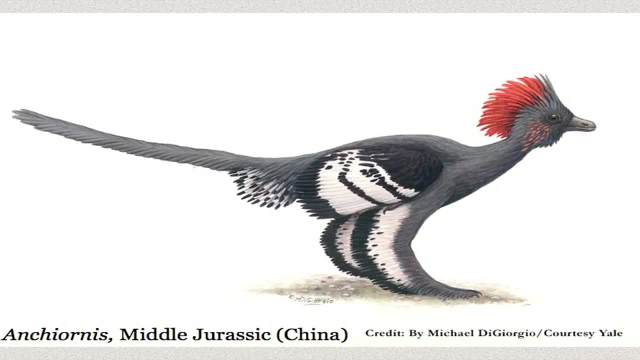 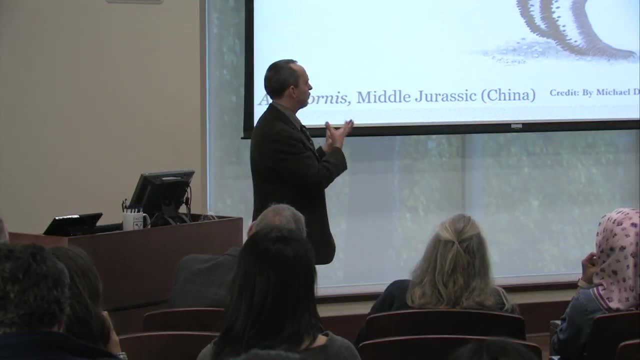 not only the feathers, but there are these pigments that are preserved in the feathers that structurally relate to colors we have in feathers today. So artists working with the paleontologists are actually able to reconstruct the colors. This one had black and white banding. 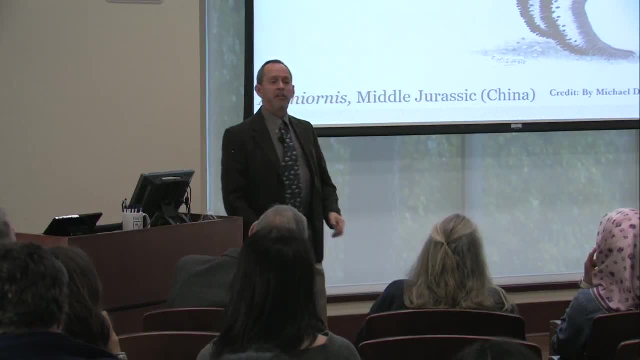 and also had red on the head. Some of the feathers were iridescent too. So if you look at a grackle or some other birds that have iridescent black feathers, we can tell that by looking at the pigments, these fossil pigments that are in the feathers. 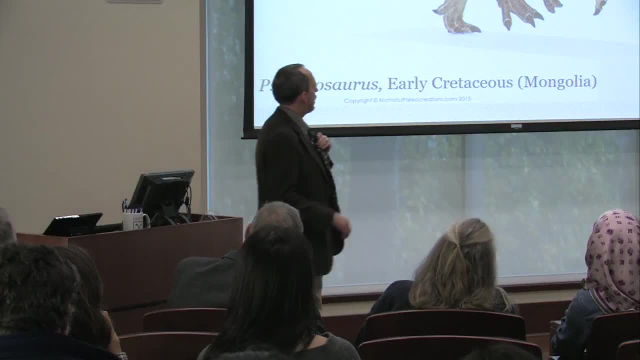 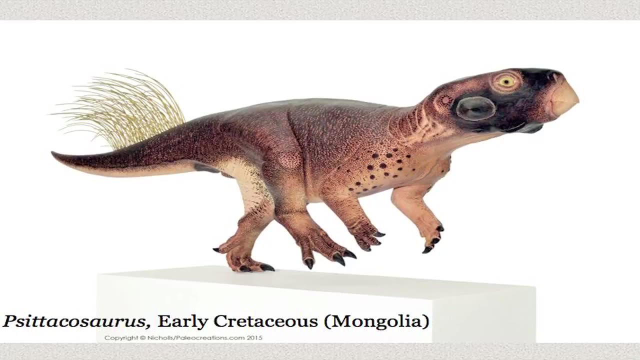 This is not a bird. This is not related to birds necessarily. This is more of an ornithopod dinosaur. but we also have feathered- or I mean color reconstructions, even without feathers. This one was just also for some of those pigments. 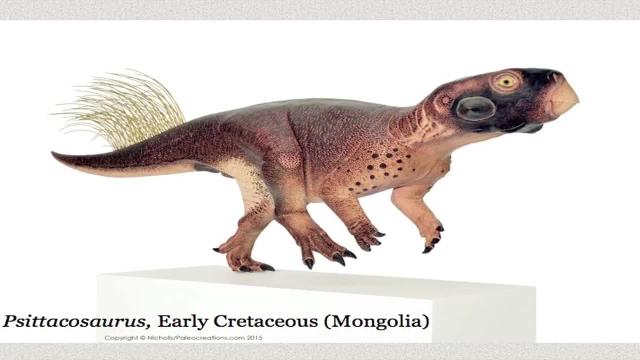 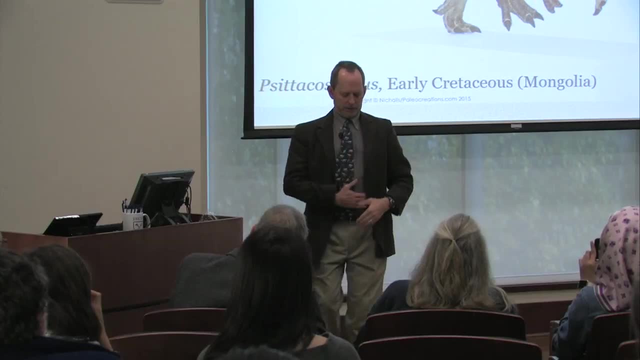 and then the artists, working with the scientists, were able to reconstruct the colors. The neat thing about this animal is that it is white, more white on the back, on the bottom and then darker colored on the back, which is a form of camouflage. 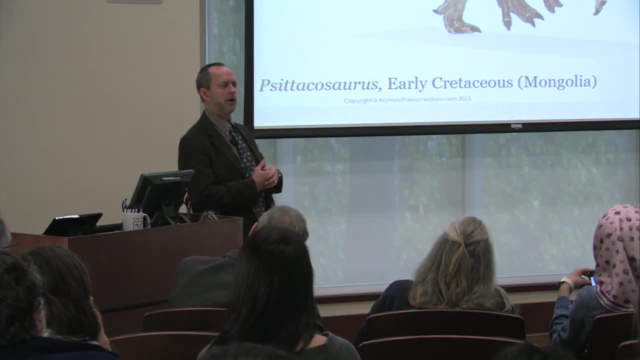 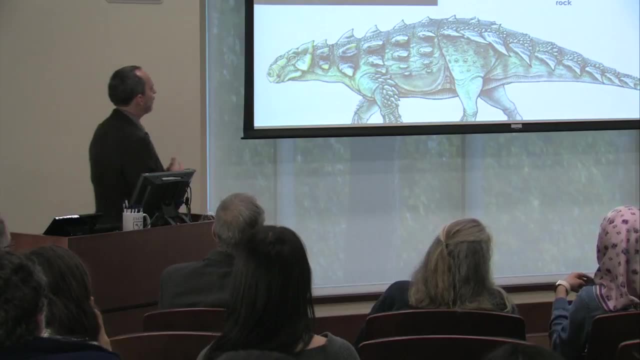 It's a counter shading. So then we were able to interpret that this was a forest-dwelling animal, that it probably lived in a shaded habitat. This is one of my favorite discoveries recently. I love ankylosaurs because think of an M1 Abrams tank. make it alive and then tick it off. These were ankylosaurs, And I love the name of this. Destroyer of Shins is the nickname that the paleontologists have given it. It was given to it because of its giant club tail there. 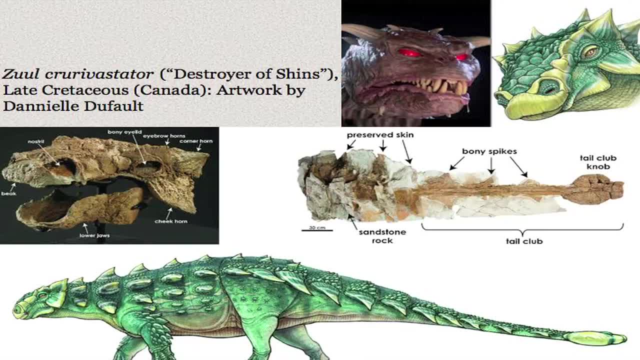 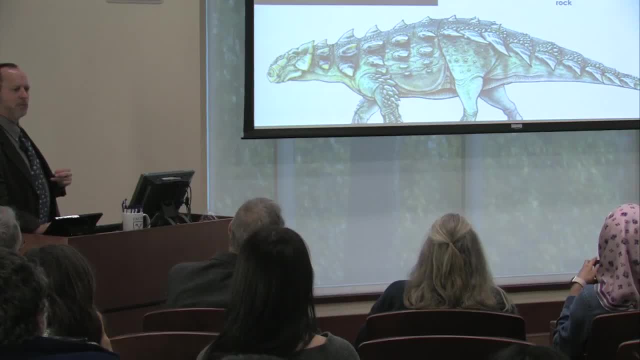 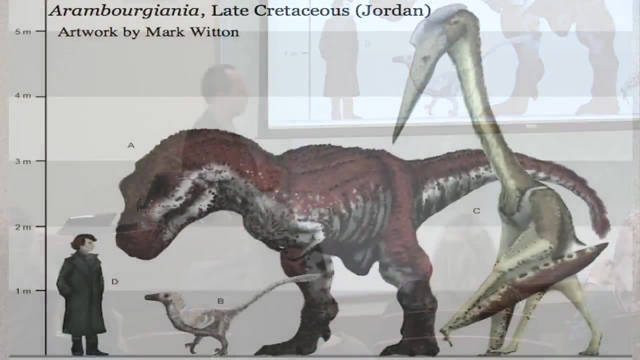 This was discovered just a couple of years ago, just was named only about three or four months ago, and it is named Zuul for the genus, because, after the original Ghostbusters movie, all hail Zuul right there. Okay, and there's our obligatory Benedict Cumberbatch. 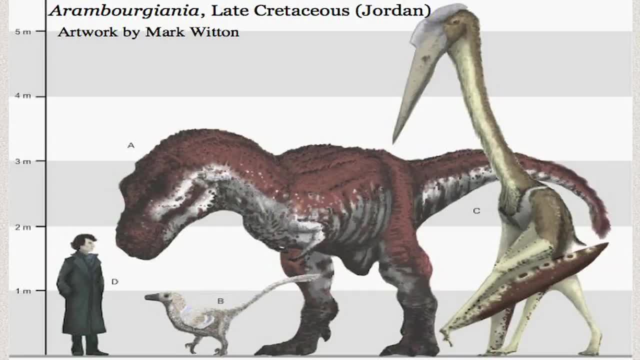 as scale slide. You probably see that in every lecture all across campus, but as a Sherlock there. so there's the Conan Doyle title. it's high in as well. This is looking at. this is a Romanian theropod- feathered theropod. 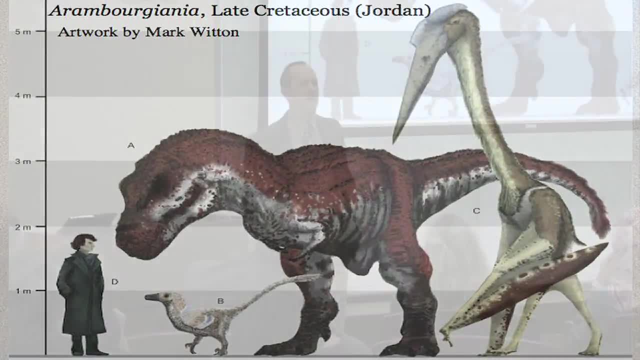 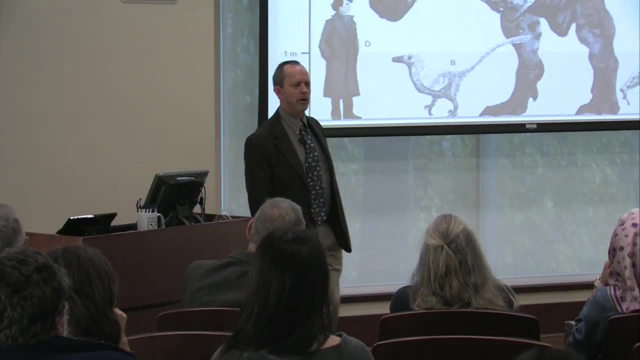 there's Tyrannosaurus rex and I want to show you how big pterosaurs got the largest flying animals that ever lived. So some of these pterosaurs we think were terrestrial stalkers, that they actually stalked their prey on land. 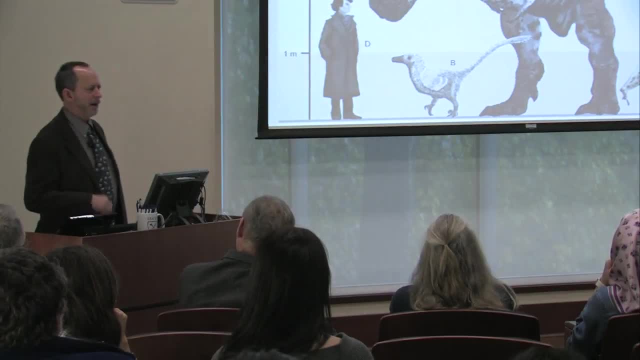 and ate whatever got in their way, rather than praying from the air. Yeah, so there are some pretty exciting things happening in paleontology now. It's something where you can check the news every week and there's always new discoveries coming out. because of this legacy, from these important books. 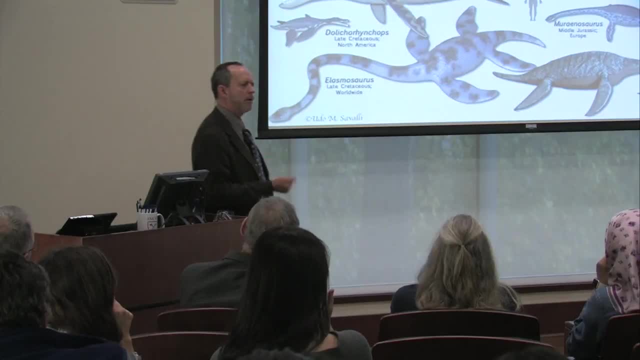 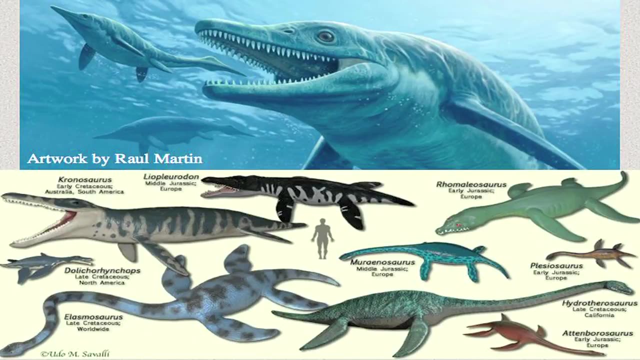 and studies before, Also with marine reptiles. we now have this huge variety of marine reptiles that we didn't know about before. Mary Anning only scratched the surface, so to speak, with those. now we know of hundreds of species of marine reptiles that also lived during that time. 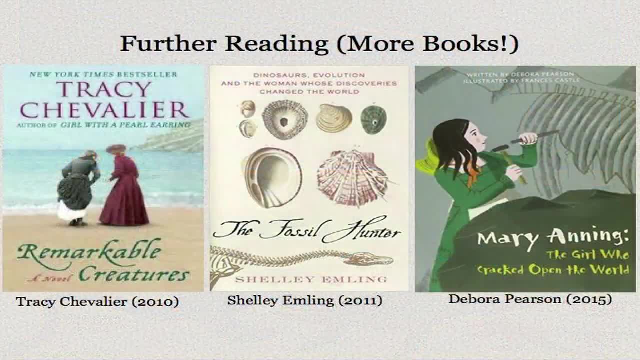 So a few more books for you, a few more things to read. If you want to read about Mary Anning, a very good novel about her, a novel about Mary Anning and her best friend at the time also has Buckland in it. 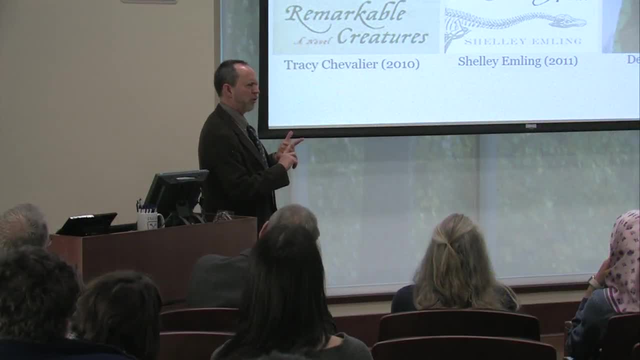 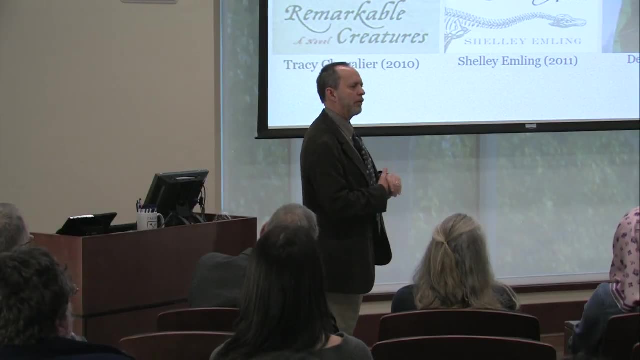 so you see a little bit of his weird personality in there, But he's a quite nice guy in the novel as he's depicted. Owen is not so nice, But there are all of these characters in the book based on real people told in novel form. 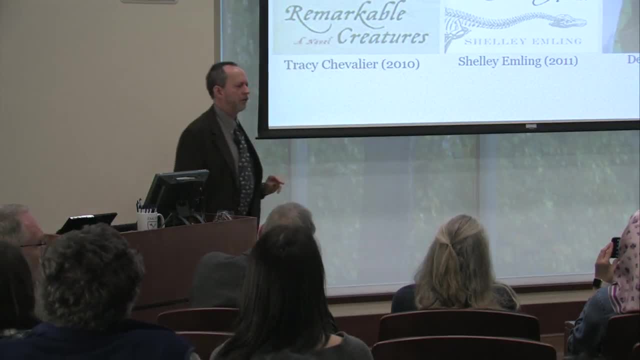 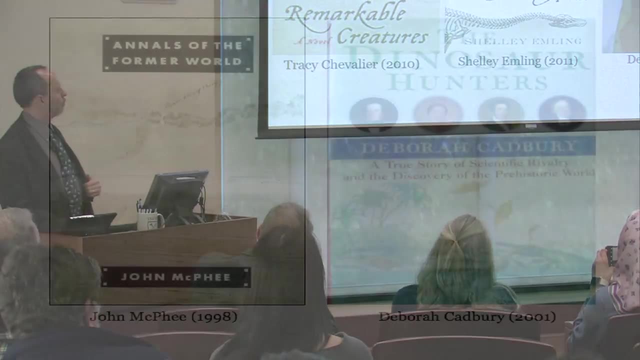 This is more of a biography about her, And then there are lots of children's books about Mary Anning. So if you have nieces, nephews, brothers or sisters who would enjoy this for a Christmas gift, good one to do Now. John McPhee I mentioned earlier. 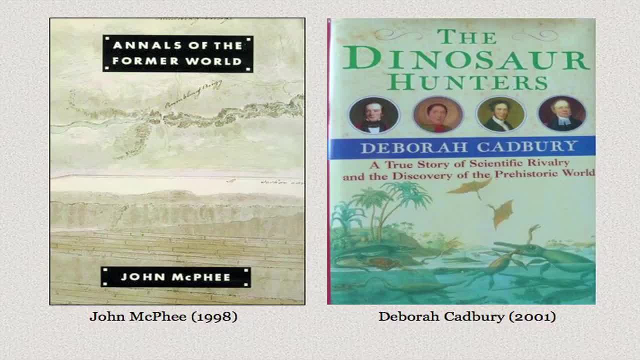 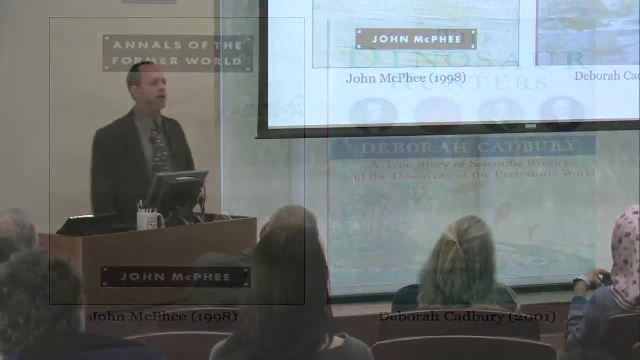 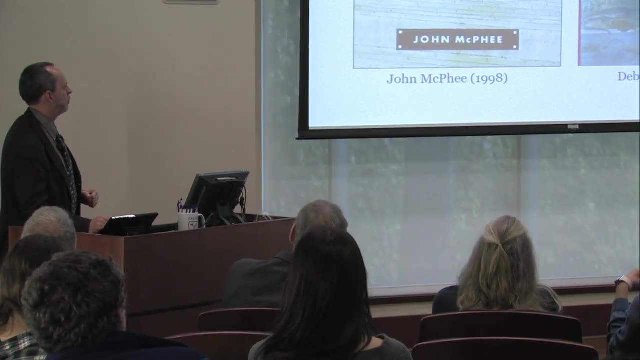 is one of the finest nonfiction writers period and he writes a lot about geology, So he's a very good person to read in terms of learning some of the basics of geology without him having to be a geologist. So he does tell it from a layperson's perspective. 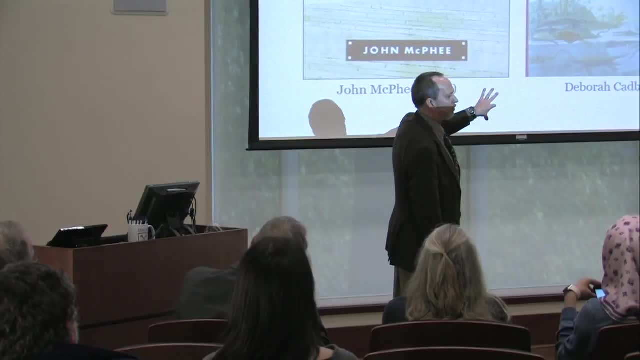 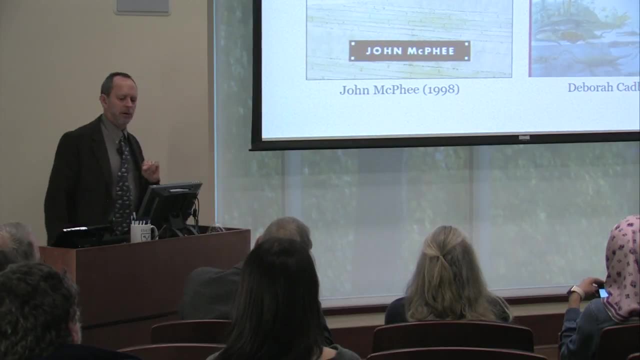 For what happened in the early 19th century in Britain and notice there's the illustration again of the ecosystem. I would read Deborah Cadbury's book. The American title is The Dinosaur Hunters. I think in the UK it's titled Terrible Lizard. 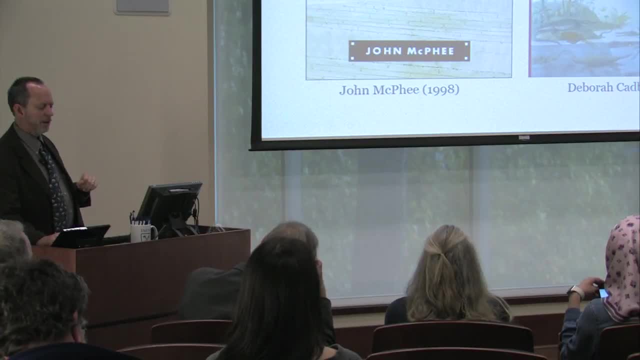 But this is about the rivalries that happened at that time and how these discoveries did get made. but there were also lots of nasty human things going on- subterfuge and those kinds of things. So there are lots of stories that are part of being human. 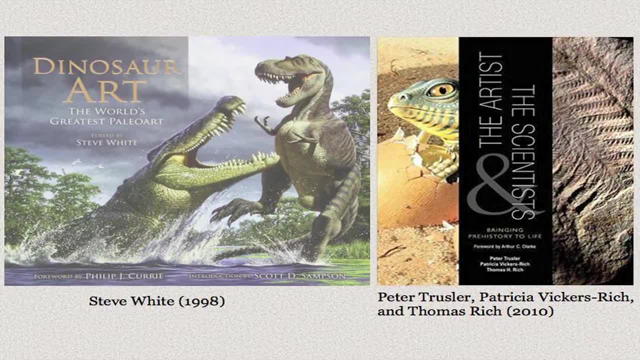 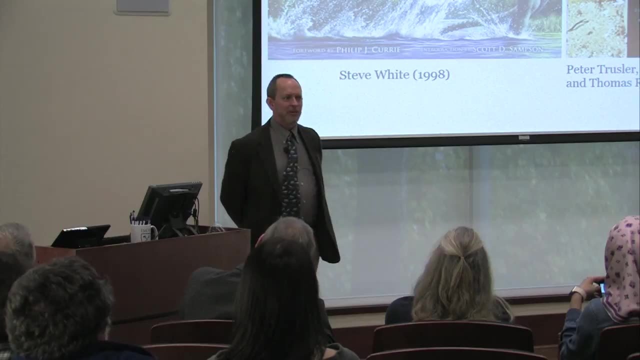 If you want art. oh my, there are so many good paleontological art books out there. This is actually painted to scale. Yes, there were crocodiles, that big Dinosuchus- yeah, The paleo art is pretty awesome when you take a look at it. 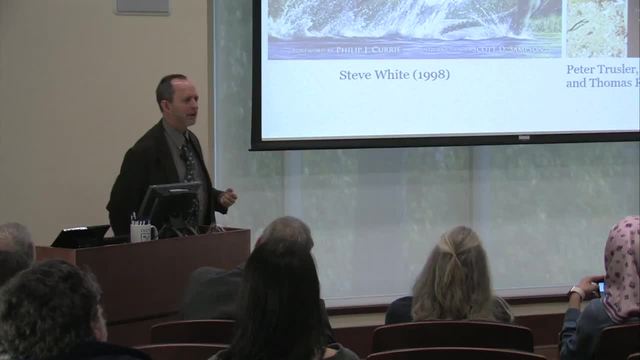 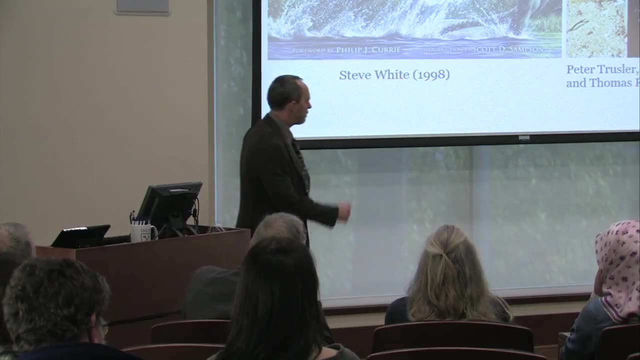 and you see these artistic recreations of these animals that actually lived. It does take you back to that time. The authors of this book? quite well, They're Australian. Peter Trusler is the artist. The scientists are a husband and wife team. 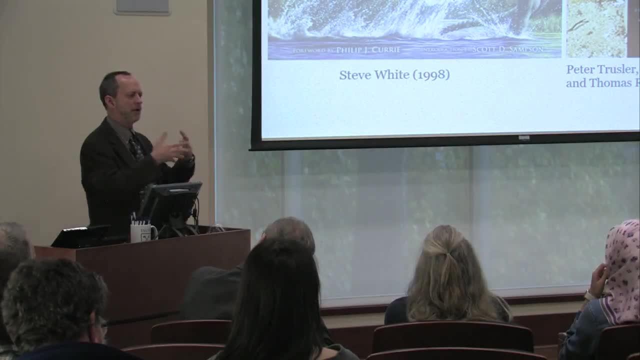 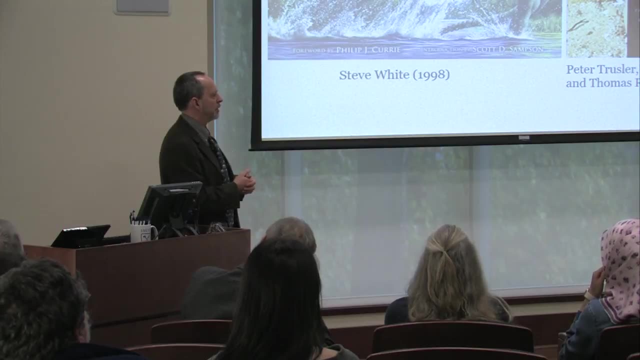 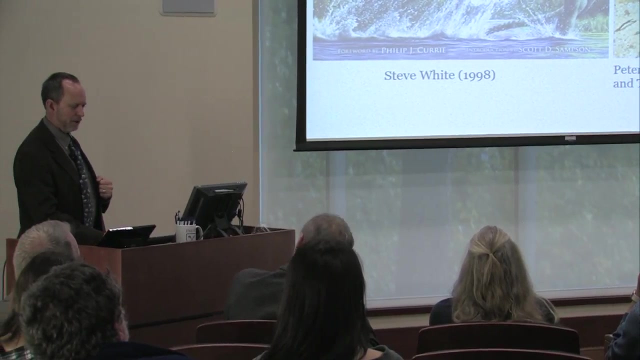 Patricia, Vickers, Rich and Tom Rich. Excellent book for looking at how art and science are not divisible, That in their case, the three of them working together over three decades, they actually were able to blend their talents and make very important scientific discoveries by putting their heads together. 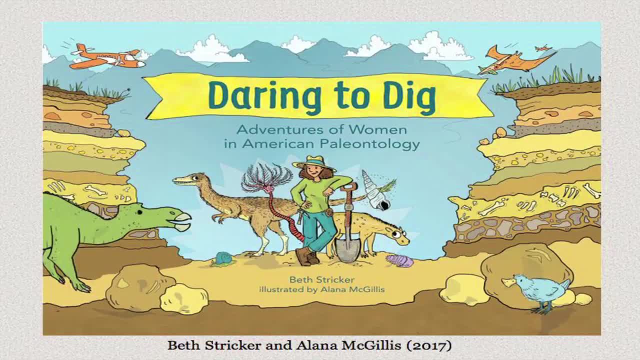 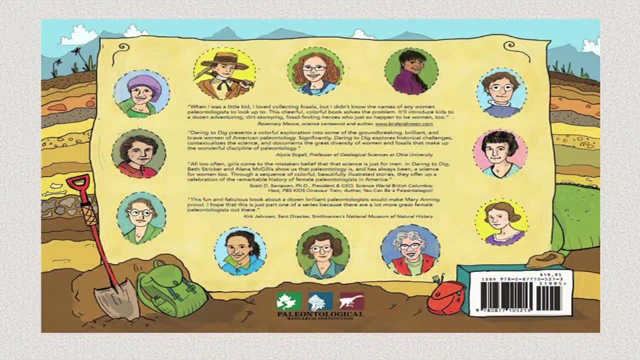 And then, if you are interested in children's books, this one just came out. And again for nieces, nephews, little sisters, little brothers, this one just came out. This is Adventures of Women in American Paleontology, And there are nice artistic depictions of 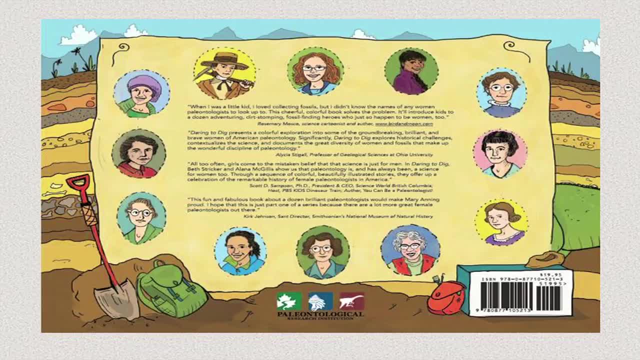 I know some of these paleontologists. Some of them are not only still alive- they'll be alive for a long time yet- But some of these American paleontologists through time, women paleontologists who have contributed to the science and are still contributing to the science. 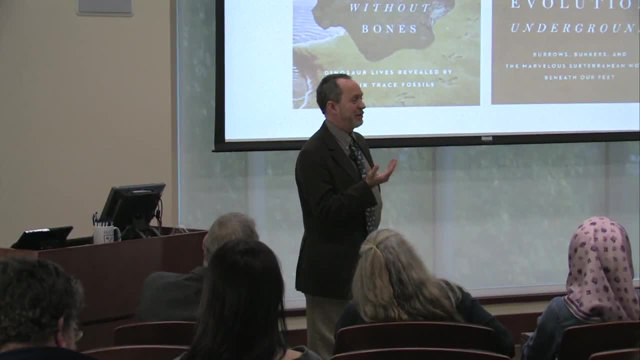 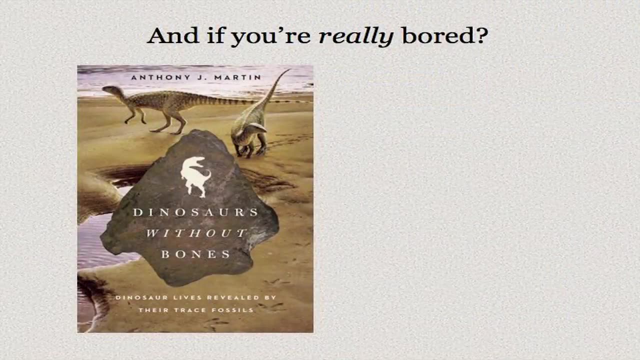 If you're really bored, you can read these books, And they do have pictures. They have photographs and illustrations done by the authors, So that's possible. And they're even in the bookstore just right downstairs in this building, by happy coincidence, And I know the author. 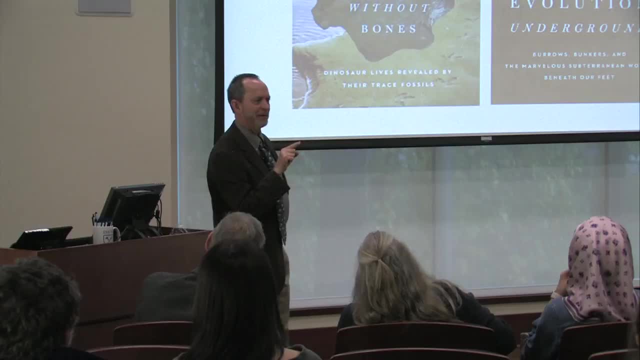 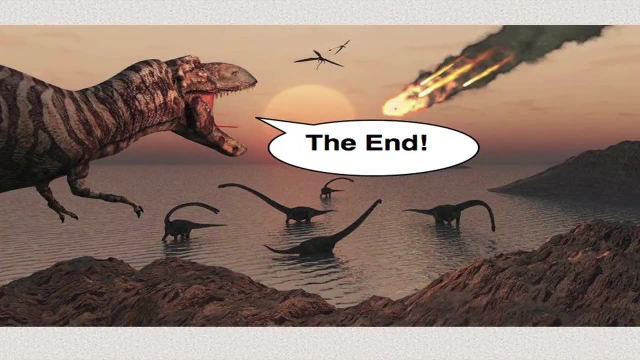 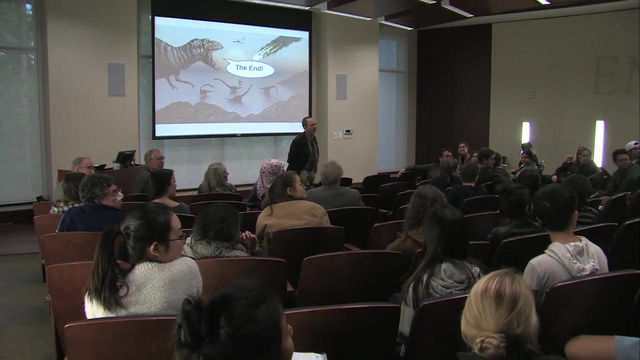 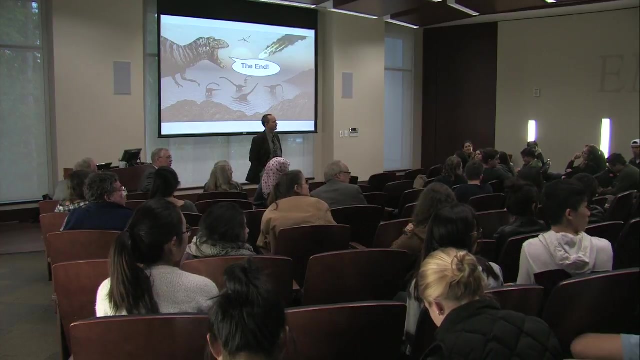 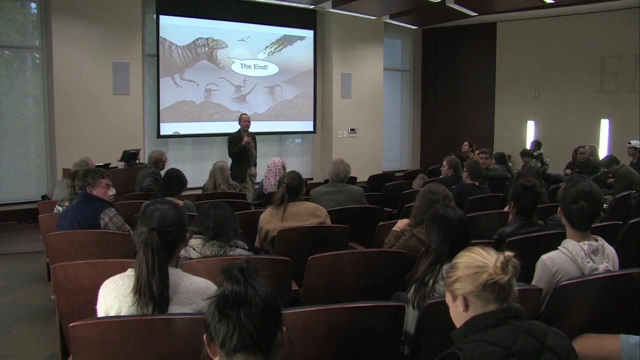 I could probably get a free autograph for you if you purchase this book or either of these books. All right, that's the end. We'll take your questions. Yes, Yes, Yeah. so that's the neat thing And I'll go back to that slide showing Adrian Mayer's book. 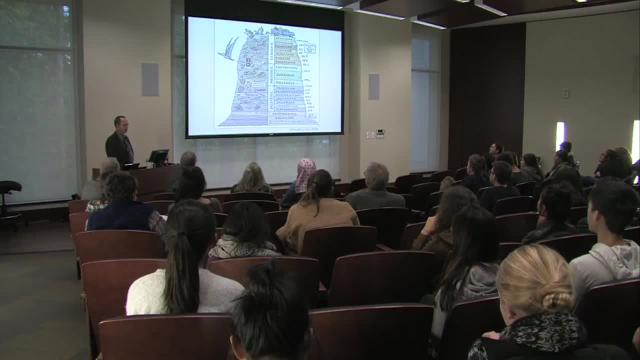 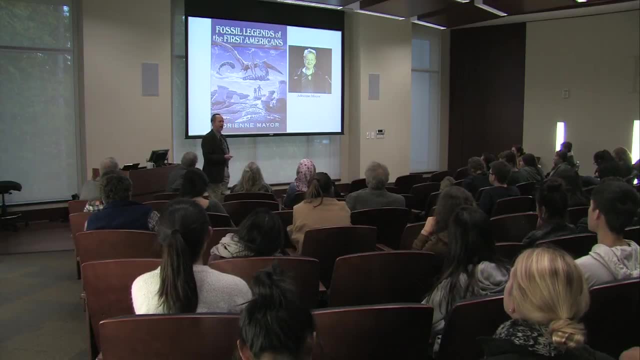 That Adrian Mayer's book. she documents it very well And she's done it in other cultures too. She did it with European cultures, the Greeks and Romans. She looked at some of the myths they had there, The myth of the cyclops, for instance. 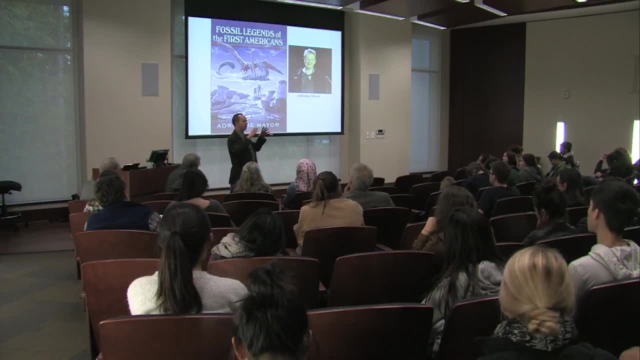 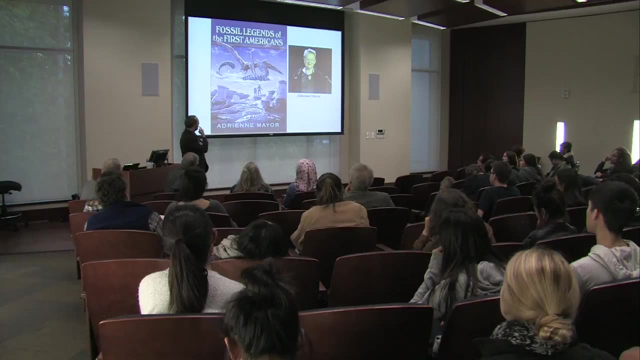 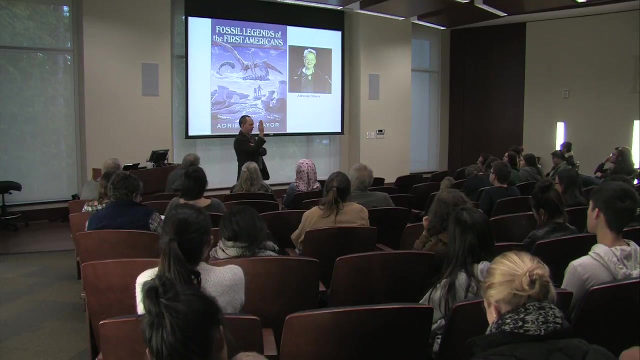 may have come out of looking at some of the fossil elephant skulls, because where the trunk was it looks like a giant eye in the middle of the forehead. And she did a few other books that also touched on this in other cultures. This one I particularly like because she looked at both the Eastern Native Americans. 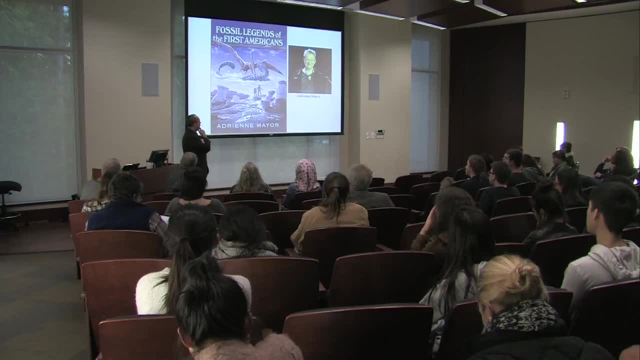 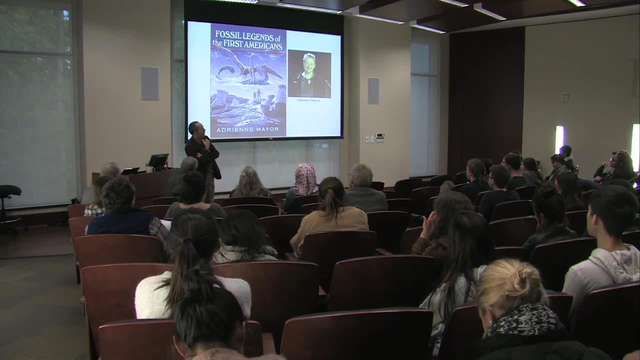 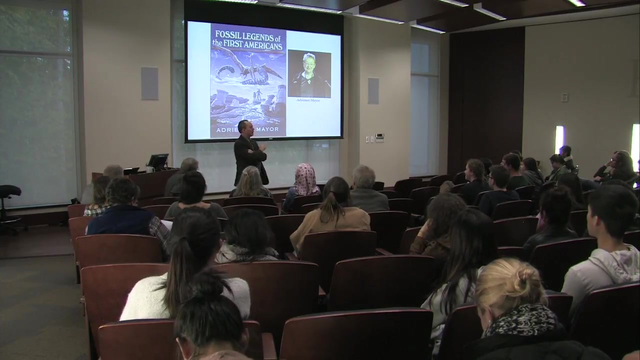 as well as the Western Native American tribes, and how some of their legends may or may not have connected to some of the fossils. So that would have been minimally. some of those legends might be as old as 10,000 years old. It looks like there's been a Native presence in North America. 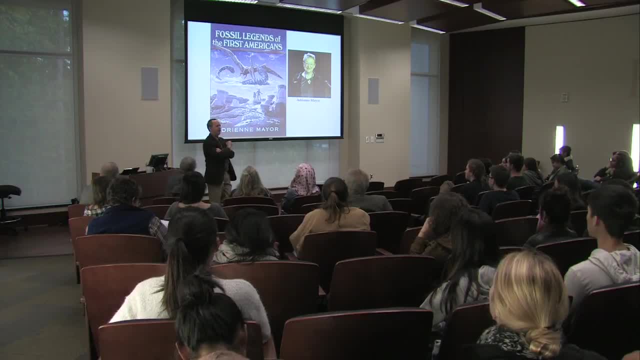 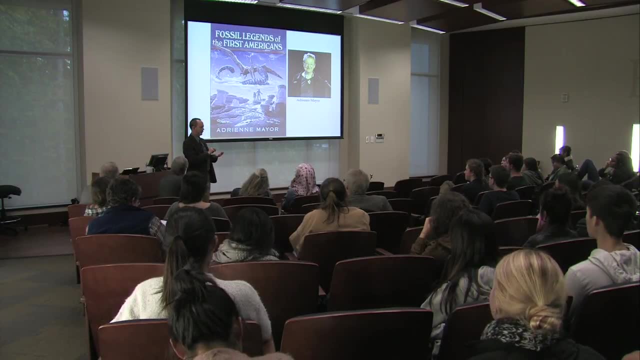 for minimally about 15,000 years now, based on the archaeological evidence. Older evidence we have is in South Africa. There are cave paintings in South Africa that are dated at about 30,000 years old that are in the same place where there are dinosaur tracks. 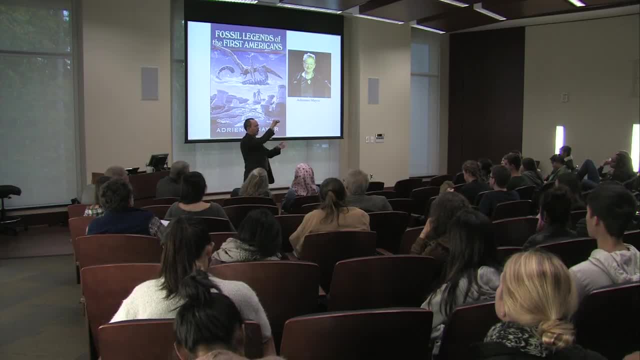 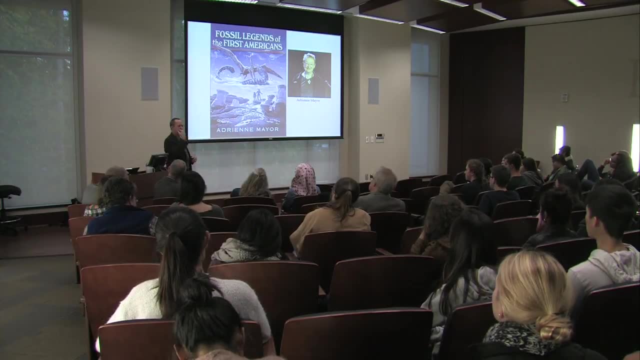 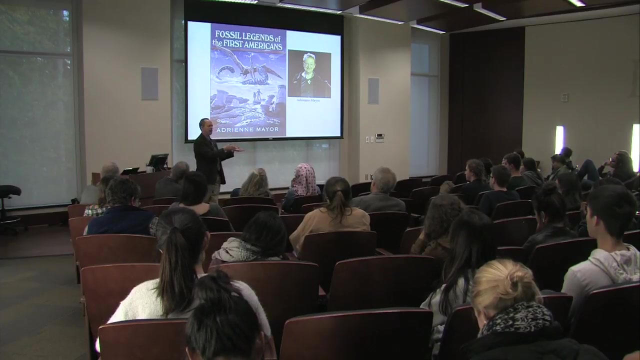 and they have these bird-like figures. they've drawn these really elongate, tall, bipedal figures that look like dinosaurs, Where some of the San tractors today are extremely good at looking at tracks and interpreting animals that this might have been something their ancestors recognized. 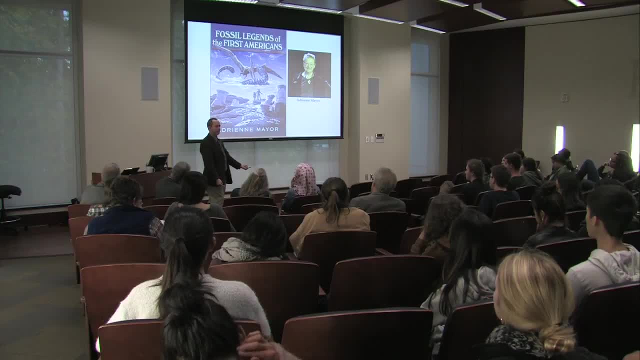 Those tracks belong to something that's like a bird-like animal. So, yeah, There's all sorts of examples of this, that well before the 19th century people were recognizing the evidence for these animals, both from tracks and other types of evidence. Yeah, good question. 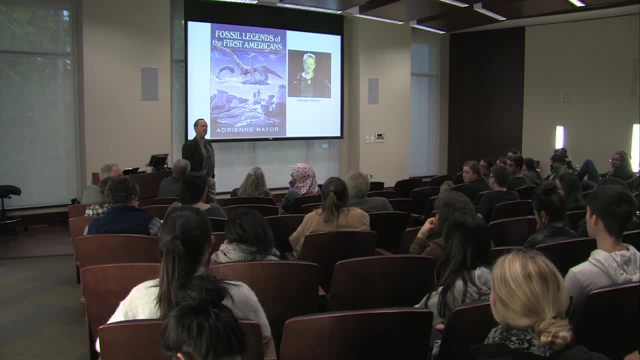 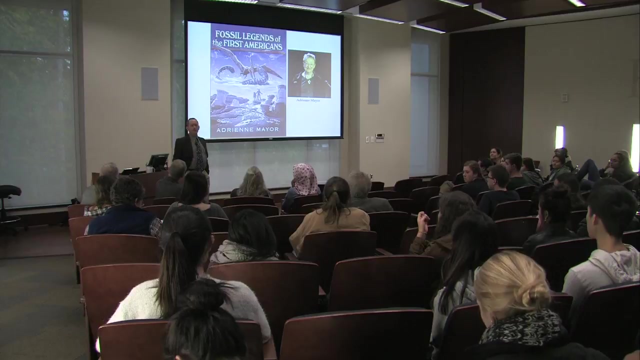 In listening to your great lecture, I couldn't help but be struck by the dominance of the Brits and the British scholars. Is that because of the empire, Or is it the religious? Yeah, that would be a great question for a historian. 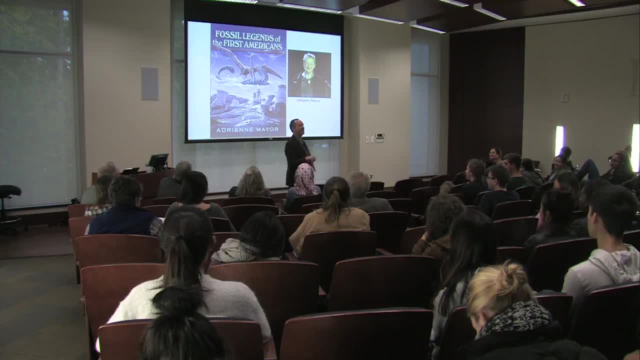 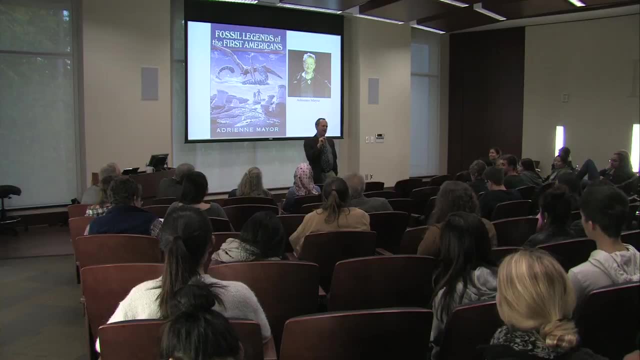 No, I'll take care of it. I'm joking, But it was partially. yeah, and I emphasize the Brits, But there were also German paleontologists There was. probably the most famous anatomist of all time was Baron Cuvier. 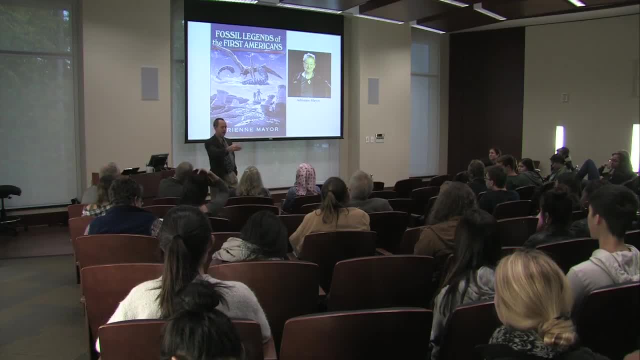 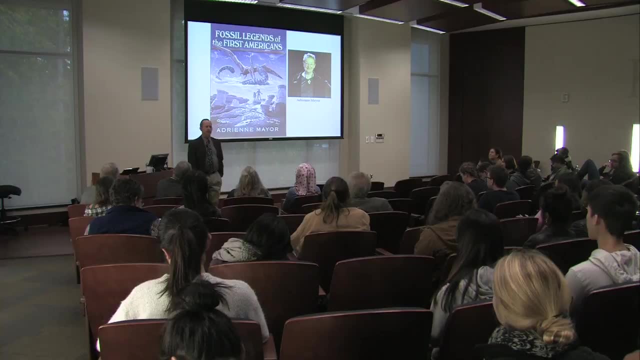 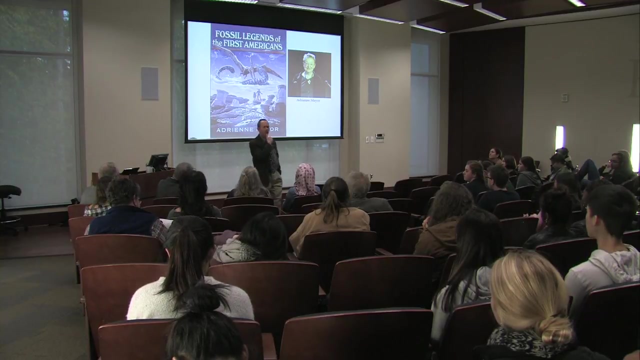 So Cuvier was the predecessor and then the contemporary of Richard Owen, for instance- and that's not so much a chagrin of Owen, because I think Owen really envied how good Cuvier was- And then it wasn't until the Americans didn't start really doing paleontology. 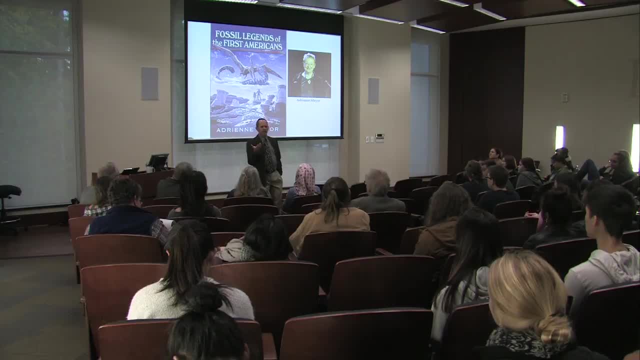 Well, I should count Thomas Jefferson. Thomas Jefferson was actually the first American paleontologist And if you go, how many of you have been to Monticello? If you walk in through the front door, there are some giant ground sloth and mammoth fossils. to the right, 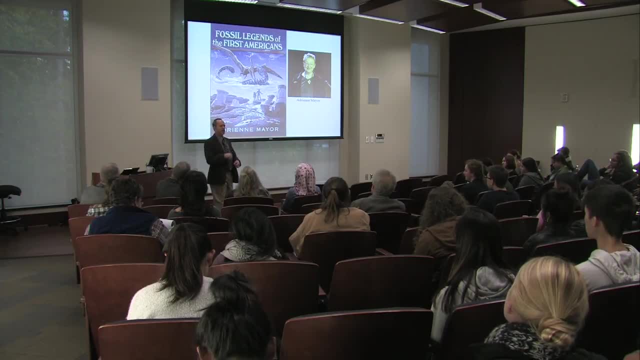 right there in the front entrance of Monticello. So he studied and actually named giant ground sloth and wanted the William Clark and what was it? the Lewis and Clark Expedition. he actually wanted them to find some of those animals out west. 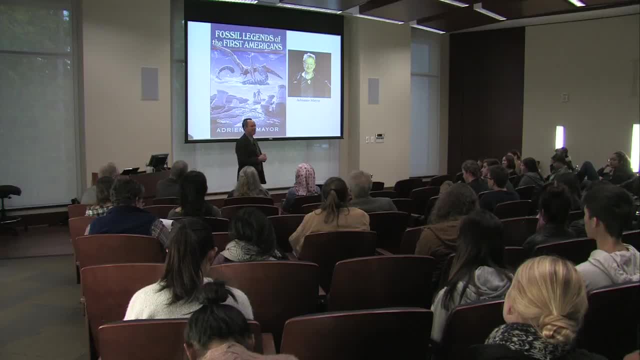 Spoiler alert: they did not find them. They had been extinct for about 10,000 years. But it was in the 1850s that some of the American paleontologists started studying dinosaurs and some of those animals, And it took off from there. 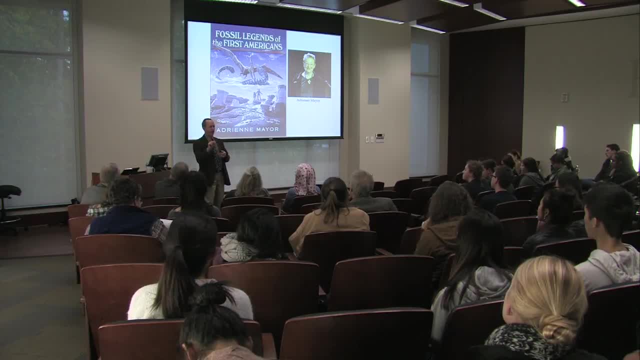 Like I said, it's in almost every country. There's paleontologists almost everywhere in the world. Just three years ago, for instance, I was in Turkey, where there were about 100 paleontologists on the field trip there, representing about 20 countries. 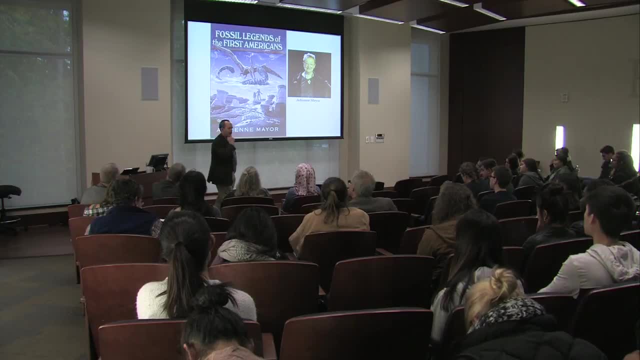 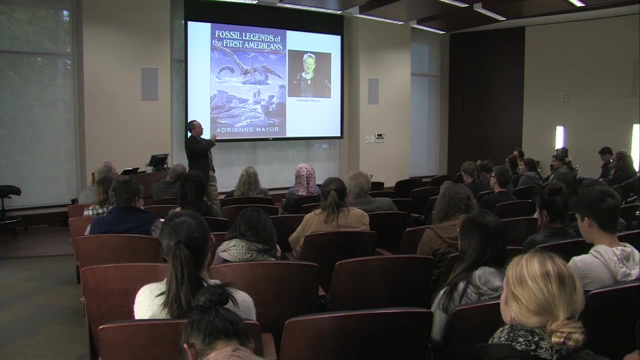 And most paleontology field trips you go on anywhere in the world, you'll get 20 or 30 countries represented in them. But yeah, it wasn't until, because what I did was it did look like the Brits were really dominating it. 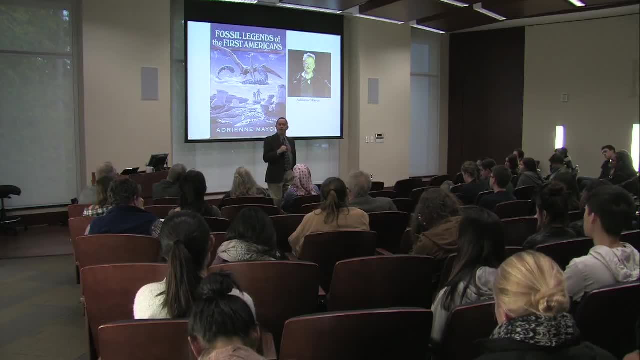 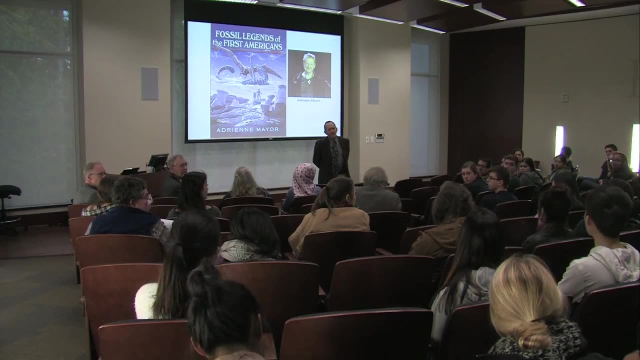 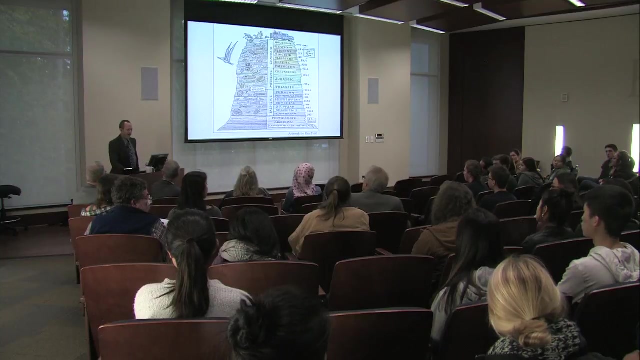 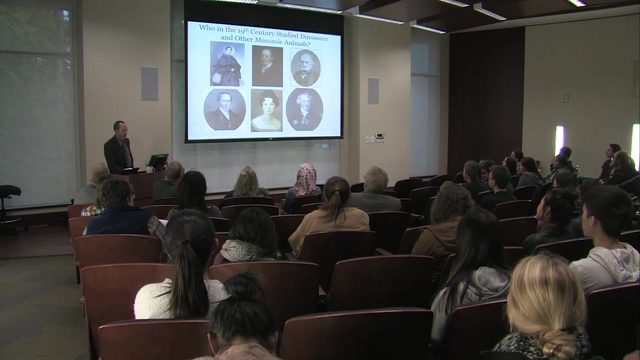 In some sense they were, but there were other people studying them too. Mm-hmm. Other questions. Yeah, Yeah, that's a great question. Let's go to that ichthyosaur. I showed a picture of it in my class: Evolution of the Earth. 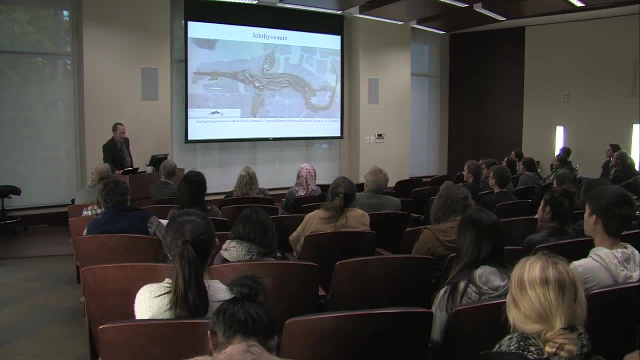 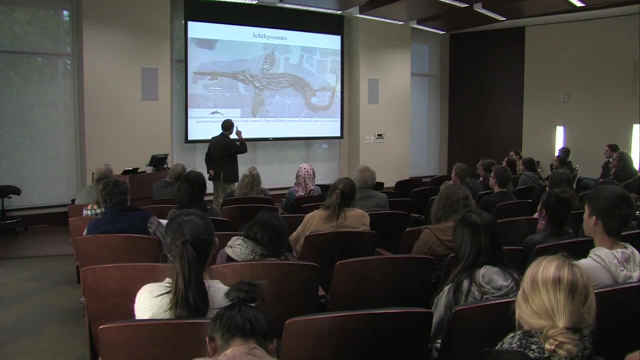 and at least one of my students is in here. There, if you go to this hall in the Natural History Museum in London, you'll see this specimen. There's this hall. it's called the Marine Reptile Hall And it goes like the hallway out there. the walls are covered with these marine reptile fossils. many of which Mary Anning found and, it says, collected by Mary Anning. There's one of them that shows an ichthyosaur baby coming out of the birth canal of the mother, And there have been dozens of specimens found since then. 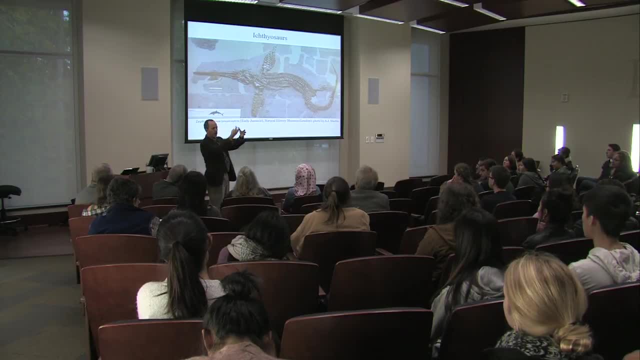 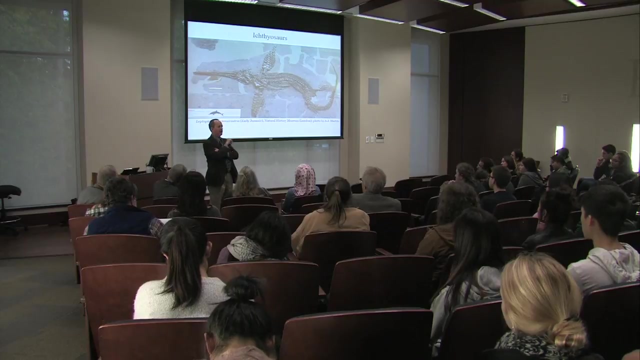 that you actually see a baby ichthyosaur coming out of the mother. In some instances they're preserved still in the mother, so they died either just before giving birth or they died while giving birth. So there was an Australian ichthyosaur just a couple of years ago reported that showed the same thing too. 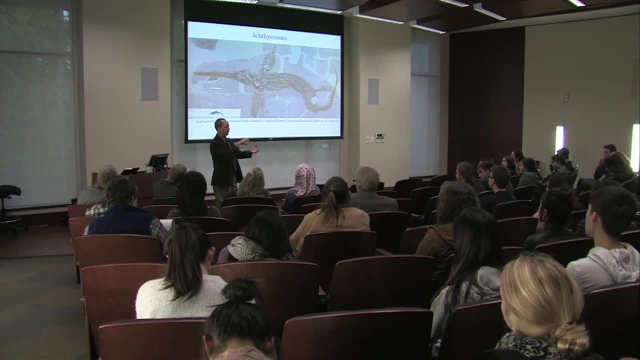 And I've seen one of the specimens that you can see, the embryonic ichthyosaur bones inside the mother. The alternative hypothesis is she ate her young. That doesn't work very well evolutionarily speaking, Mm-hmm, Not at all. 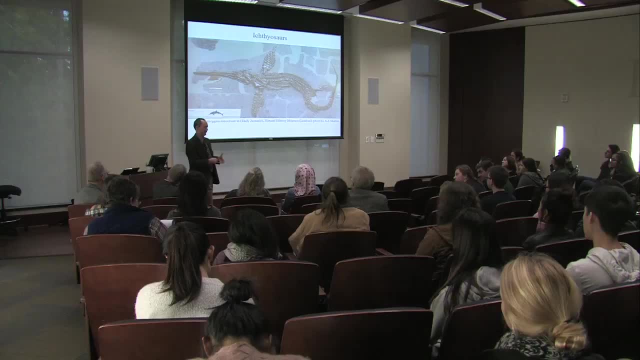 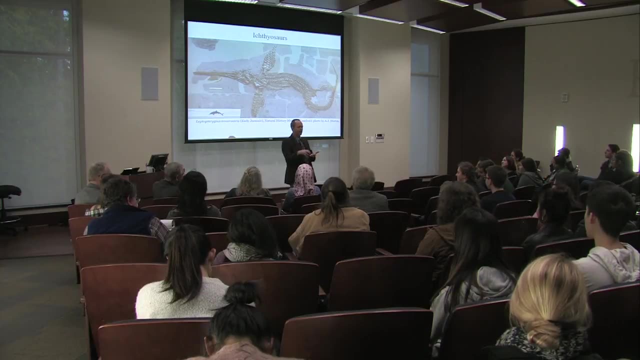 Not a good strategy. long-term Might work in a pinch, Not to give your parents any ideas, But it looks like this is really good evidence that they gave live birth. and then we have other marine reptiles since then, some plesiosaurs and mosasaurs that we also think gave live birth. Makes sense because if you're an eight to ten ton animal, going up on shore to lay your eggs like a sea turtle might not work all that well. So giving live birth is an evolutionarily sound strategy that gets selected for over time. 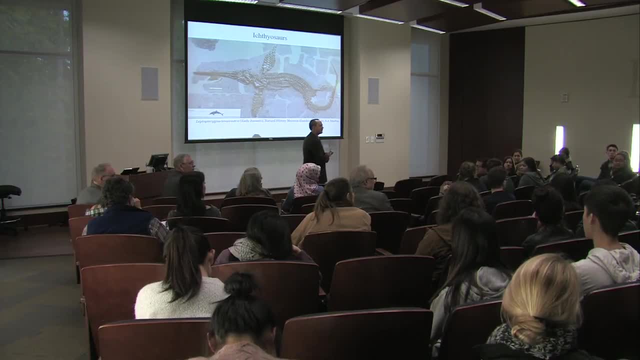 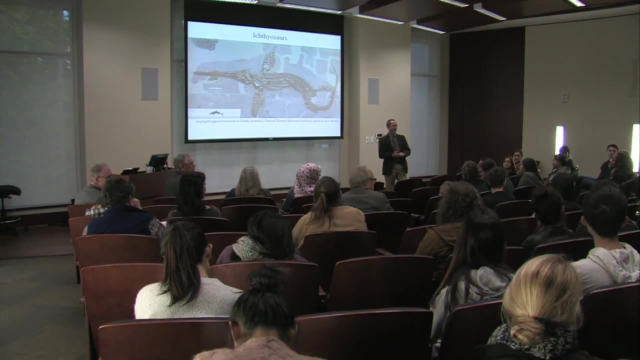 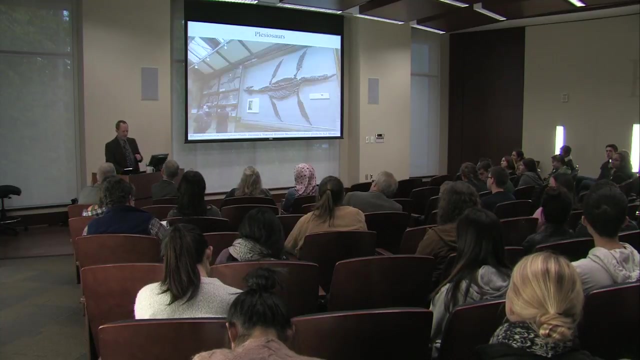 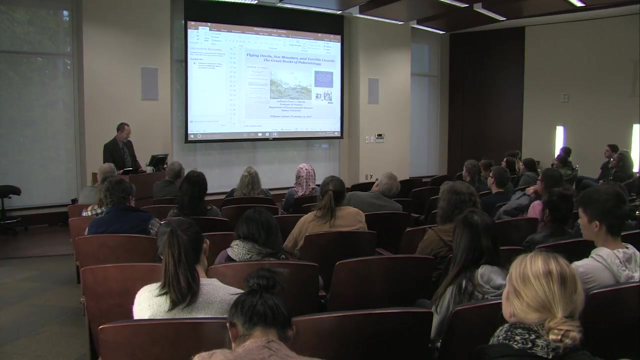 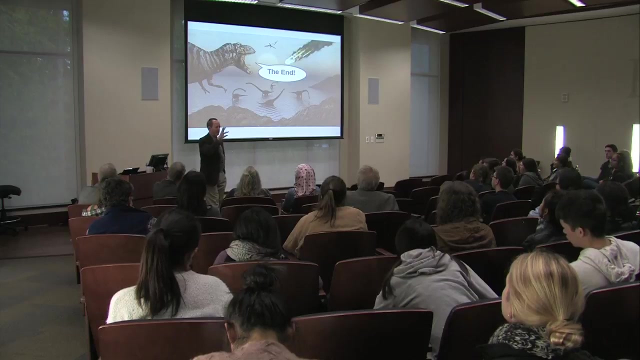 Yeah, really good question. Uh-huh, Yeah. Yeah, My very last slide, actually sorry for the whiplash. Okay, The very last slide actually touches on that And I was talking about that. By lucky coincidence, in my class today I focused on the end. Cretaceous extinction. 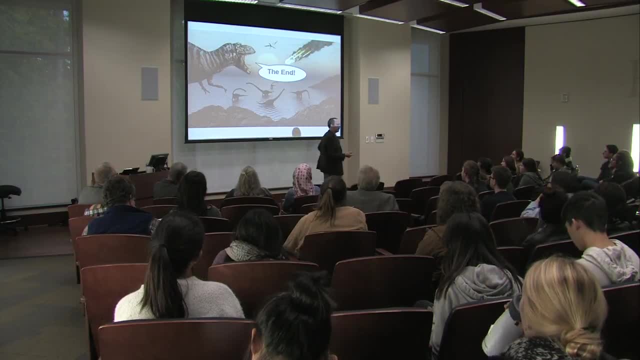 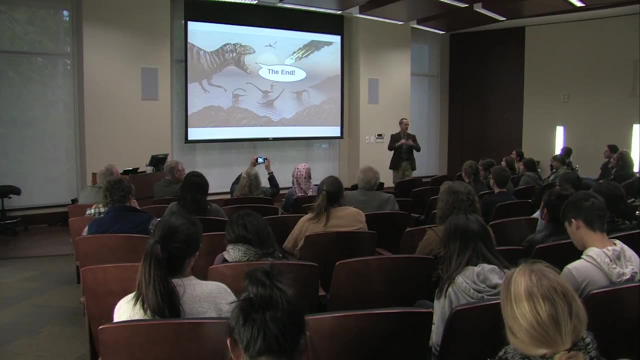 There were several factors happening. There was volcanism happening where India was its own subcontinent and it was drifting north, and there was all this volcanism, the flood basalts of the Deccan Plateau there. That was going on for millions of years. 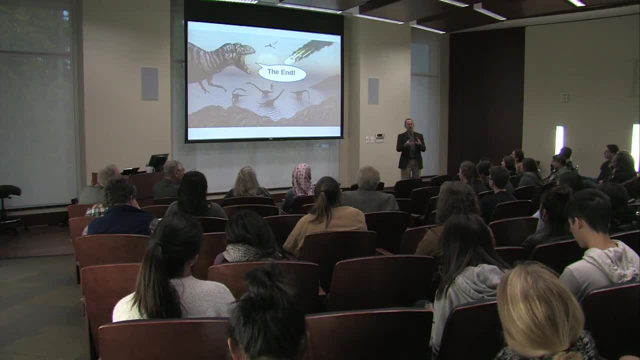 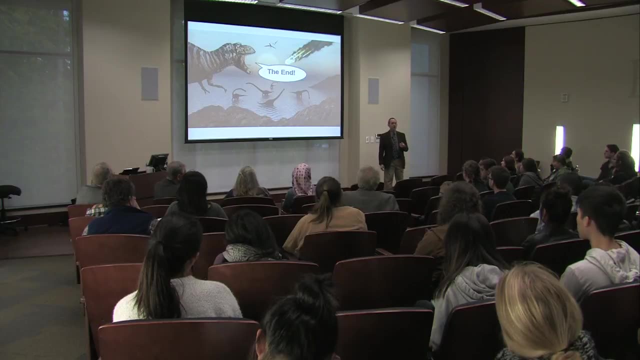 That was changing climate at the time, So that was causing some ecosystem stress at the time. And then a 10 kilometer wide meteorite hit the Earth And that was really bad And I was talking about that in my class this morning. 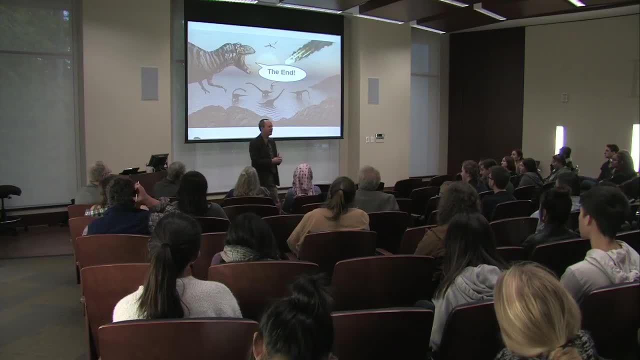 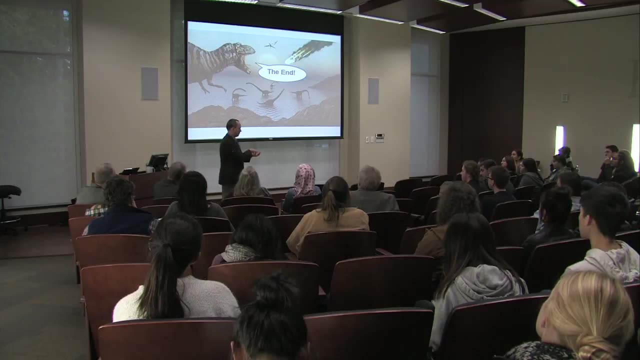 calculated as the equivalent about 300 million nuclear bombs going off at the same time in one place. It hit rocks of the right composition. right composition that it put sulfur aerosols and soot up in the atmosphere. So it actually caused global cooling below freezing for three to five years afterwards. So anything that was big died because photosynthesis shut down. So there's the base of the ecosystem, both the oceans and on the land. You don't have photosynthesis, You don't have plants for the herbivores, The big herbivores die. 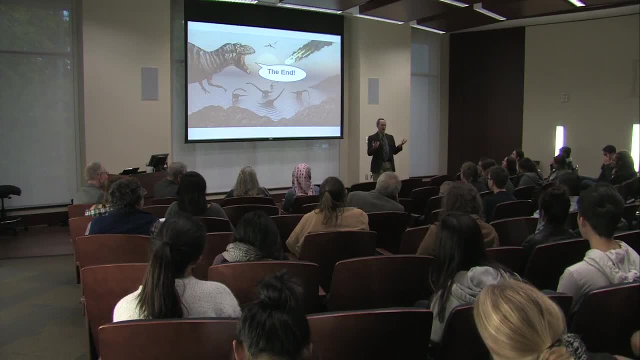 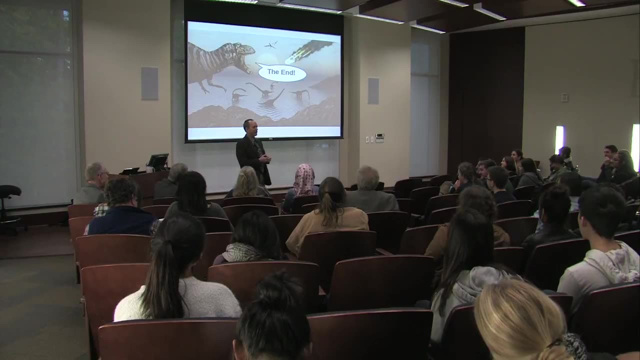 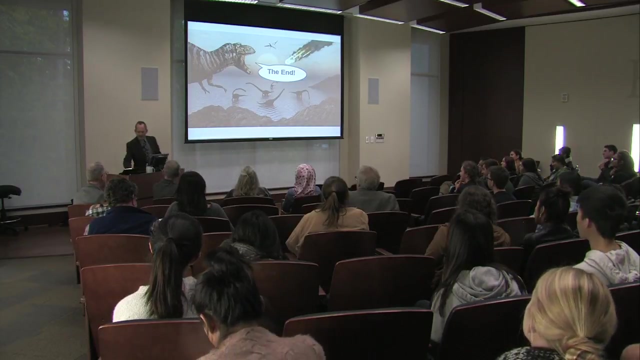 The scavengers are loving it. for a while The scavengers are going: yeah, more dead meat yum. But eventually that runs out And then you're dead. So anything big died, Small animals survived And I like- and this is actually in that book on the right by some guy I know- 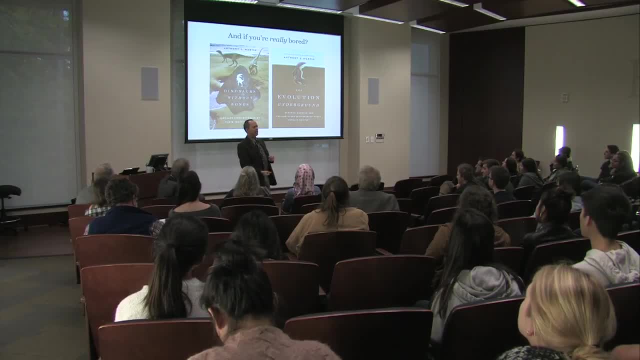 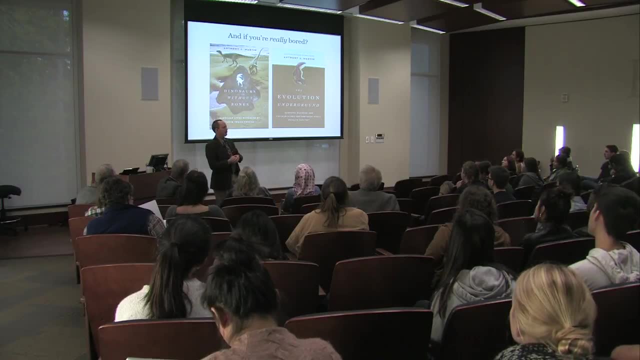 That book. that was one of the themes I had in the book is that mass extinctions through time, especially this one with a meteorite. if you were a small burrowing animal you had a major advantage making it past the extinction. And I like to say we're here talking about it now because of that. 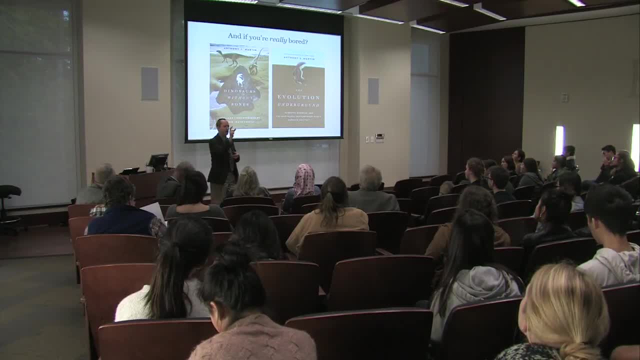 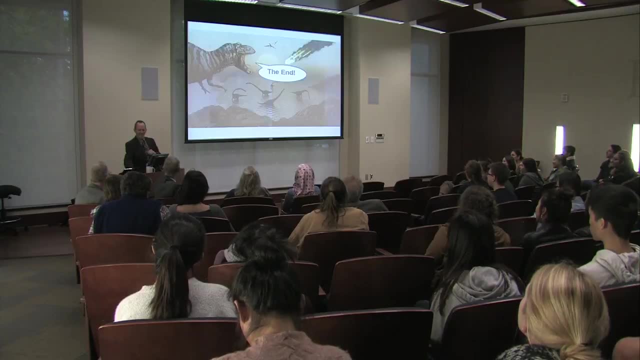 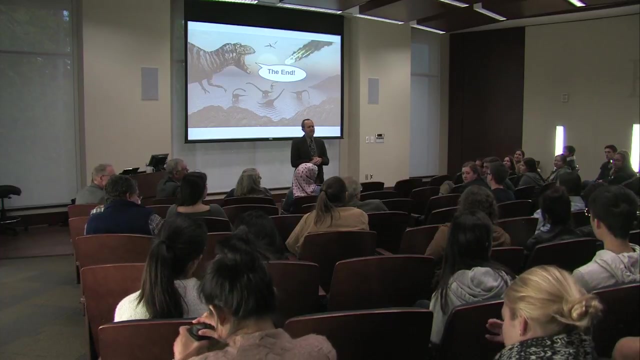 Because our mammal ancestors were little and they were in burrows. That's why, every day, I am thankful for them and their burrows. Okay, good question. Others, Any others? Yes, How did site excavation when, during the beginning of formation? 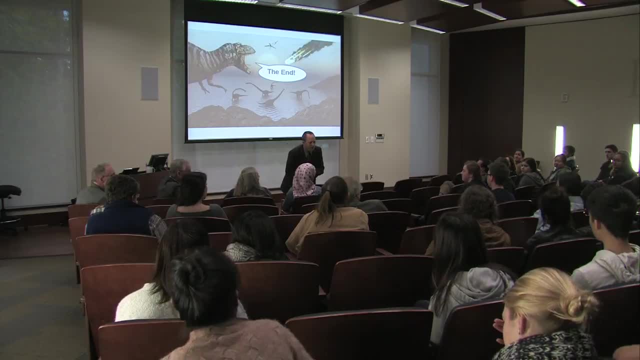 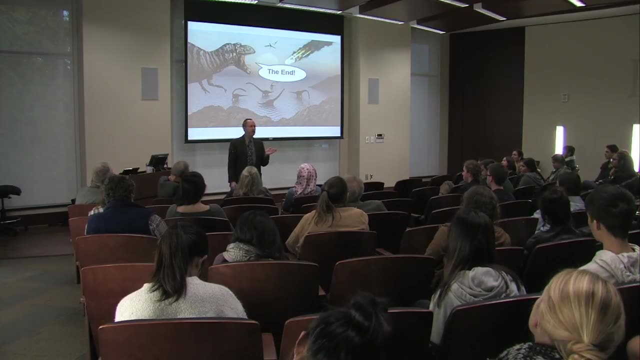 compared to what it is now. Say again the first part: How did site excavation Site excavation? It's still very much the same. Yeah, this is neat, Some of the dig sites I've gone to over the years. you look at photographs from the late 19th century. 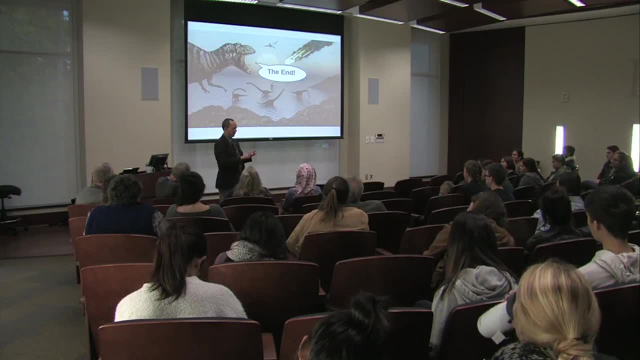 especially in the American West, when there were two paleontologists, rival paleontologists Cope and Marsh. They were going into the American West during the Western expansion. They were hunting for dinosaurs out there. You look at their dig sites and they were doing almost the same things as today. 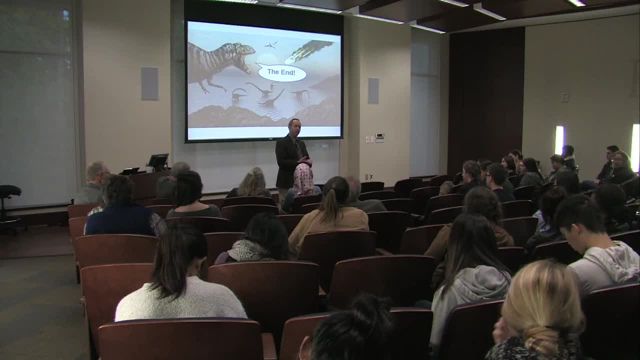 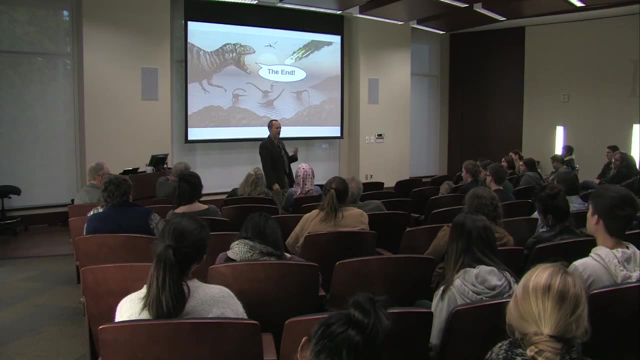 So a lot of the same brute labor, brute force- going out there and digging and using pickets, and now we have jackhammers and other pneumatic tools that we use to break up some of the rock. But a lot of the techniques are still the same. 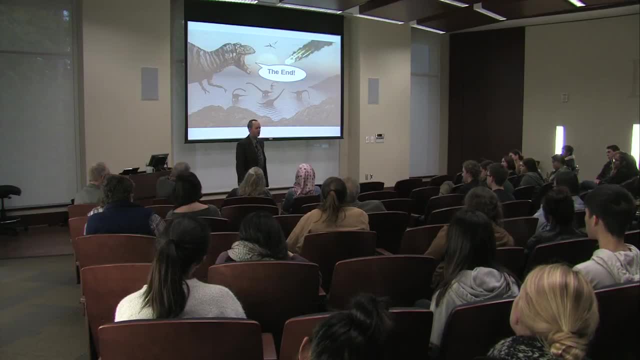 There's a few upgrades, but not many. It still requires a lot of physical labor for those sites. Yeah, Does that answer your question? Mm-hmm. Good, We have time. We need to stop now, but please join me in thanking Dr Martin. 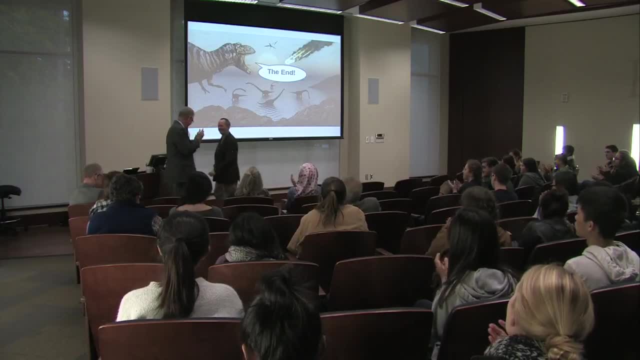 Thank you very much, Thank you.